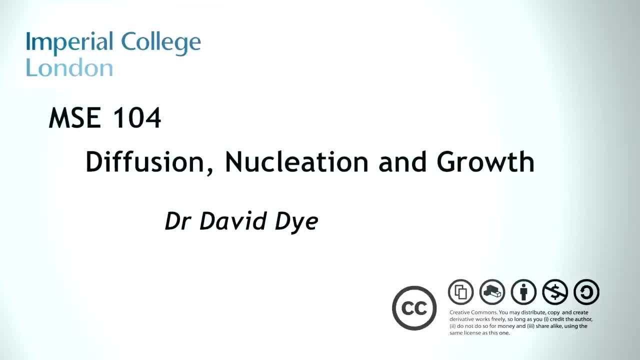 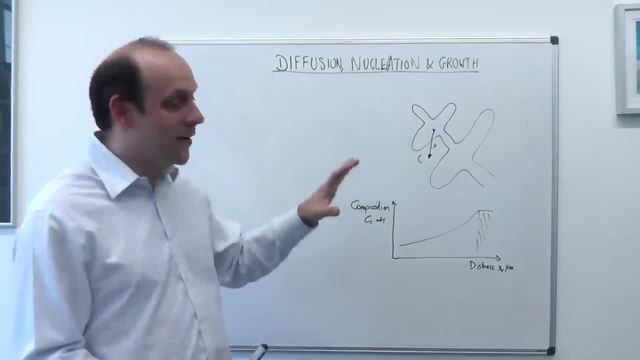 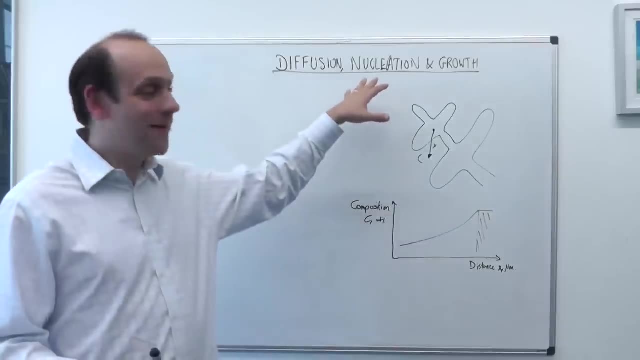 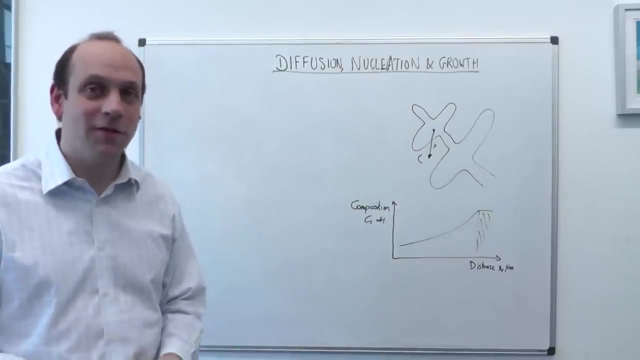 Okay, so this piece is about diffusion, nucleation and growth. So we're going to start out thinking about diffusion and then how we form microstructures, how they nucleate, how they begin and how they then grow. So previously we looked at the Scheil solution for solidification in 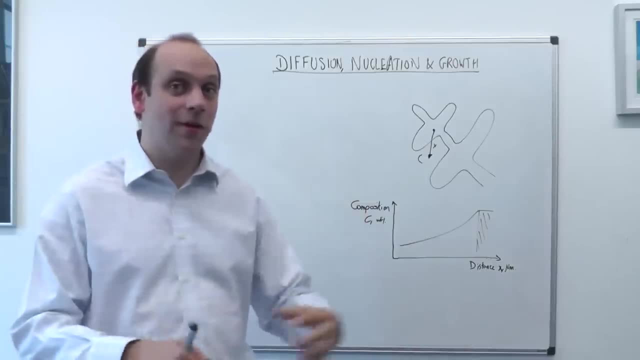 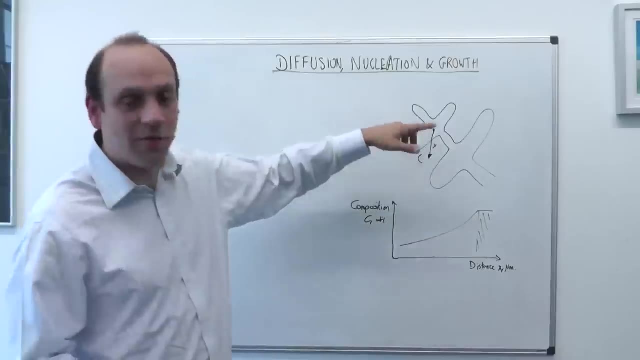 the case where there isn't time for diffusion to happen in the solid, And we said that we typically grow things as dendrites. We found that in the labs And if we plotted the composition from the first solid to form to the last solid to form, we said we'd have a curve that looked 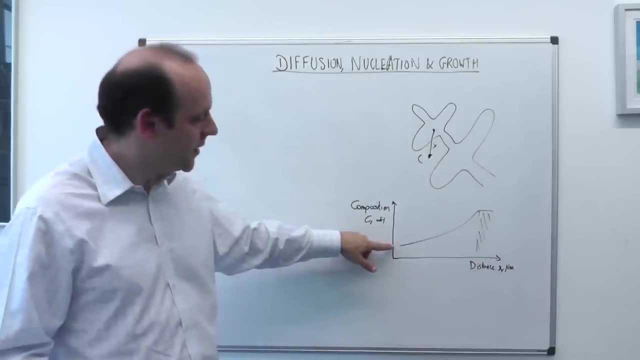 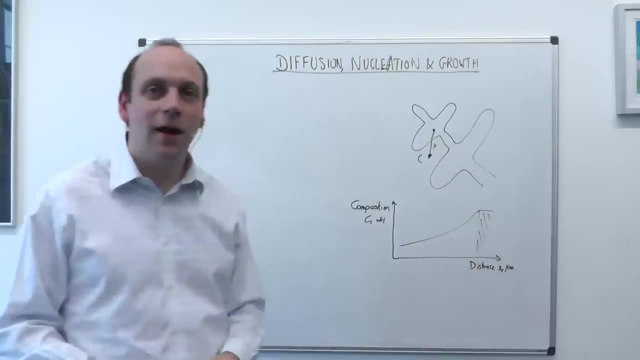 like this. So it would start off quite low, quite pure. solid would form first, And then that composition would come up according to the Scheil equation, until we got to the eutectic composition and then the last material formed as eutectic. 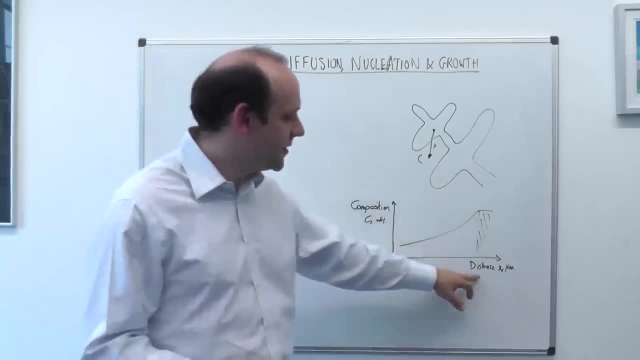 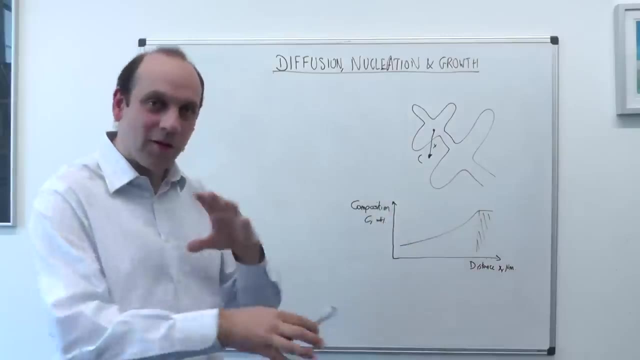 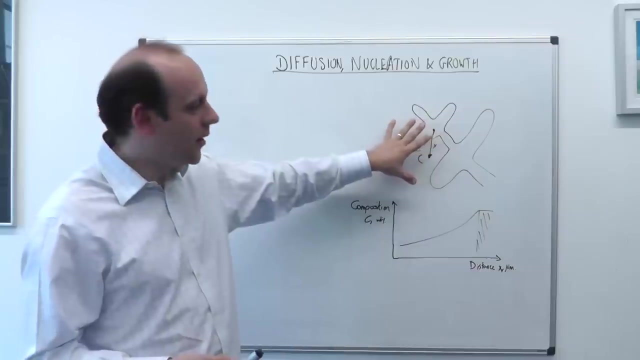 And so we'd have a graph of composition versus distance, which a distance would roughly be something related to volume fraction, although it's difficult with the areas and volumes and so on. So then we said that we would want to homogenize this composition by heat treating. 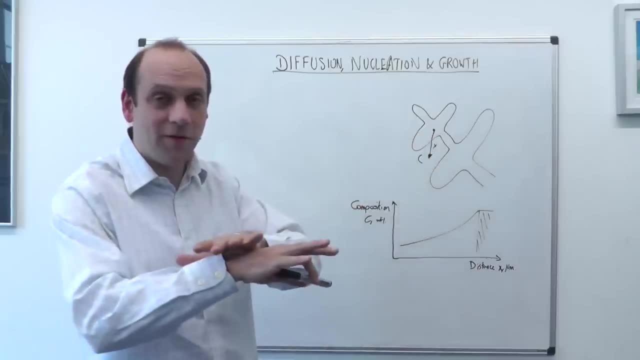 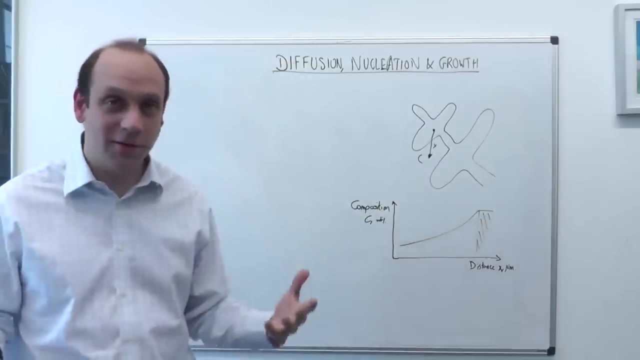 it so that all of the atoms could interdiffuse and level out this composition profile to the alloy composition. And this happens by a process called diffusion, Which you'll study more in 102, but this is the, if you like, the brief introduction. 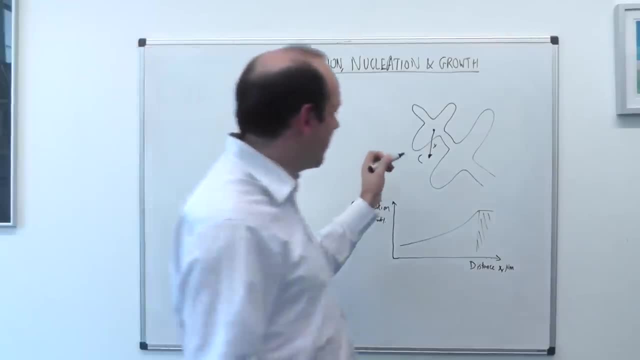 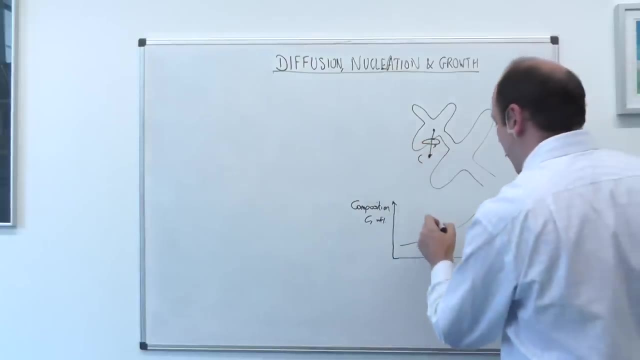 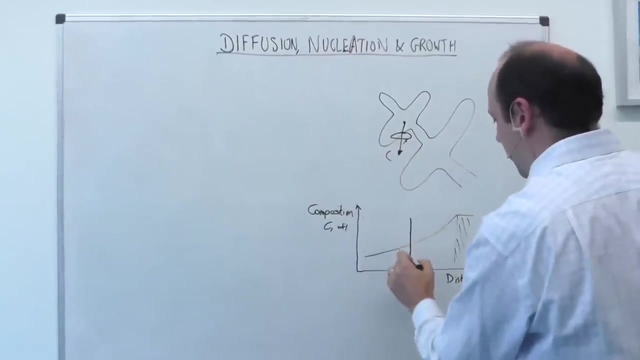 to why that occurs. So we consider here, if we take an area, a control area here, sort of projected into the page, and we ask what the flux is, the movement of atoms is through that area, say that's at that position in distance. So we imagine we've got a control. 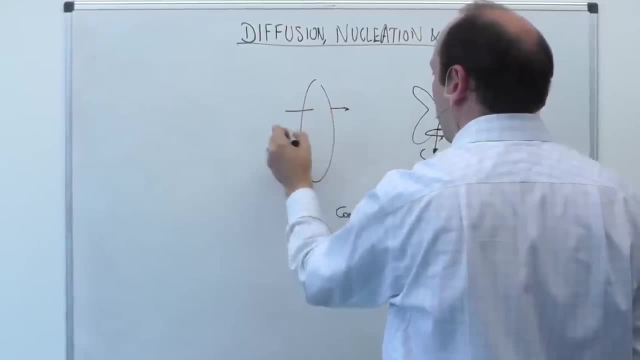 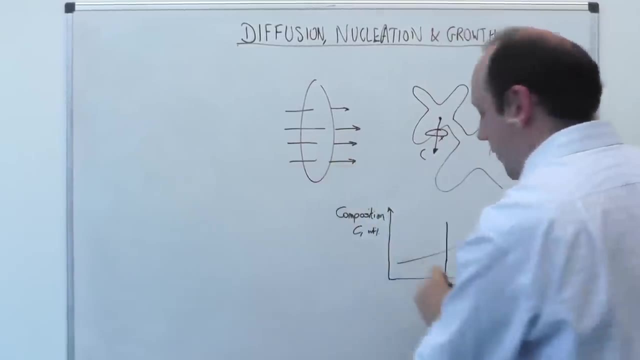 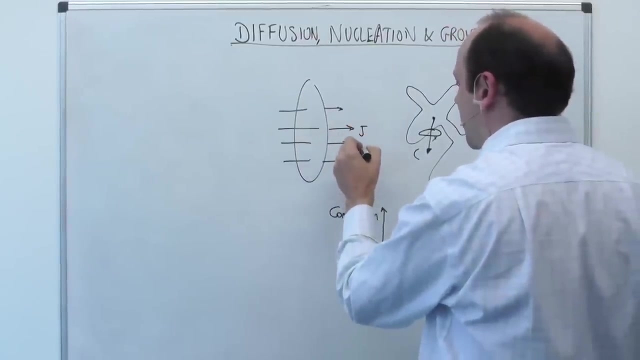 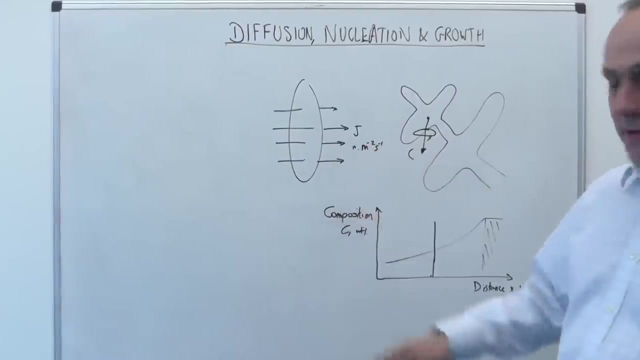 area and a flux of atoms going, if you like, through That area, Then in the middle of this composition profile. that amount we call J, So that's a number of atoms in N, say, per meter squared per second, And that's called a flux, The 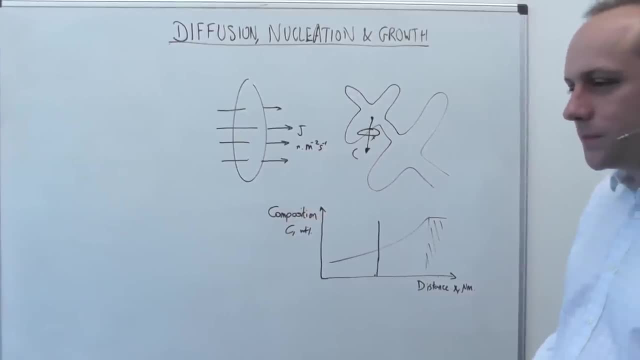 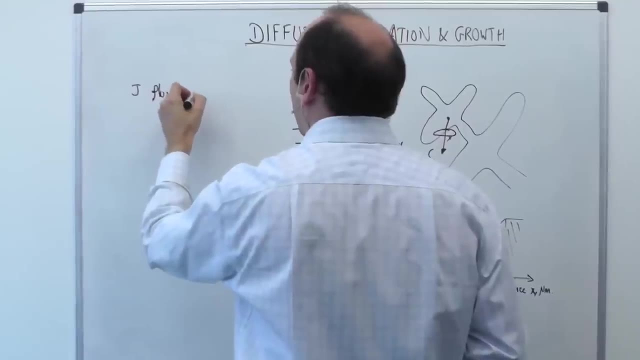 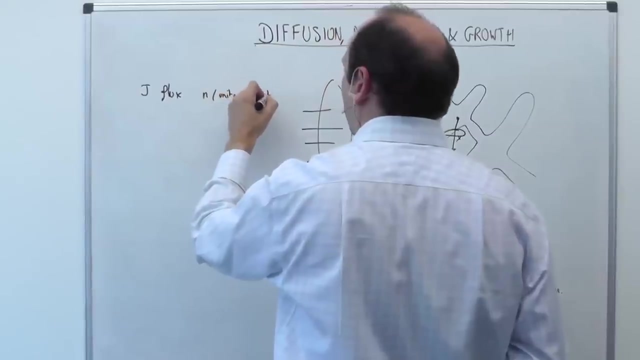 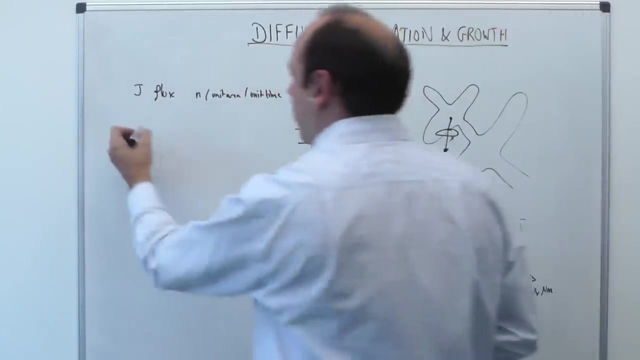 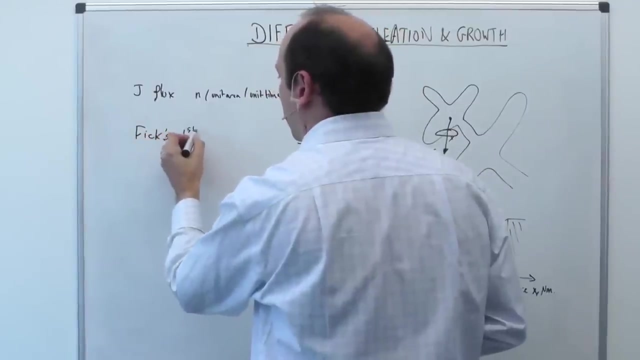 number of atoms going through this control area. So J, here is a flux And it's in, It's in numbers of atoms per unit area, per unit time, And Fick's first law is the following: So this is Mr Fick, And his first law says that: 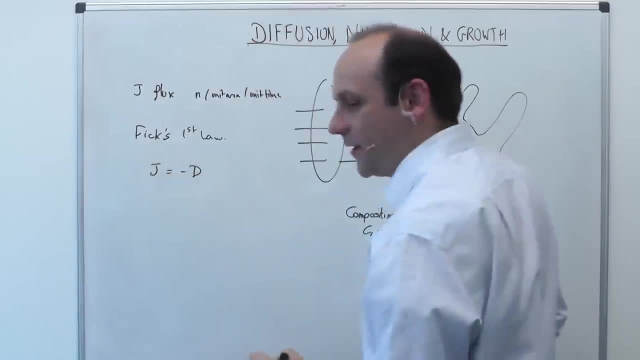 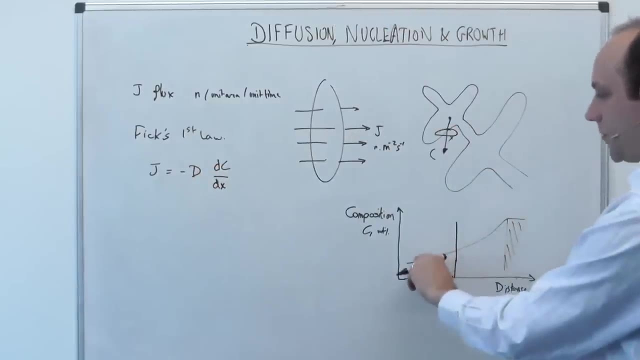 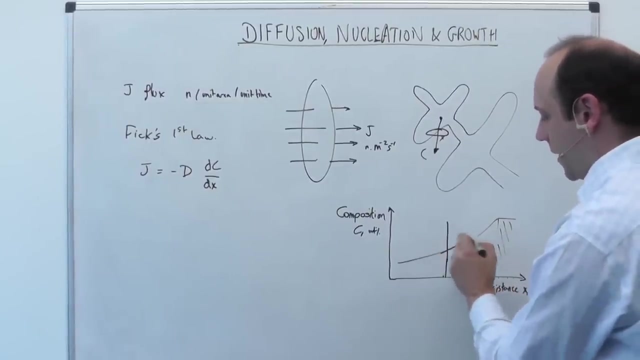 the flux is equal to minus a diffusivity times The concentration gradient. Atoms flow down a concentration gradient, So here the concentration gradient is positive. As we've drawn it here, the atoms would move to equalize that, So they would move that way. 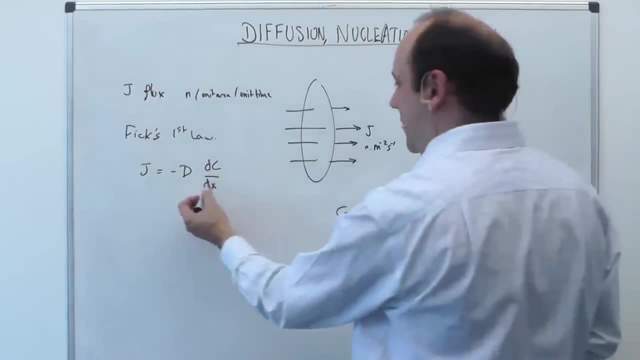 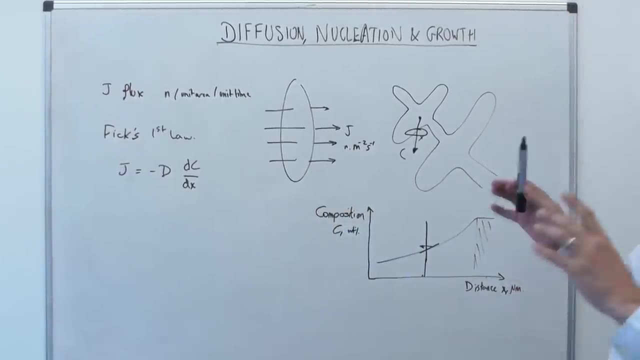 So they'd move opposite to the concentration gradient. So this dC, dx, that's how steep that is, And the steeper it is, the faster atoms would go. And that's a phenomenological law, so-called, So it's one that's true by 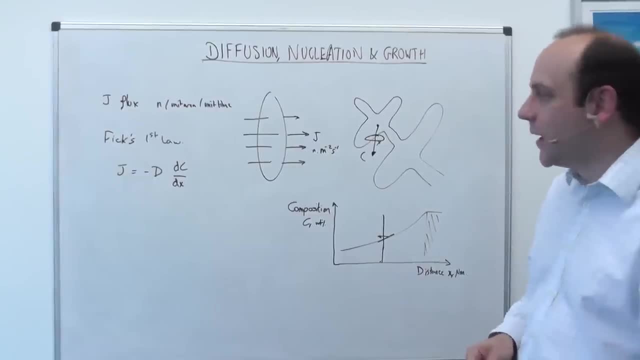 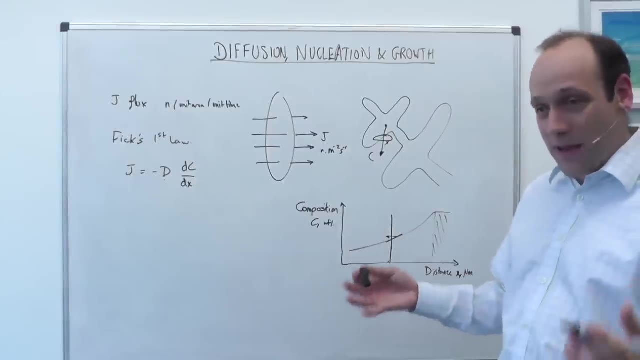 observed to be true. it's just an observation, and this d that's, if you like, the tendency for atoms to diffuse. so it's generally observed that big heavy atoms, things like tungsten, diffuse very slowly and light atoms, things like aluminium, diffuse quite fast, and that's a attribute to 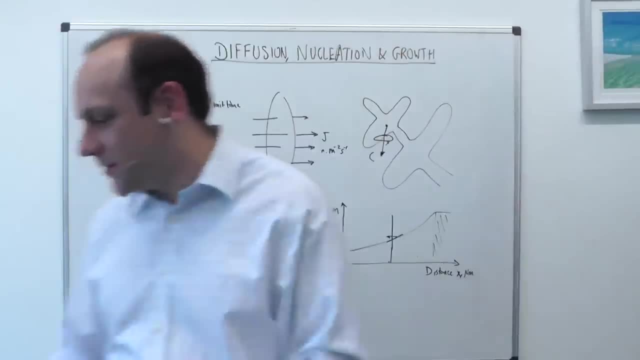 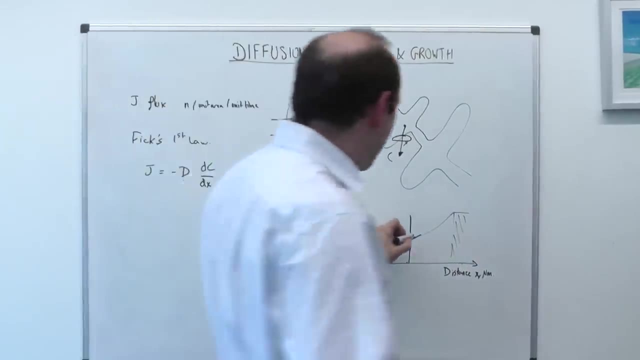 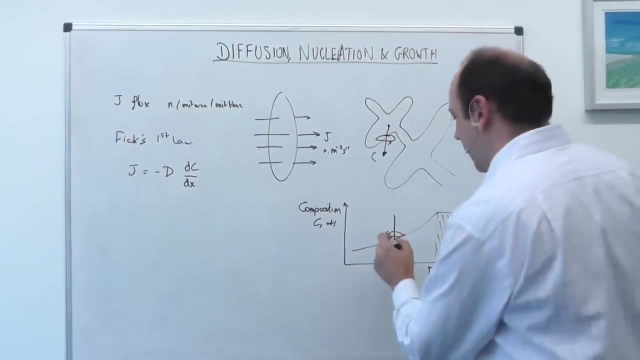 the diffusivity d. so that's Fick's first law. now, if we think of atoms as being here, as jumping from one side to another, according to some thermal activation process in, and so it might be possible for atoms to also jump the other way. so we've got atoms jumping. 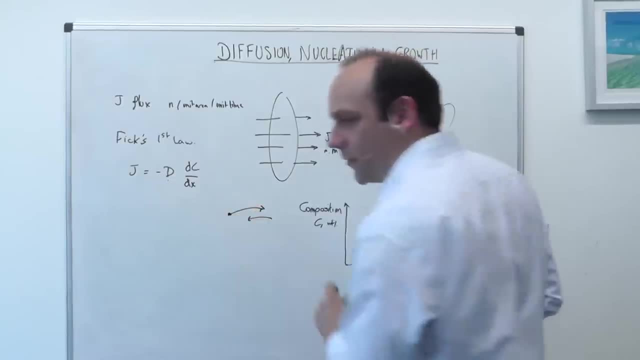 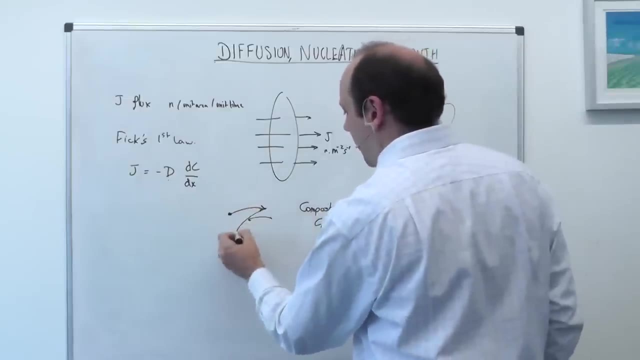 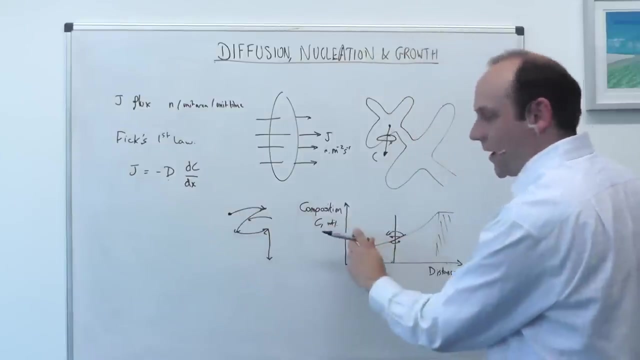 forwards and some atoms here jumping backwards, there, if you like, on a random walk. so that is, the atom might jump here, then it might jump there, then it might jump there, then it might jump there and net. the probability of jumps this way is greater than the probability of jumps that 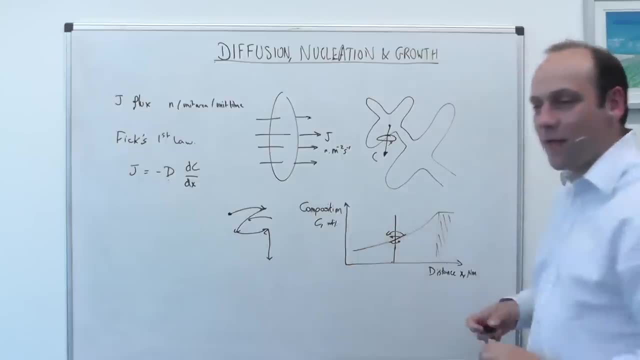 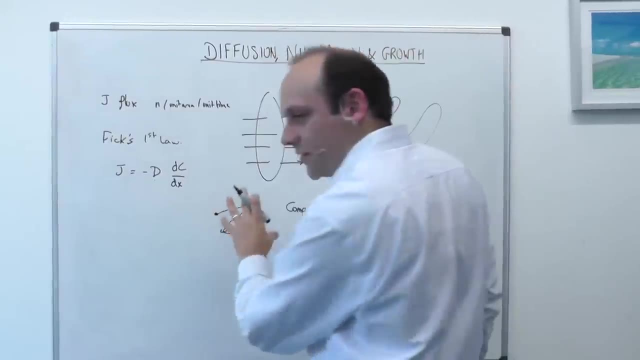 way. that is, they'll tend to net out to going in that direction and we would say that the average distance traveled is proportionate. if the jumps happen at a constant time interval, then the average distance traveled which will cause the jump to be greater than the probability of jumps. 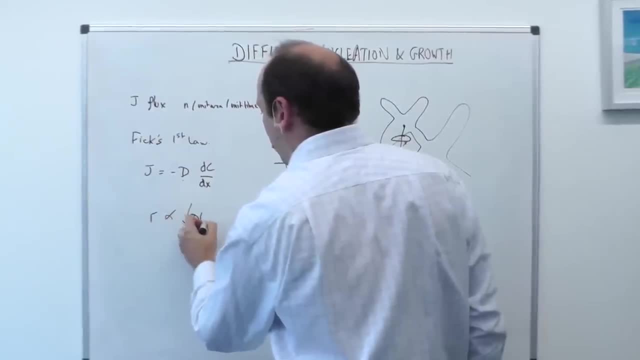 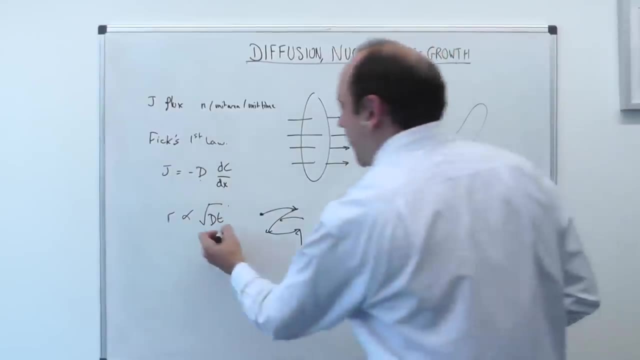 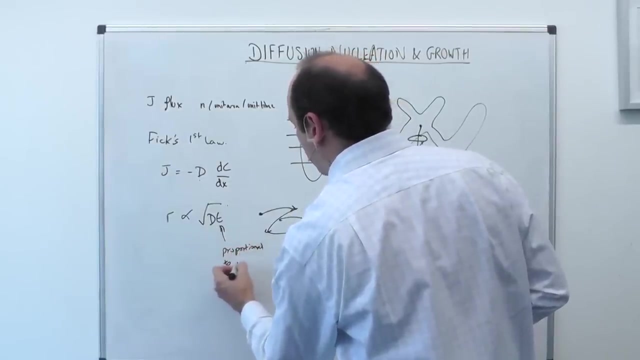 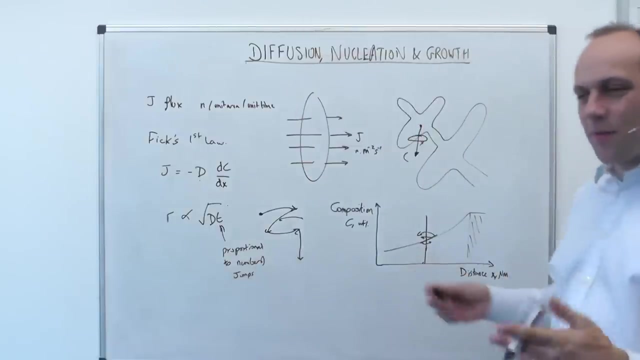 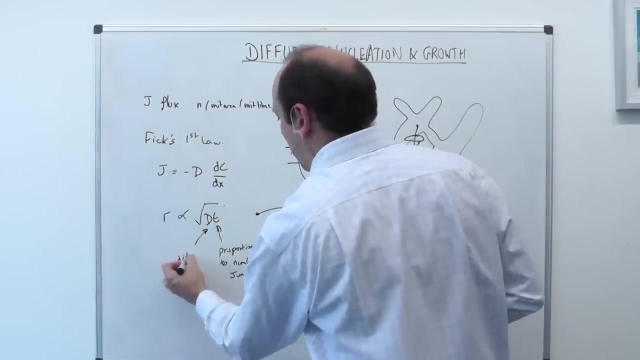 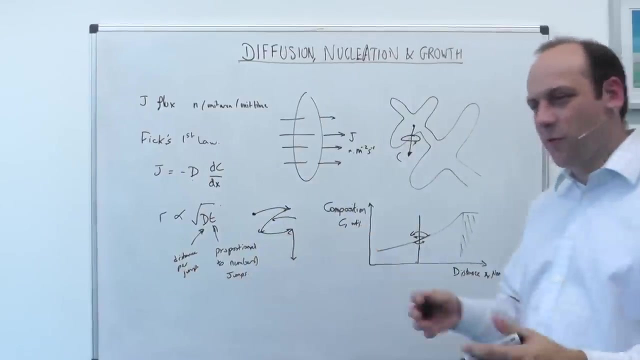 will be proportional to the root of diffusivity, times, time, and you'll see that in in materials physics. so t there is proportional to the number of jumps, of jumps. so they happen. so with the frequency, and d is relating to the distance per jump classically, although obviously in atomic lattice that probably isn't quite true. 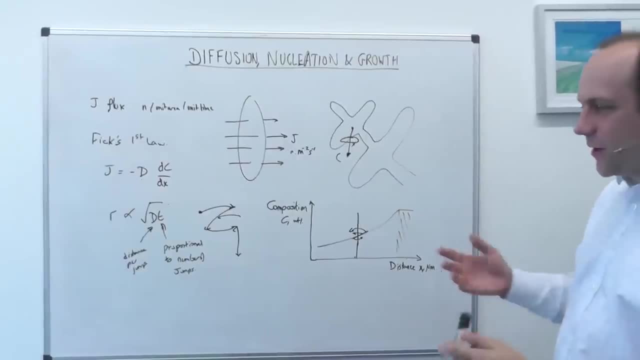 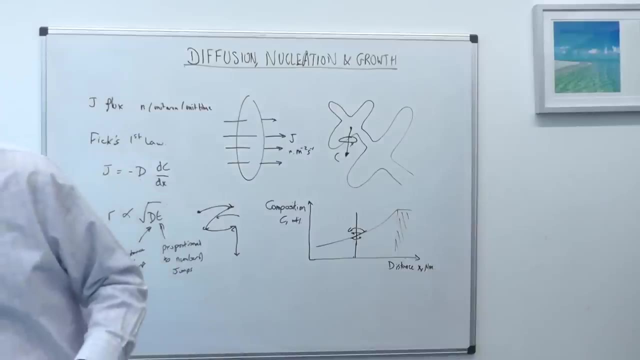 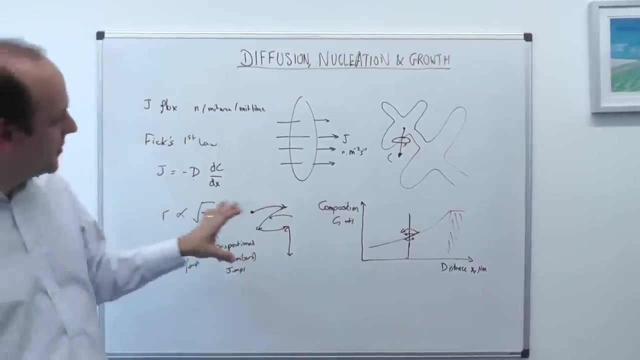 but it's sort of the average distance they move in a jump or how easy it probably comes into, how easy it is, something like that and that's, if you like, an atomic view of diffusion. and if we consider instead the number of atoms moving in or out of a control volume, we can derive- and you'll do this- 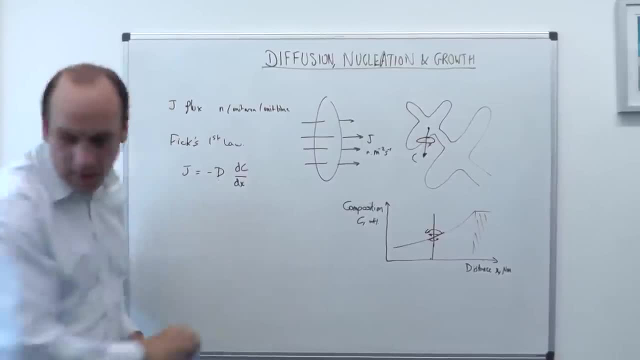 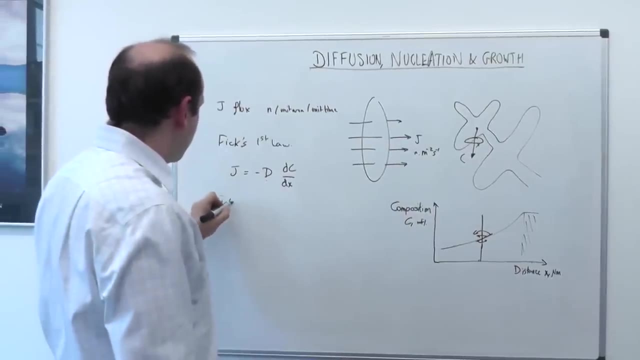 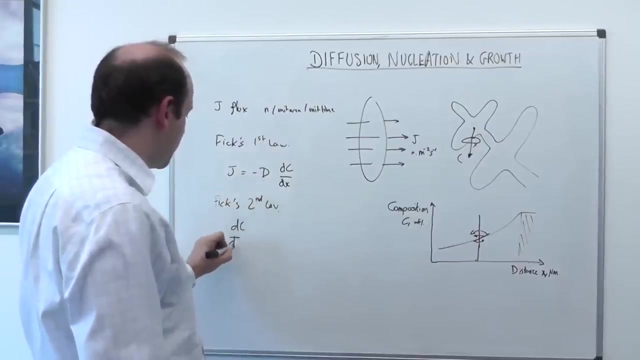 maximally so. so, for example, if we think about a key function which we know that there is an asteroid and we can become very honest with that, then at some point in my application I can come up with aThanks for the long När and take my curiosity and make some quick observations with this功 paper in overcoming the���a. that are so important. our next step is to solve the problem- we usually call this equation- by the use of prevented нос olvosa, therefore the curve work. so this equation we're going to do now, we're going to do this first, I'm going to do the SEAT for eachوب inflation marker. 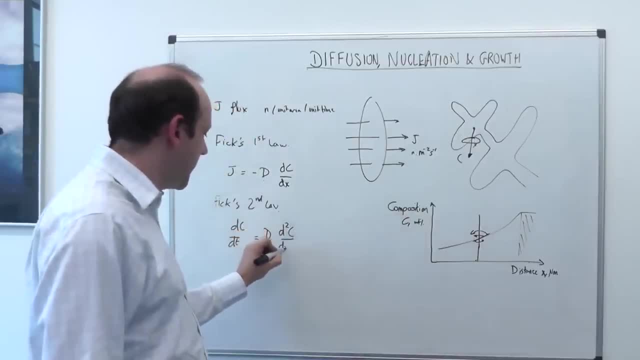 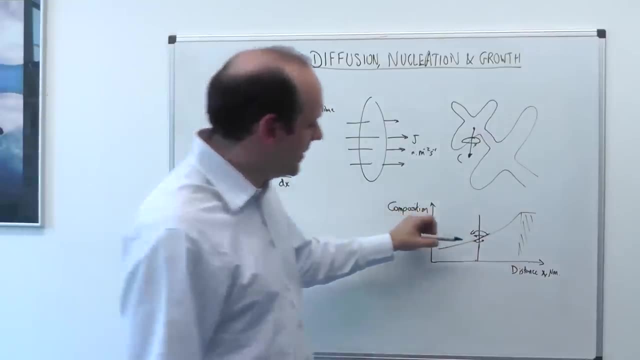 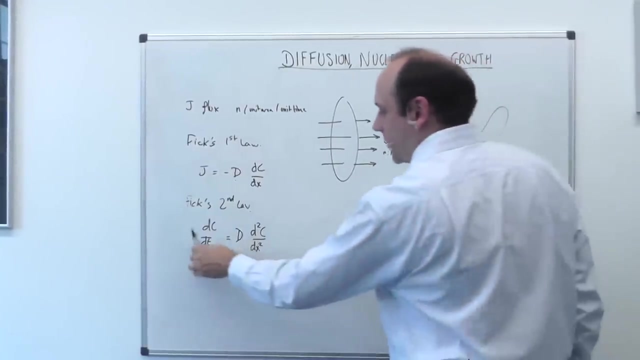 we're going to solve a larger area at two. your have n of ar obviamente you would waw to the corresponding nineteen accelerate, a aiming for by dx squared. so it's the second derivative of the composition gradient. so if this is a constant fixed gradient, that means this has a second derivative of zero, which means that 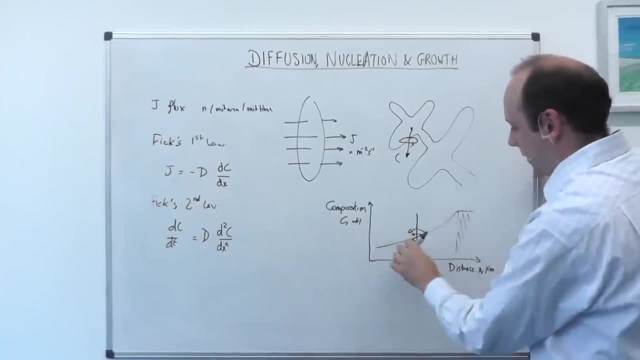 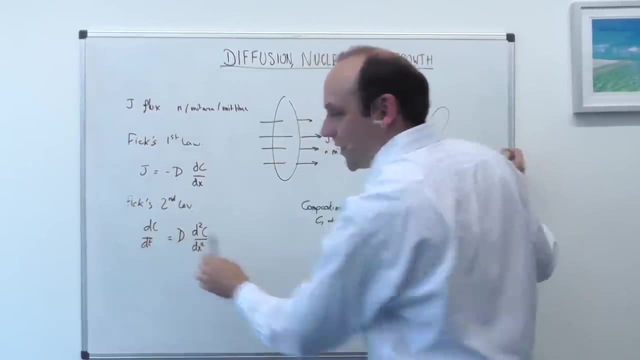 the composition doesn't change with time, but if there's a curvature to it. what this is is: how is the second derivative so how fast is that curvature changing? and that gives you the composition change with time. so it's, if you like, the composition flattening rate or the 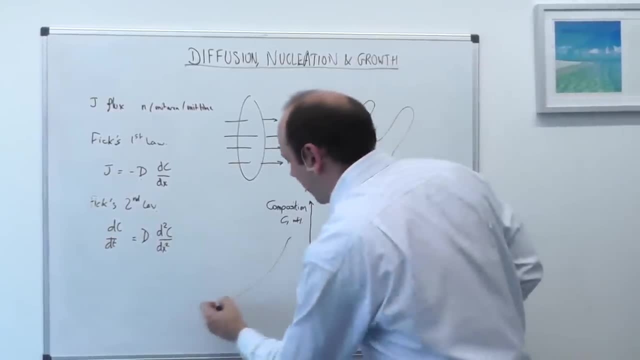 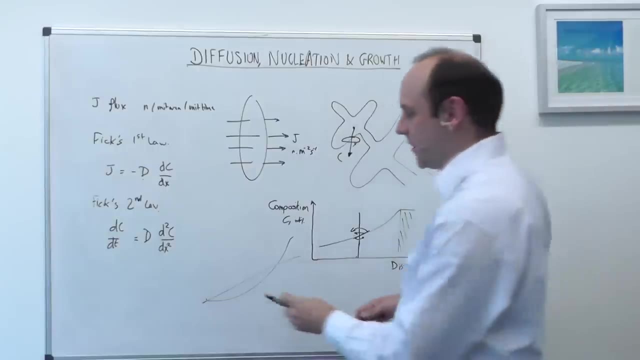 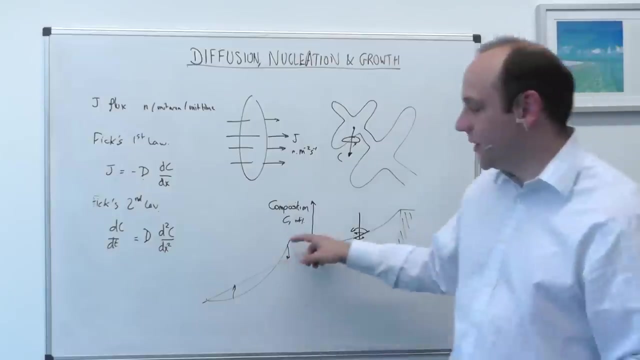 concentration flattening rate, how quickly a curve like this becomes a curve like this, is proportional to the. so this, this flattening rate here- that's how fast this comes up or this goes down- is proportional to the curvature in the concentration profile. and that's fixed second law. and you'll derive that by considering the number of atoms. 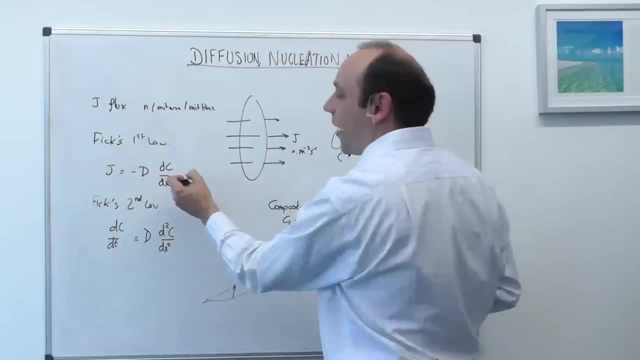 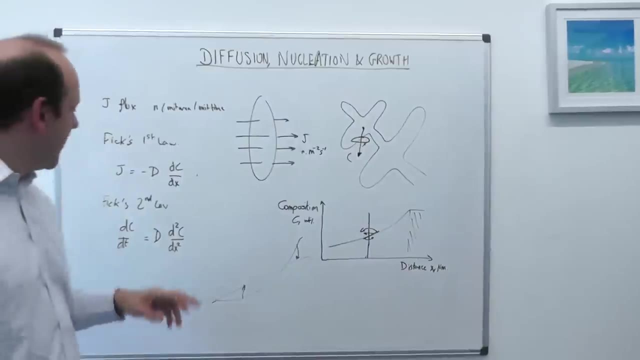 moving by the number of atoms, moving by the number of atoms, moving by the number of atoms moving in and out of a control volume at two different positions. so you'll derive that from fixed first law, but i'll leave that for for 102. now if from our atomic view, then 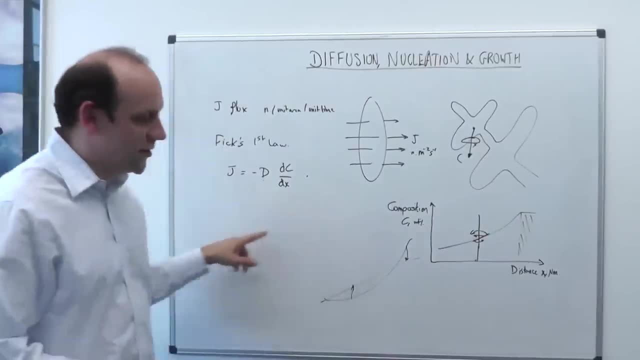 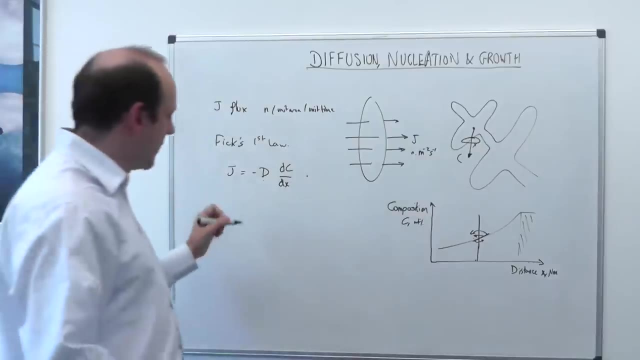 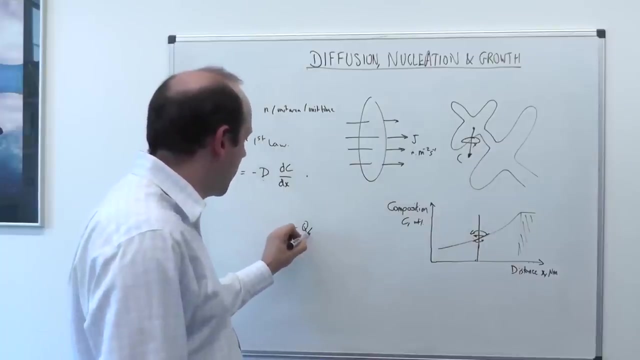 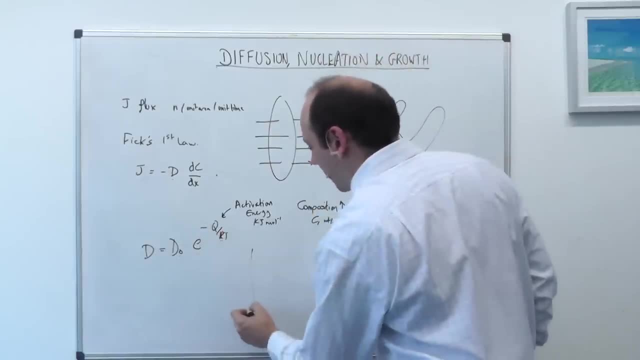 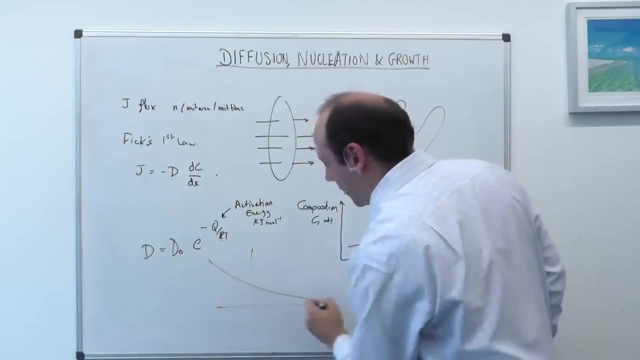 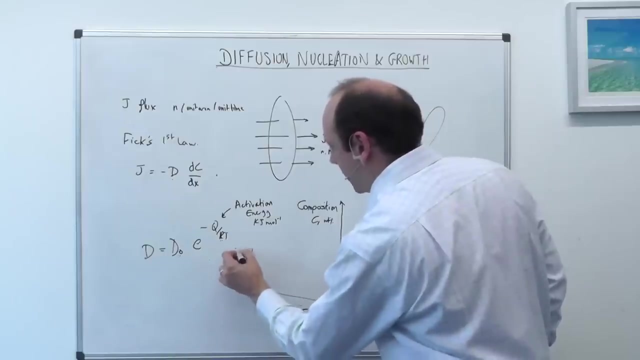 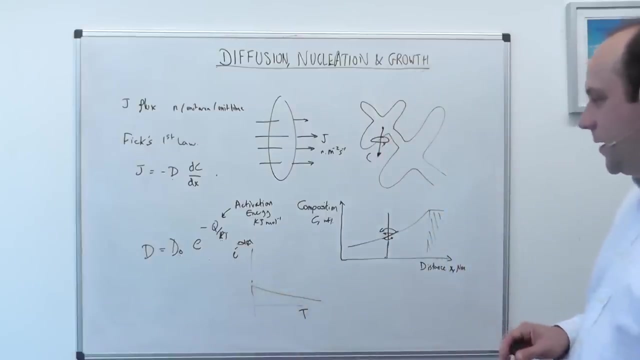 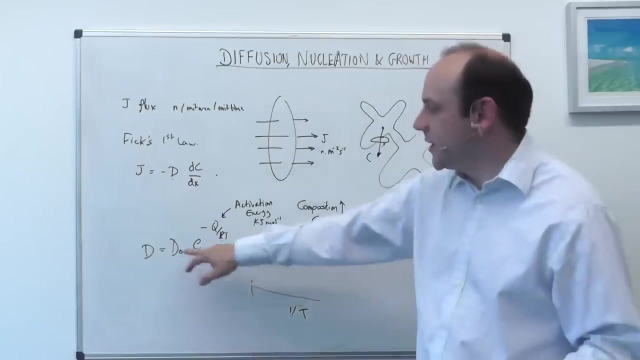 by the number of atoms moving, by the number of atoms moving, by the number of atoms moving at the limit of 15orao, by the number of atoms moving, by the number of atoms moving together, is: is this, is this um and uh, that's what that would look like. um. so this d north, then, is the um? uh. diffusivity at zero. 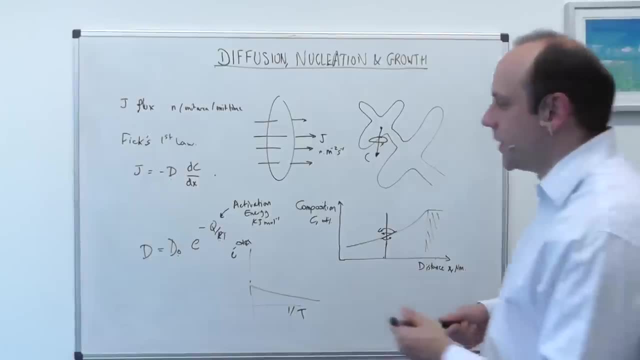 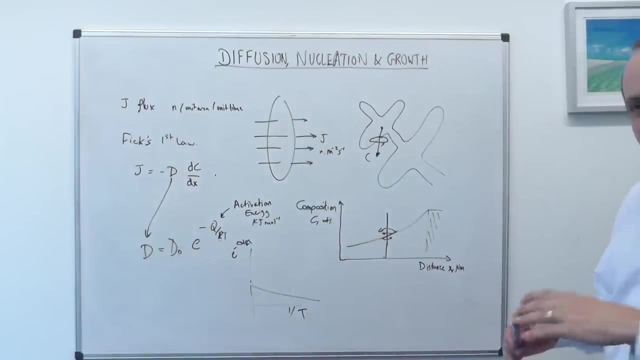 or nearly, as it approaches zero temperature. um, so this diffusivity here is something that varies very rapidly with temperature. so if we homogenize at high temperatures, everything will flatten out quickly, and if we homogenize at low temperatures it will be very slow. so, practically speaking, 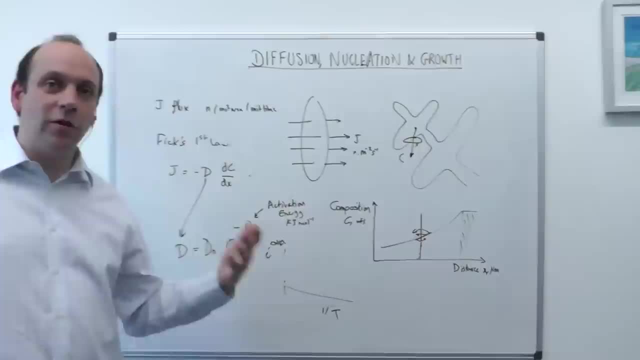 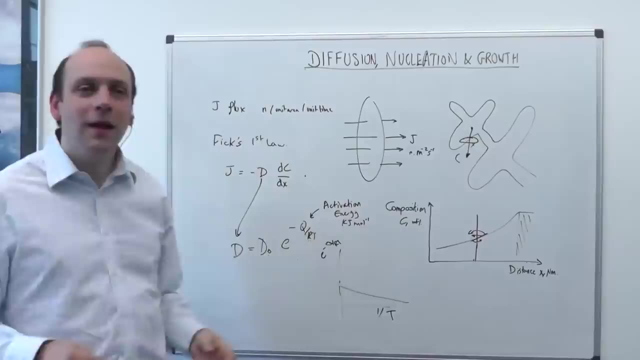 for instance in a, in a nickel super alloy, then there's no real point trying to do a heat treatment to homogenize this out at low temperatures, at six, seven hundred degrees. you need to get up to um temperatures like a thousand degrees and that's for an alloy that melts at 1300. 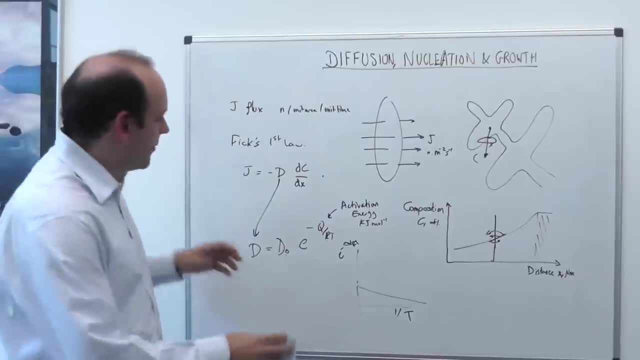 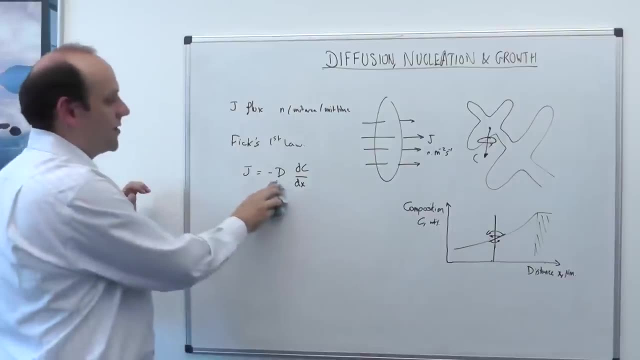 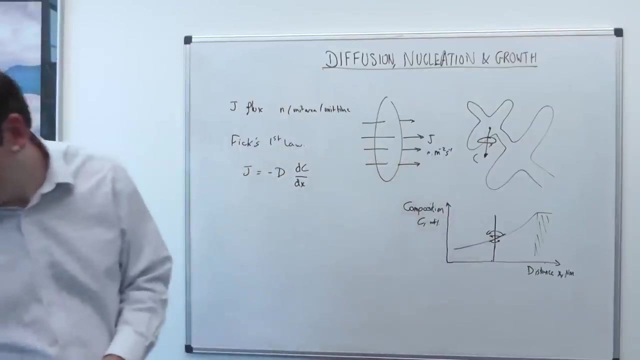 um. so then that's how we would go about taking our ingot that we've solidified and homogenizing it, and the process by which that would happen, and we can do all the calculations for how this would flatten out um, which we were doing in something like 204. so then the the next thing we need to think about. 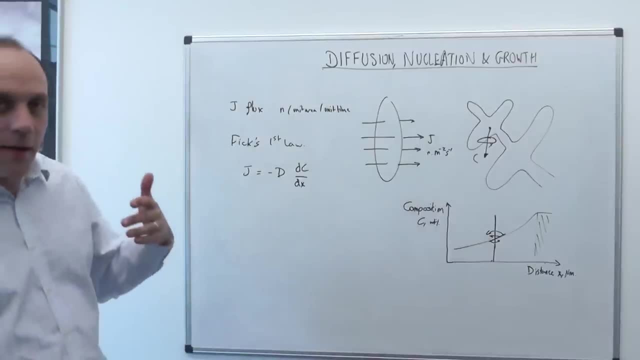 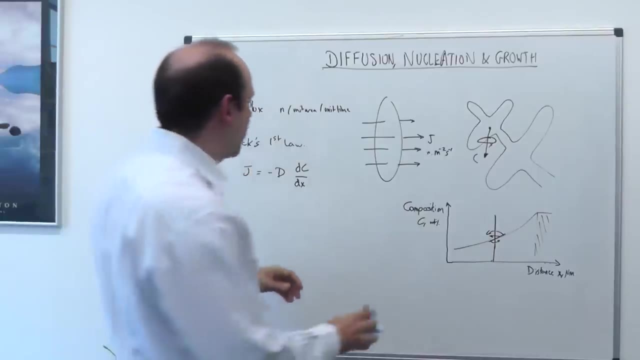 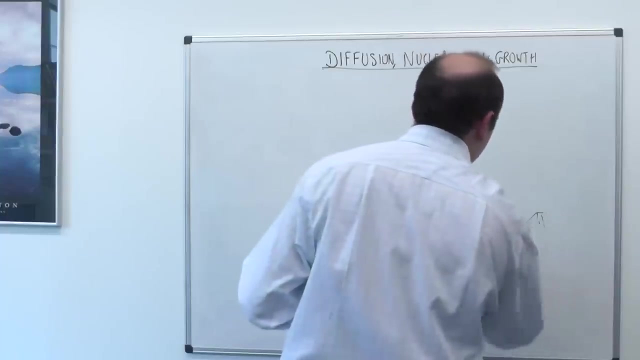 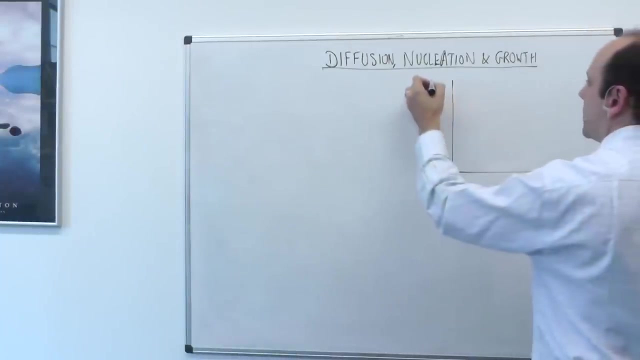 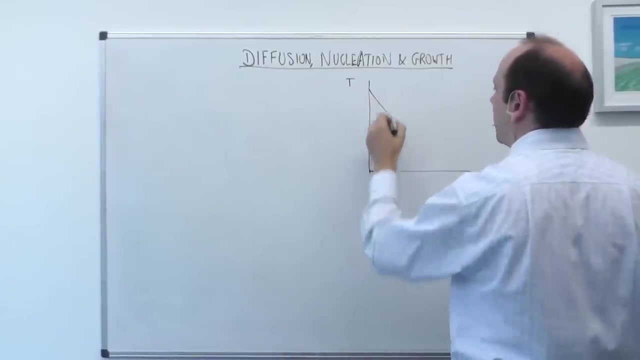 is, if we have a solid um, then uh, how quickly can new phase precipitate out within it? so just to sort of sketch a microstructure, let's see what that looks like. so uh say, we have a phase diagram, so this is um, temperature, this is composition, um. and we have a phase like, say, 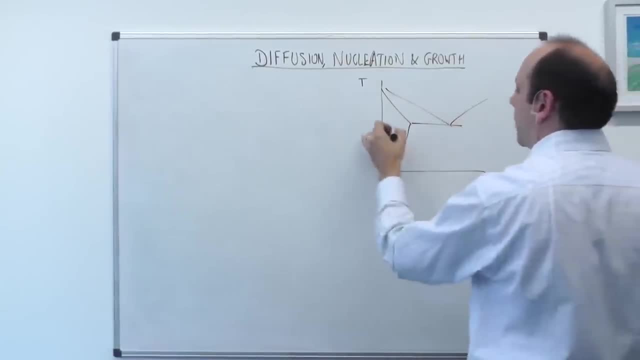 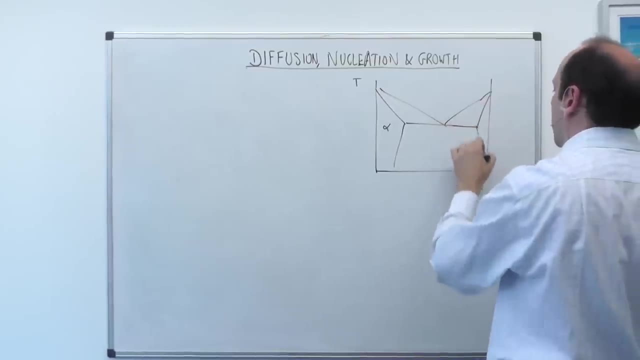 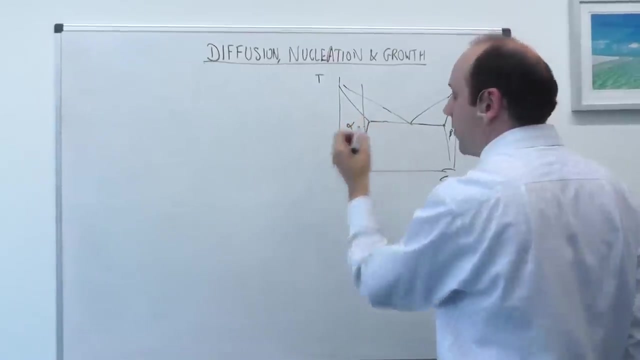 it's a eutectic phase diagram, nice simple one. um, we have a phase alpha here and you know, somewhere over here there's going to be a beta phase. um, and say we're here or no better yet say we are here and we were in the solid alpha phase. so our microstructure looks like this: 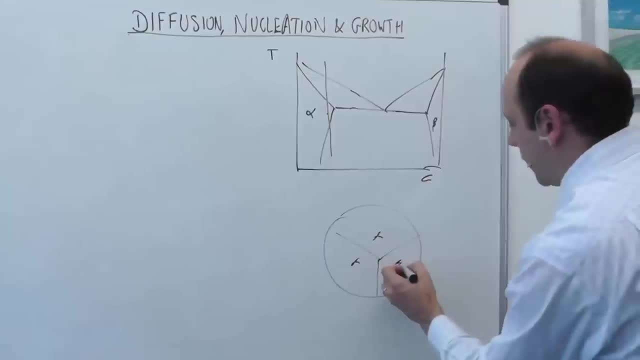 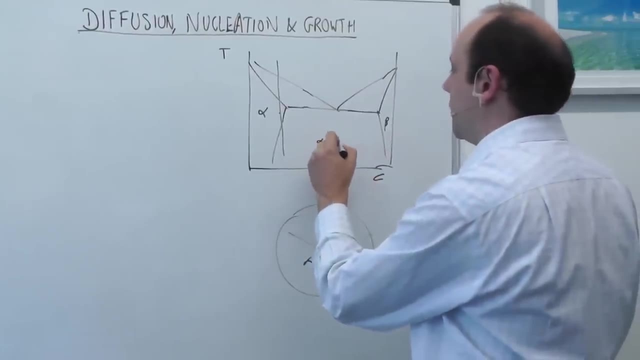 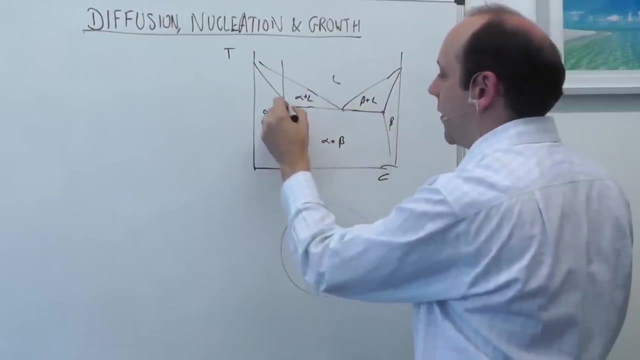 something like this with alpha grains, and previously we've said that we would probably nucleate the new beta phase when we came into this alpha plus beta region. when we came into this alpha plus beta region, we went from here in this alpha region to here. then we'd probably start to nucleate the beta phase at the, the place where there's lots of. 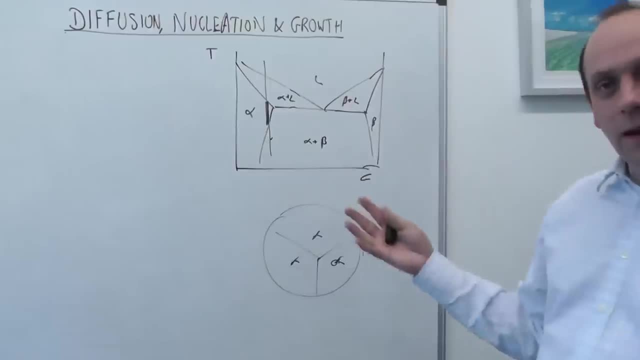 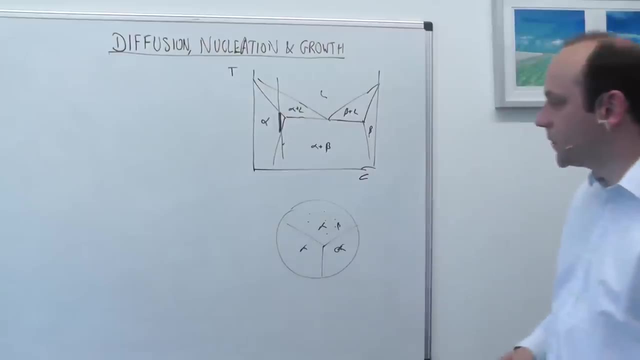 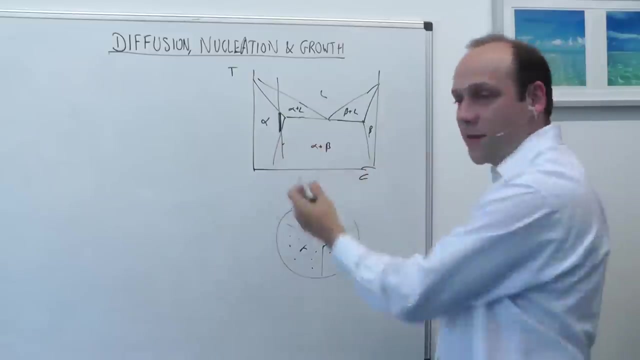 energy to do that at the grain boundaries, but if this is at a very low temperature that might not be possible. you might nucleate new little phase and then you're going to have a beta phase, and that's how we would then start to form our beta phase. and we can think about that from a 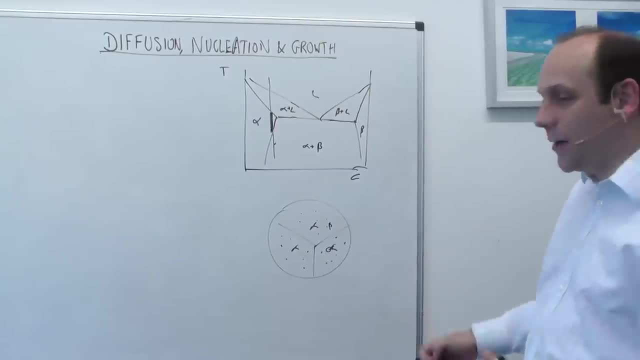 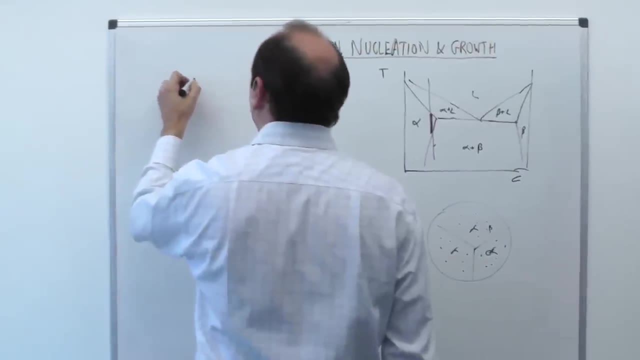 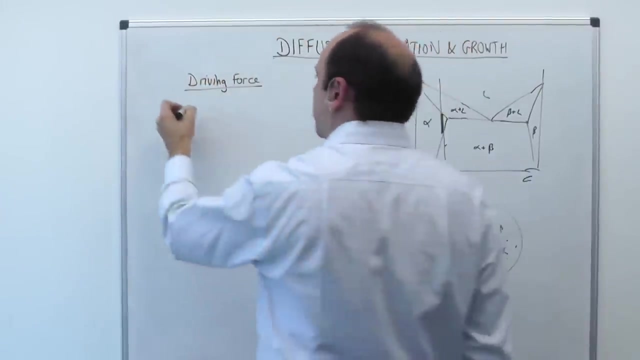 thermodynamic point of view, actually to get how quickly that might happen and start doing some math to describe that. so we're thinking about what's called the thermodynamic driving force. so if we write the gibbs energy as being delta h minus t, delta s hopefully starting to get. 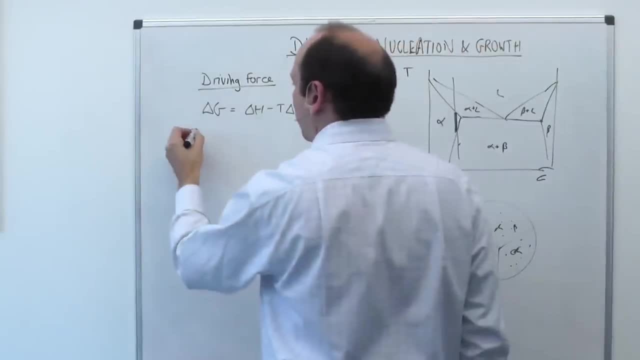 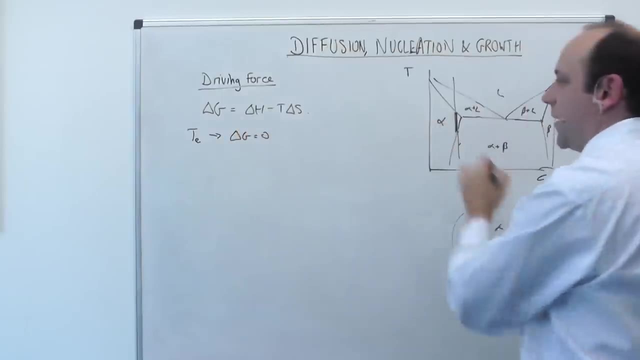 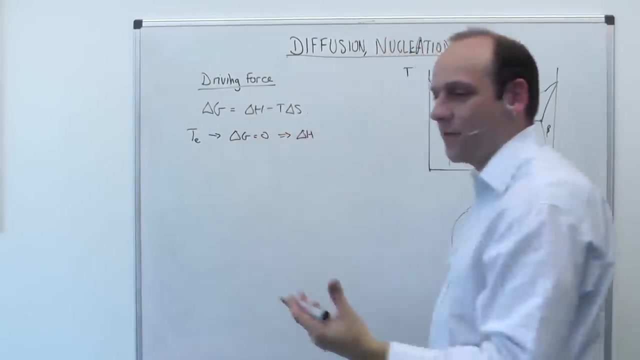 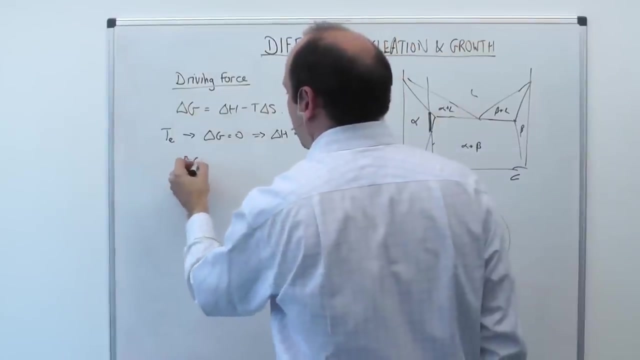 familiar with that equation now. and at the equilibrium temperature te, then delta g is equal to zero. so at the phase boundary here, and therefore delta h at that temperature is equal to t equilibrium delta s. so we can substitute for delta h in here, so delta g um as a function of temperature. 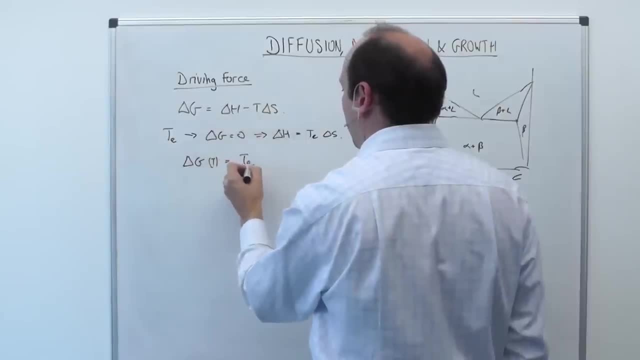 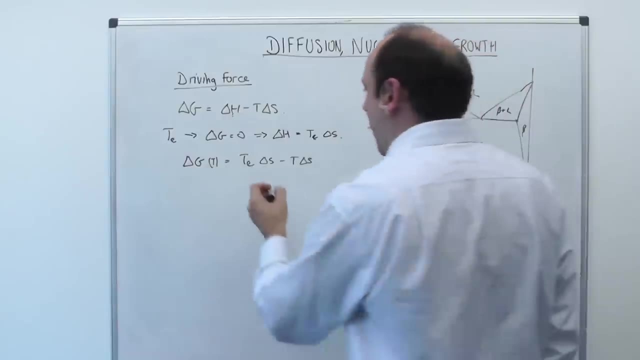 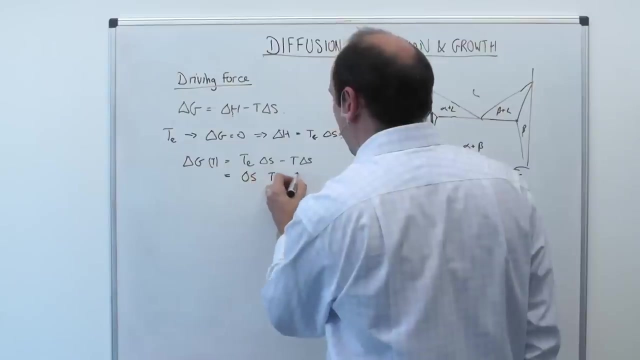 will be then equal to t equilibrium delta s minus t delta s, because we're substituting for delta h in there um, and so we can write this as being delta s um times t equilibrium minus t. so if we're at a temperature of delta h and we're at a temperature of delta s, 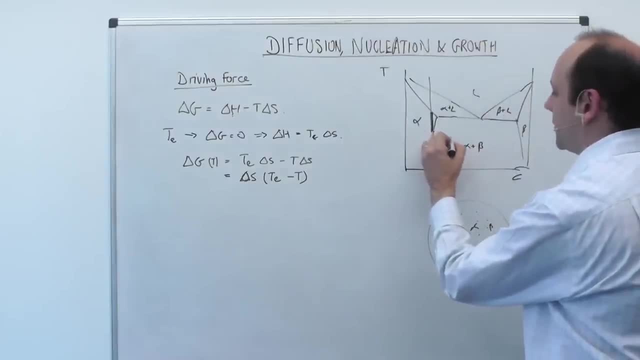 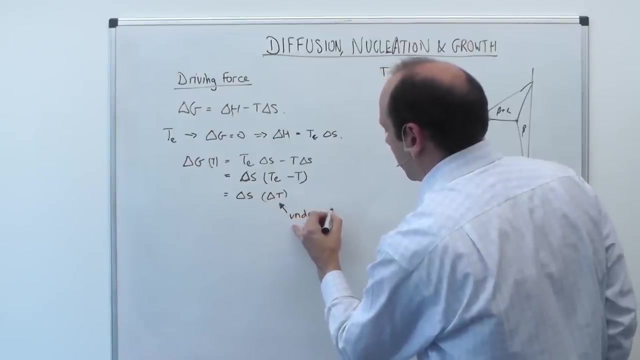 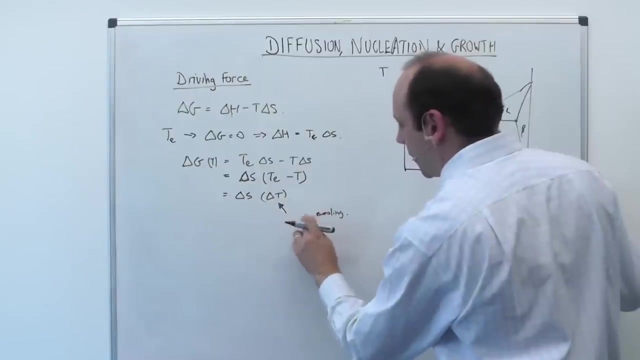 and we're at a temperature below the equilibrium transformation temperature. this delta t here, and that's equal to delta s times this delta t, this amount here, and that's called the amount of under cooling we have. so this is the or the super cooling- it's another term, that's a synonym for it. 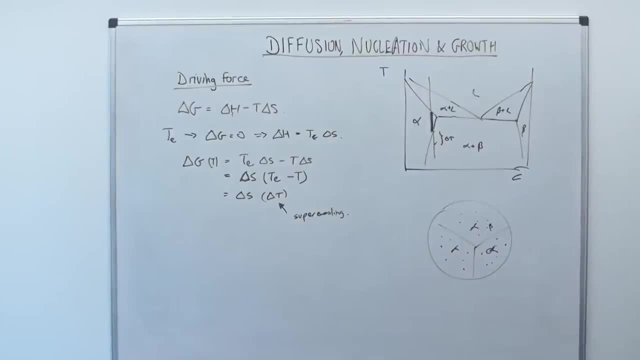 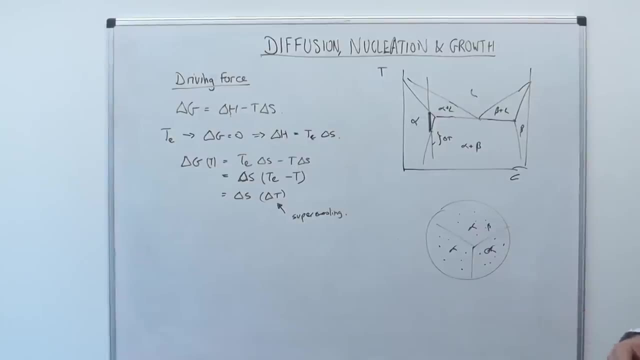 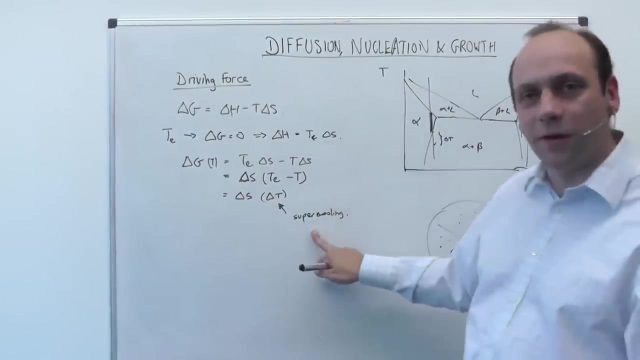 so, for instance, if you take very, very pure water that you filtered very nicely so that it doesn't have, um, any bits of dust in it, um, and you put it in your freezer, you'll find that quite often it won't freeze because until you go to very high super coolings, because it doesn't have any nucleation. 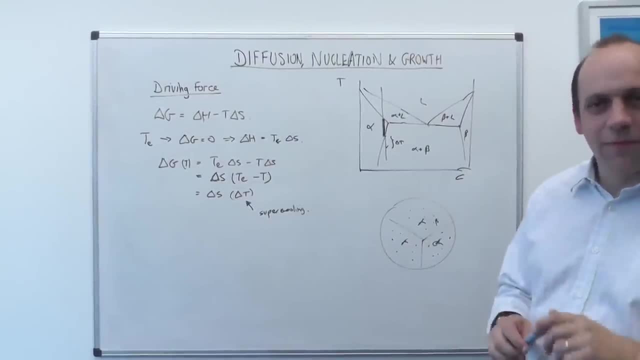 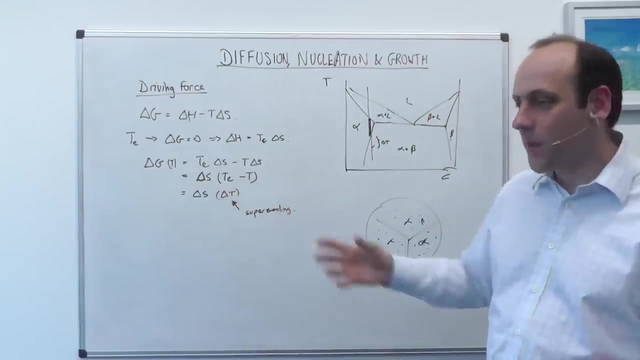 sites. you need the little bits of uh specks of fluff or dust or particle particular in there in order to give it some sites to nucleate from um, in order to give it some sites to nucleate from um, in order to give it some sites to nucleate from. 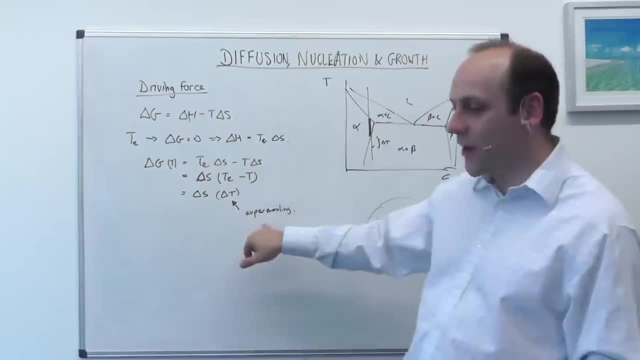 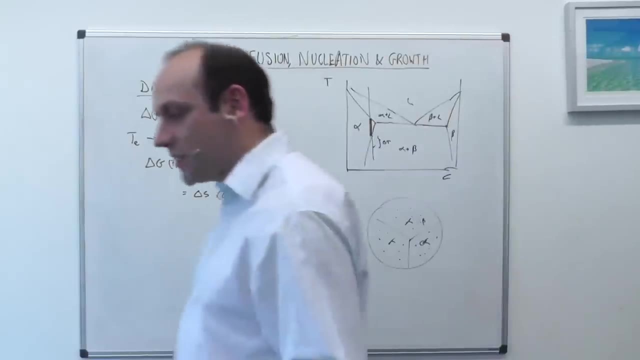 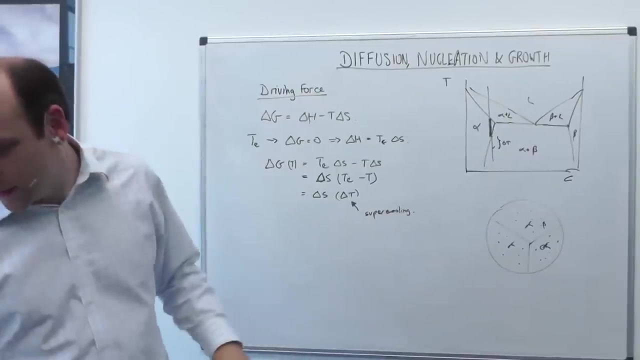 in order to have an um, and if you don't have that, you need a greater amount of energy driving it to produce ice crystals, and quite often in a material we don't have many places to nucleate things from, but so let's think about that. having done that, having 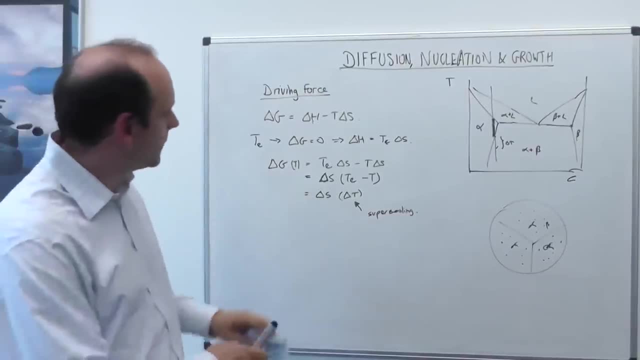 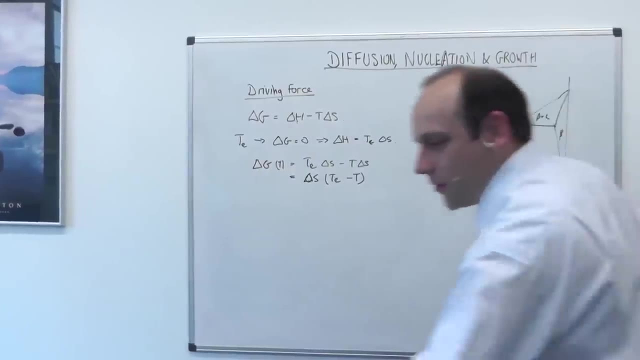 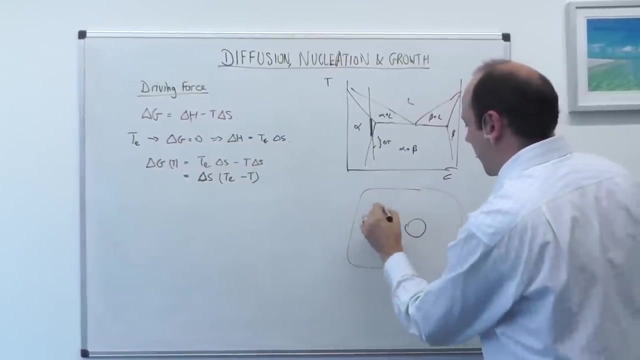 derived an expression for delta g. um think about that situation. so we're thinking about a situation we zoom in on one of those alpha grains in that micrograph And we think about a situation when you nucleate a little amount. so we're somewhere in a C of alpha and you nucleate a little amount of your new phase. 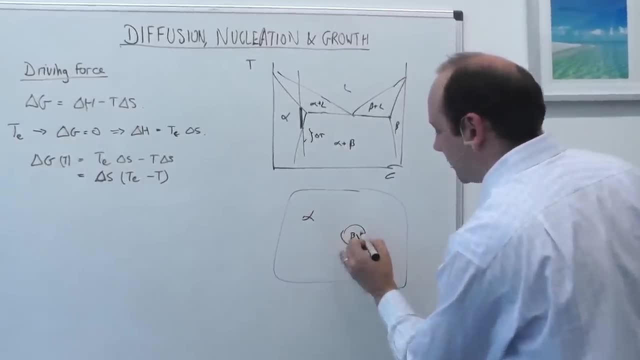 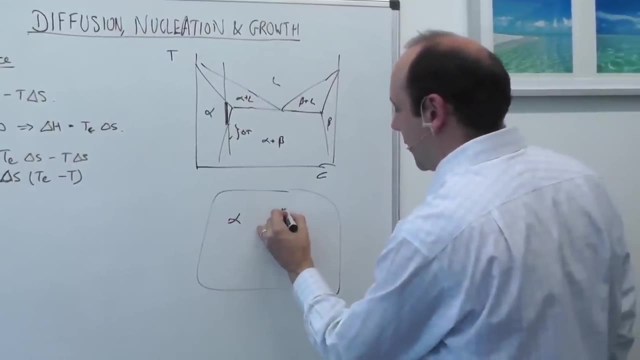 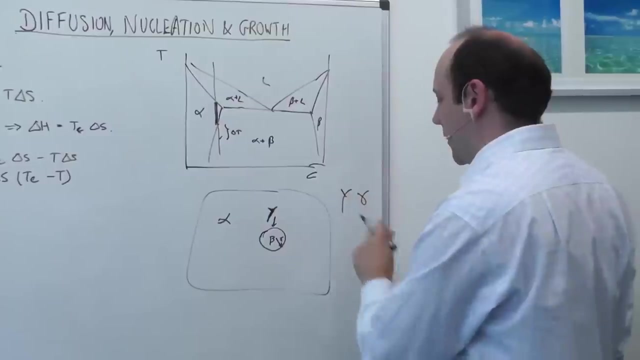 And say it's got a radius R here, And say that there is an energy associated with the surface which is gamma. So you draw gamma like that. So you can draw gamma like that, or you can draw gamma like that. I'll draw it like this. 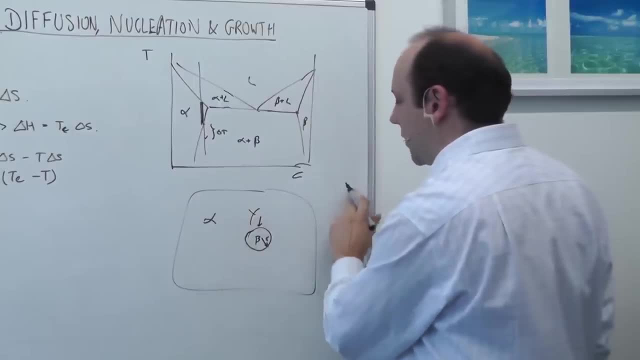 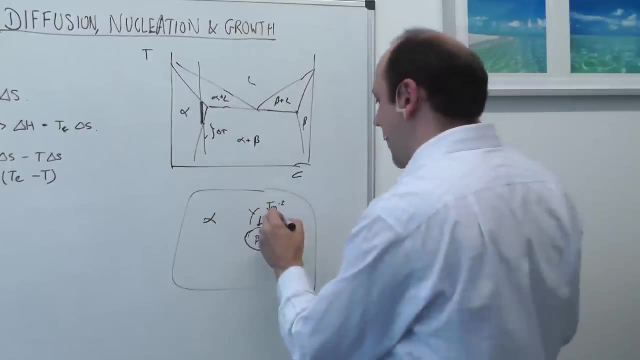 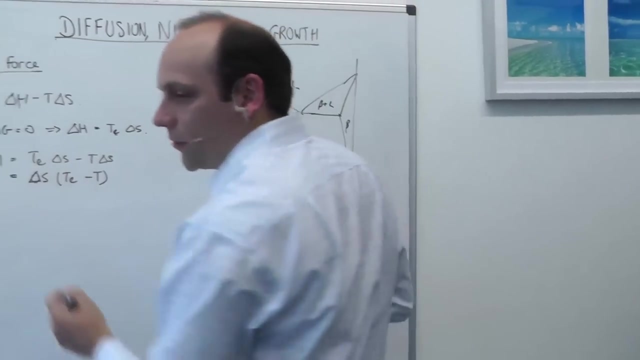 And that's going to be an energy in, if you like, joules per meter squared. It's an energy associated with the surface between the alpha and beta And we've got an energy available from this super cooling, If we say that's our delta G per unit volume. 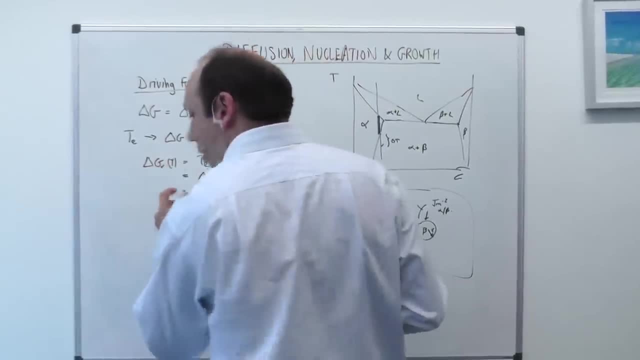 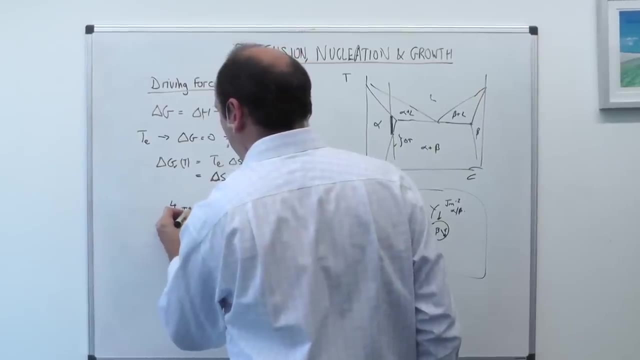 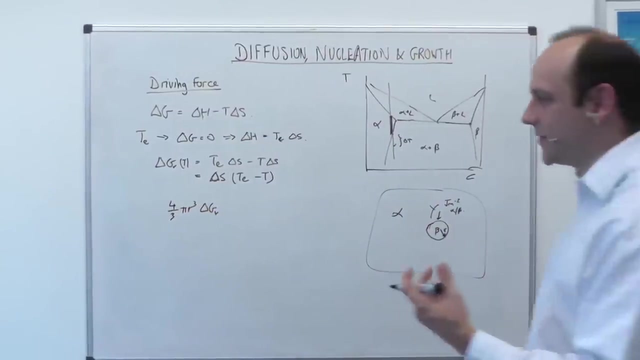 We've got a thermodynamic energy available from transforming that of the volume of a sphere, Four thirds pi R cubed times the amount of it that we've transformed, a delta G per unit volume, And that's an energy that drives it forward. so we'll say that's negative. 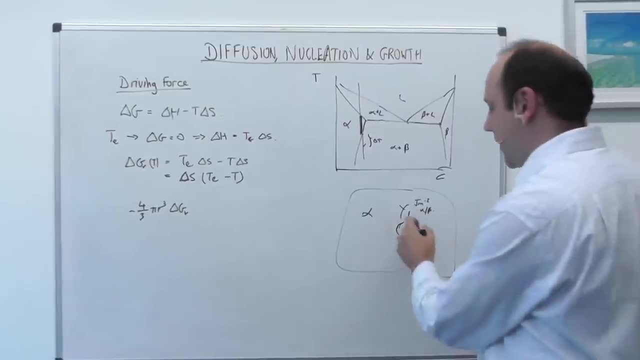 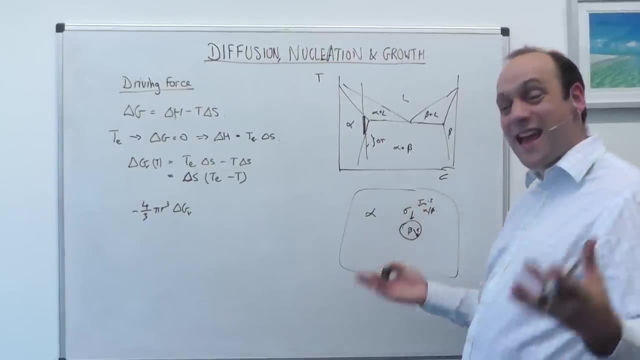 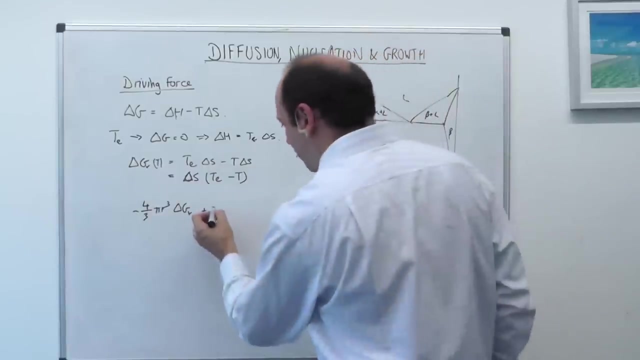 And we expend that on making this surface. actually I'm going to call this surface energy sigma. now another Greek letter, Sigma is Greek letter S for surface. Sometimes, in some other circumstances, we call it gamma. it's just terminology Plus four pi. as long as you define it, it's fine. 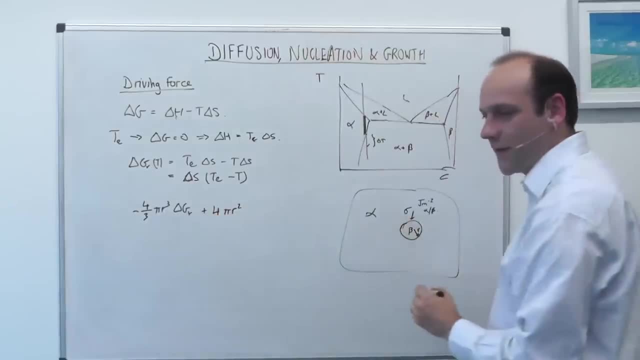 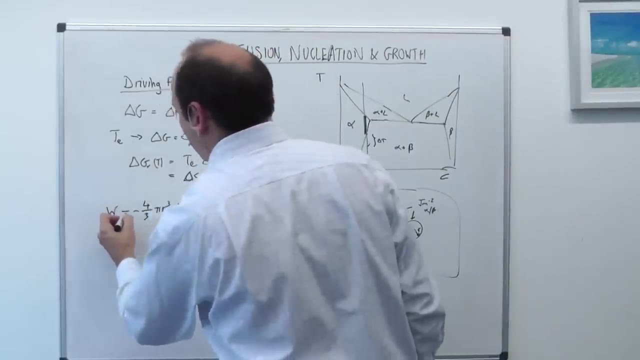 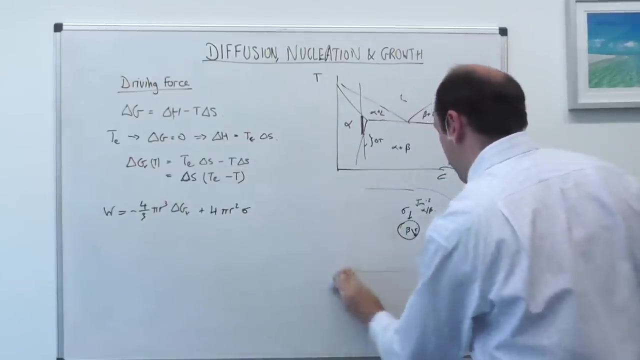 Four pi R squared, that's the surface area of a sphere times sigma, And that's our net energy available to grow that. so we'll call that W, And if you graph that out what you have, I'll actually rub the phase diagram off now. 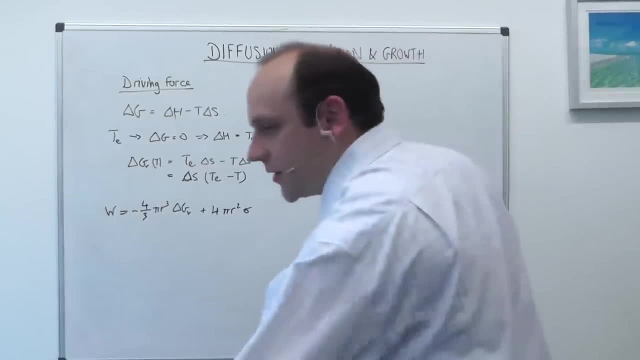 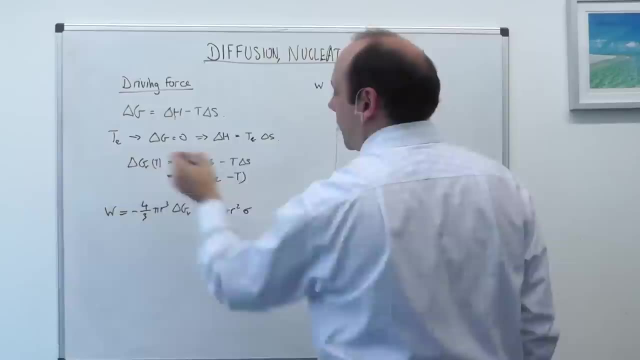 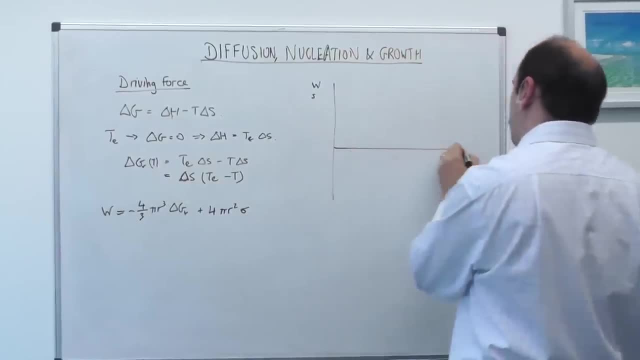 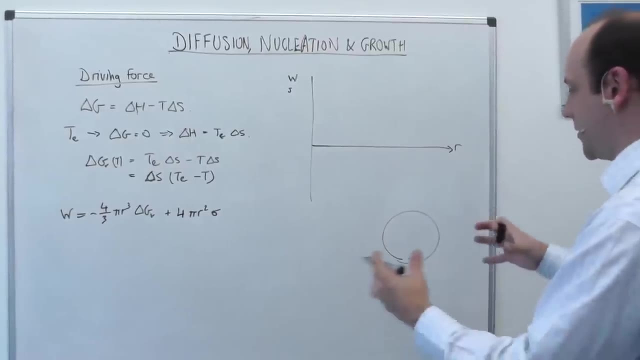 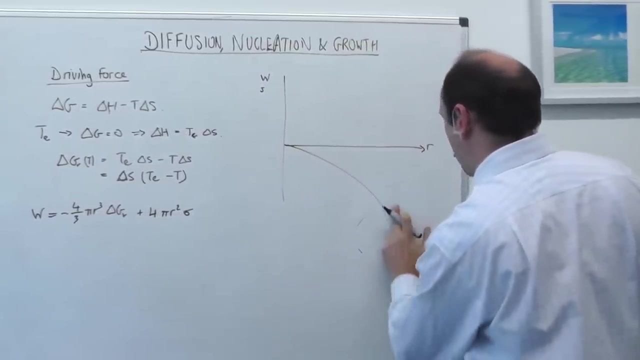 Against the size of the particle R. so we've got a little particle and we're asking what W does. as we change the size of the particle we're nucleating. So we've got here something that goes off as a minus four thirds pi R cubed. 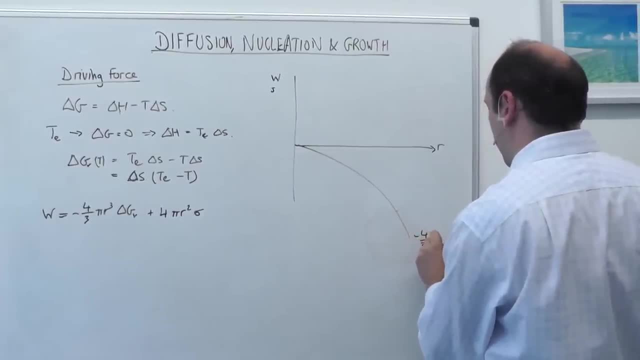 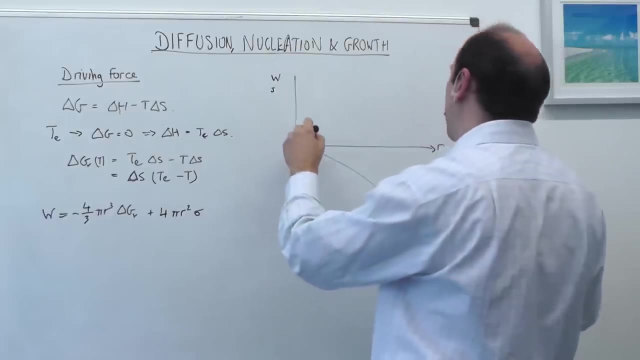 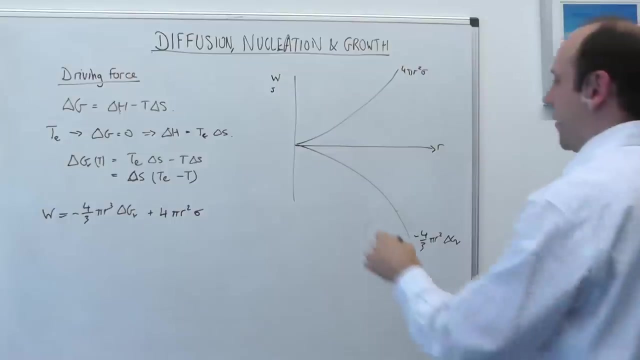 So that's my minus four thirds pi R cubed delta GV, And the other component in this equation is something that goes more gently as a squared term. That's my four pi R squared sigma, And if I add those two together, well, I get a curve that looks something like this: 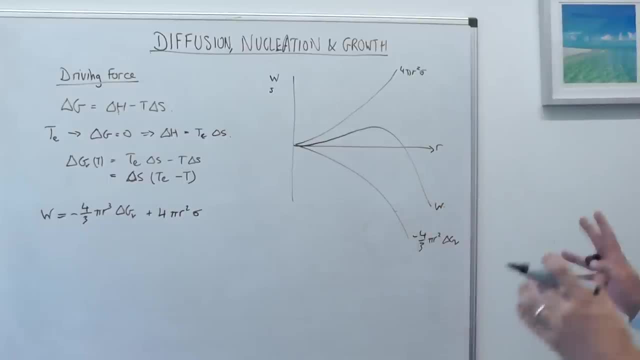 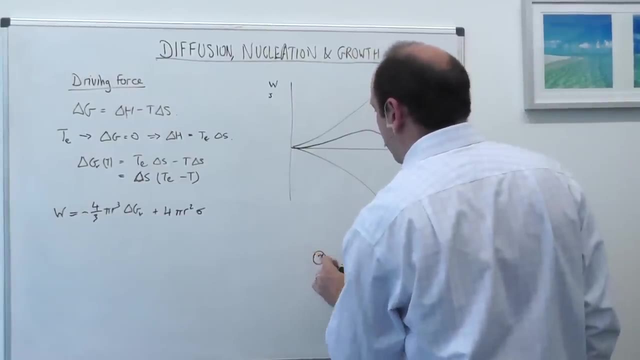 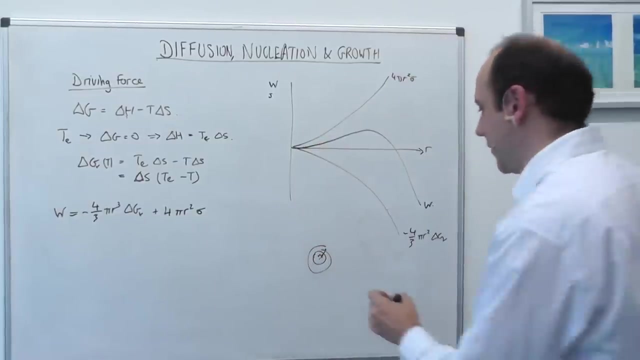 So that's what W looks like. So what does that mean? What it means that For very small particles, things with a small radius R, then actually if you increase them in size by a little bit, by an amount dr, so that's then a radius there of R plus dr. 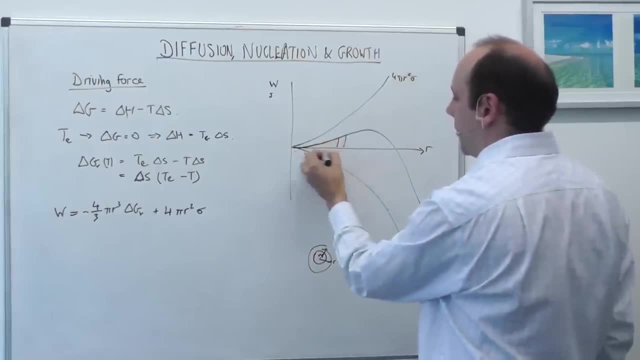 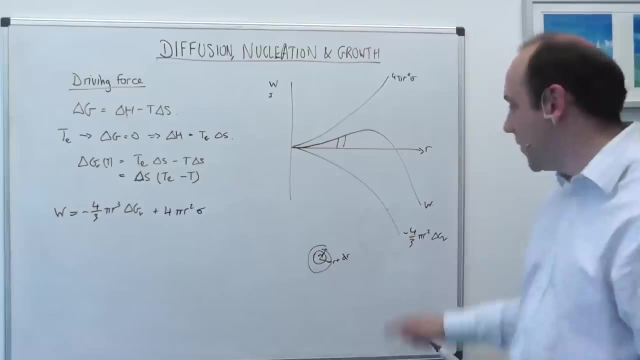 If you increase them in size, say from here to here, from R to R plus dr, then you have to expend you've got. you're spending more energy creating the surface than you're getting from the change in volume, And so that requires you, requires energy. 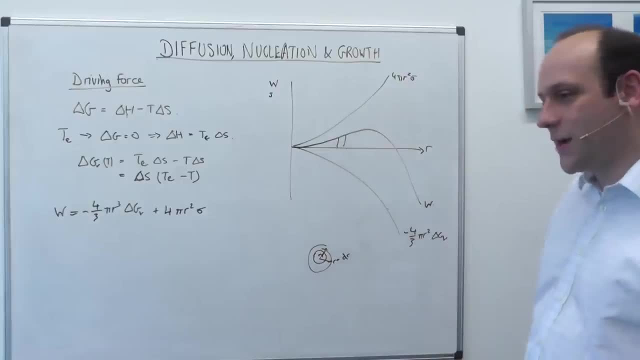 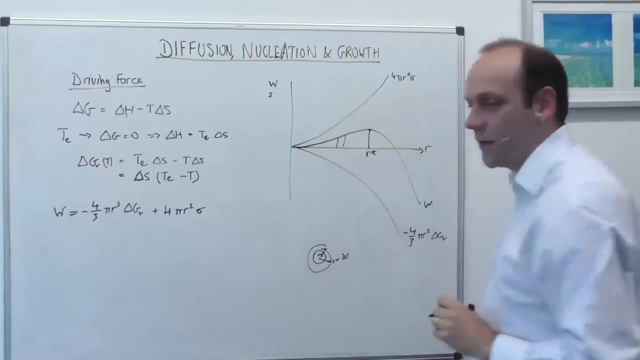 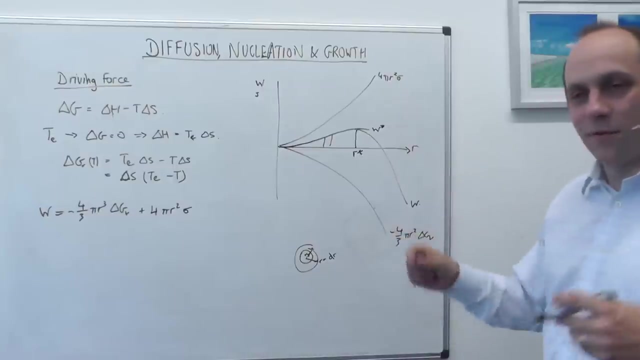 It doesn't give you back energy. So that's an unfavorable thing to happen. But beyond this maximum point here, let's call that maximum point a critical radius R star, And it'll have a critical energy W star as well. Beyond that point, the energy you expend on creating new surface is relatively small compared to the energy you expend on the energy you get from transforming from the alpha to the beta. 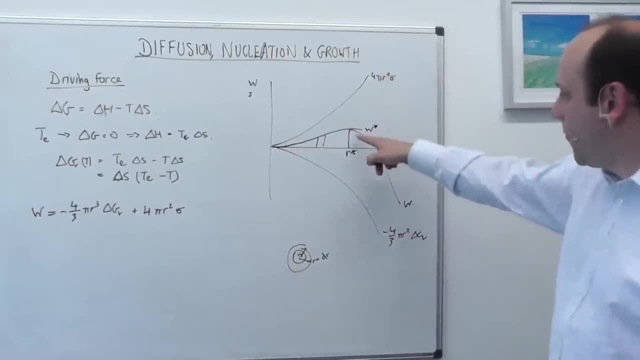 Of course, we know that the Compton Higgs safety isед is a chaotic process. bake face is a洲 whack base. stack up with the and we can, and therefore you need to have a particle of this initial critical radius in order for the transformation to happen. 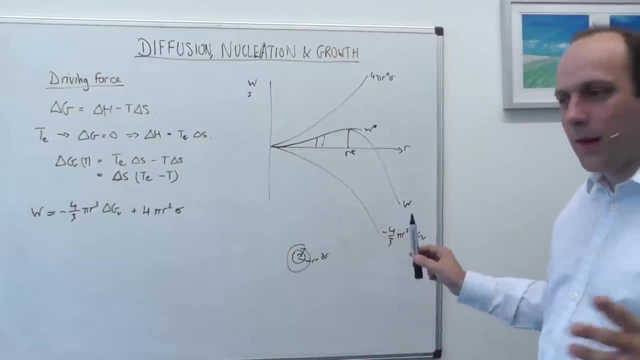 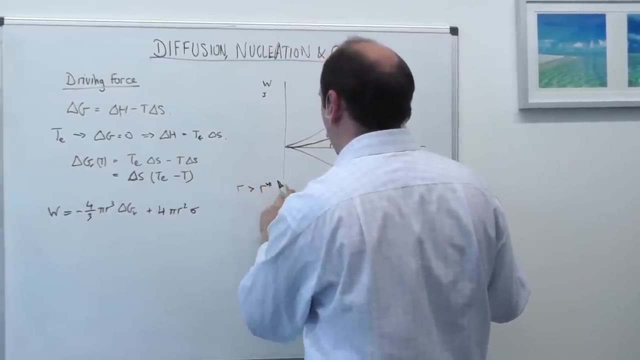 So I'll say that again. So you need to be bigger than the critical radius in order for the transmission to proceed, for an initial nucleus to grow. So if R is greater than R star, and then where's the particle density of it? So you've got Green. 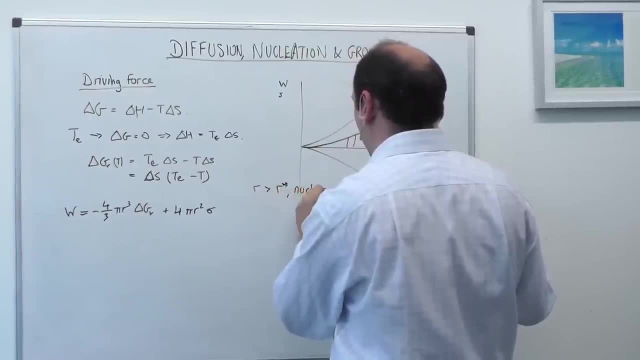 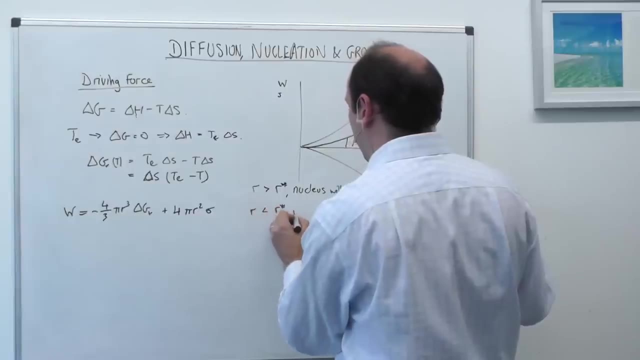 but you've got zero And you know designing R starr when you go up the Internet you've got a's and g for you're having to eat this beautiful exercise. the nucleus will grow and, conversely, if r is less than r star, the nucleus will shrink. 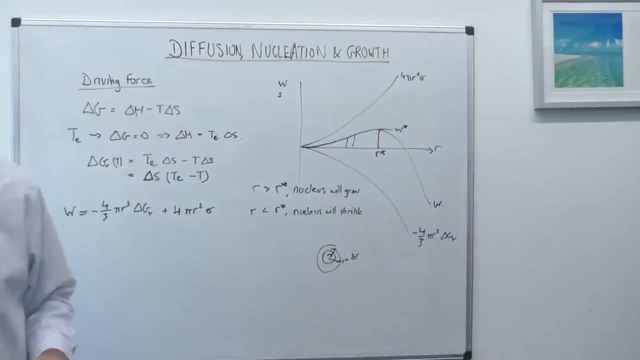 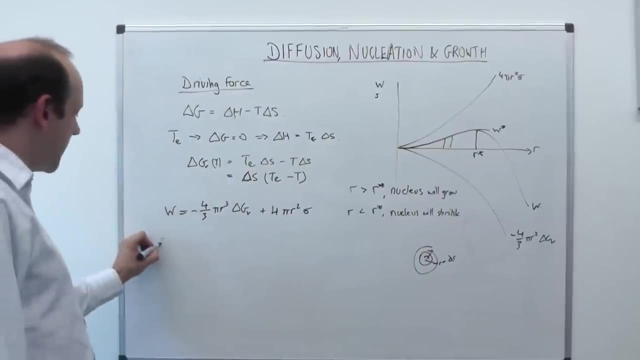 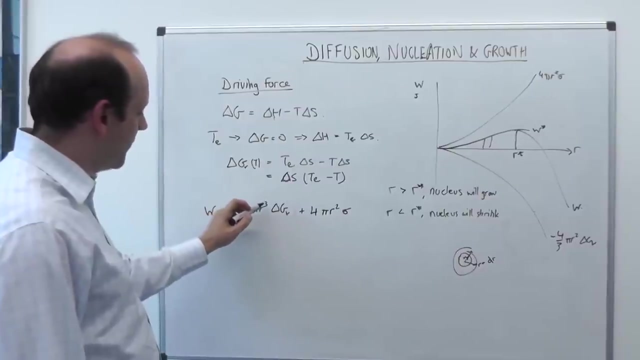 And we can work out then what r star must be. So if we want to find the maximum in a curve, then we just differentiate it, So we can say dw by dr. well, that's equal to minus four thirds pi r squared times three. 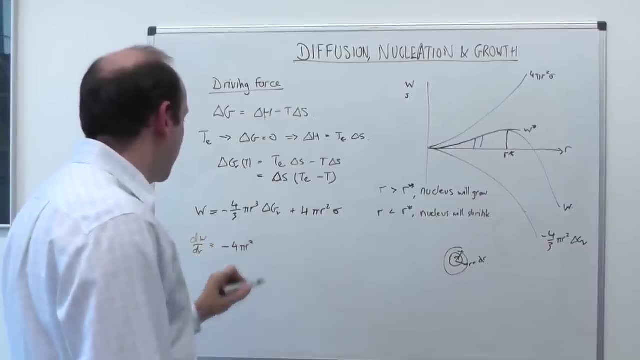 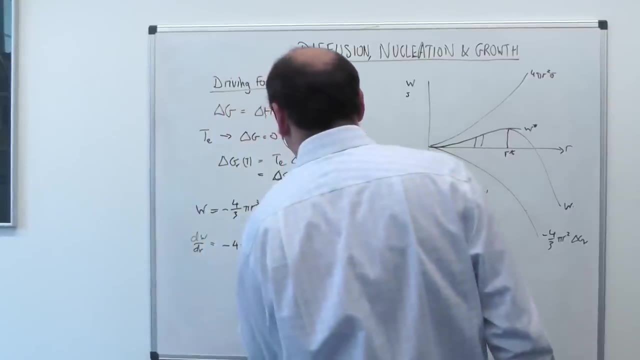 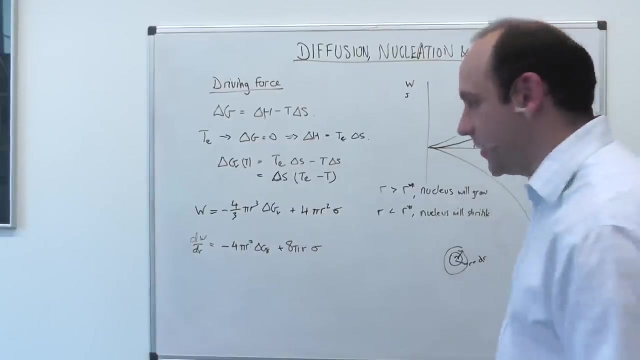 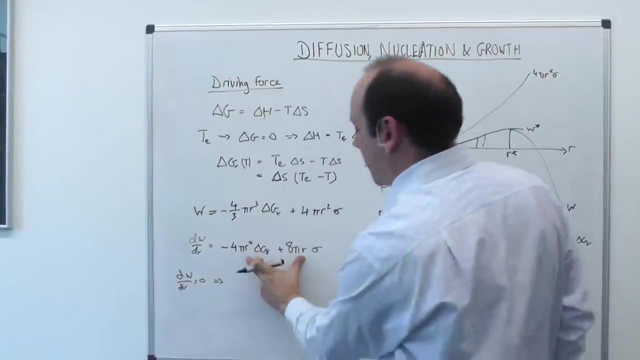 so that's minus four pi r squared delta gv plus eight pi r sigma. Just r squared goes to two r, And at this maximum point dw by dr is zero, And at that point these two things will be equal to each other. 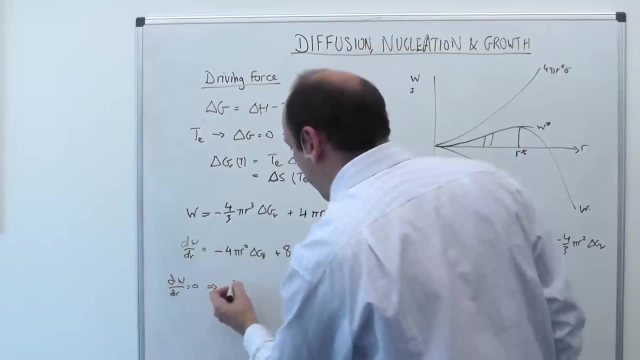 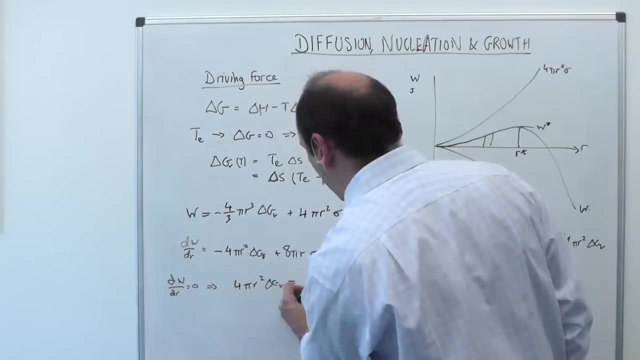 So we've got a zero over here, we pull that over there. they'll be equal. So we've got four pi r squared. delta gv equals eight pi r sigma And we can cancel the pi's. there we go gone. 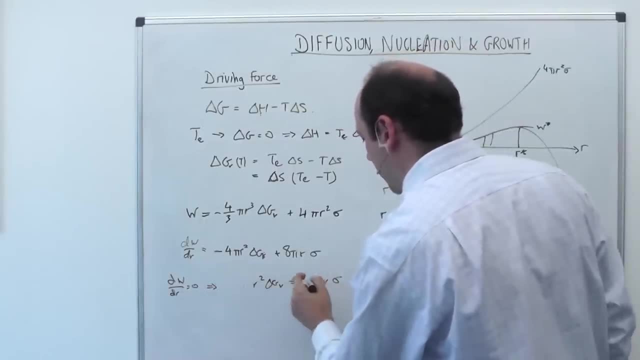 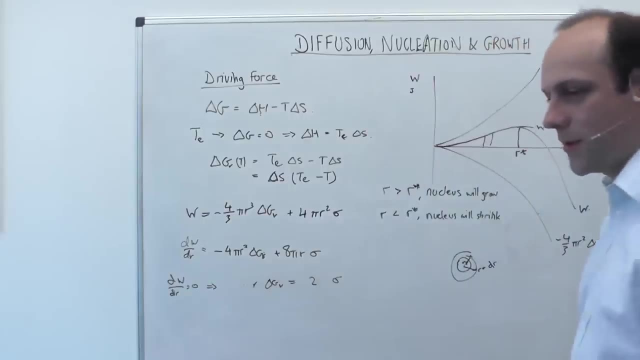 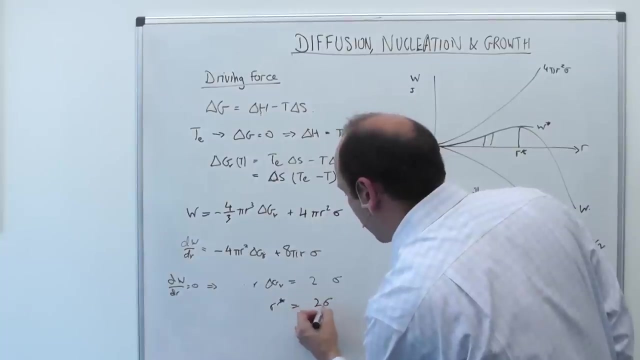 And we can cancel the eight with the four and get a two, And we can cancel the pi's with the four and get a two, And we can cancel the r with the r squared, And then we can say, therefore, that r star at our critical radius is equal to two sigma over delta gv. 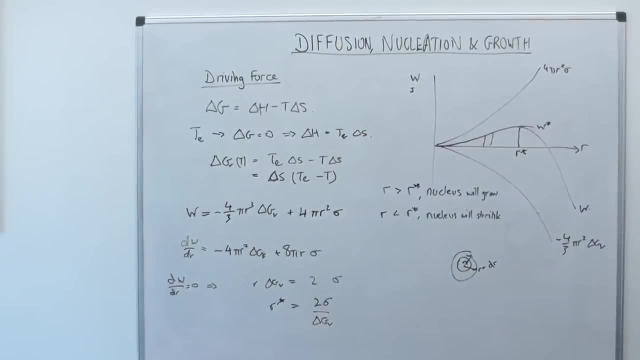 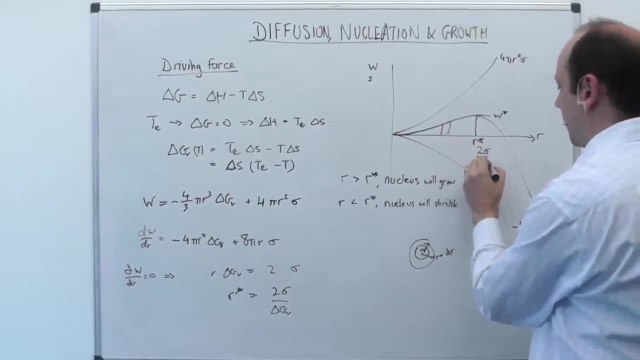 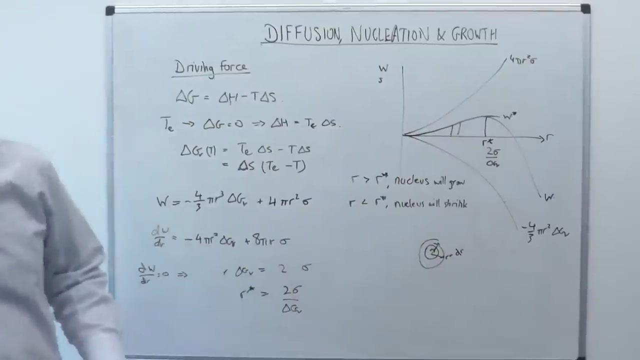 And that's going to be our solution. So this value here is equal to twice sigma divided by delta gv And we can then go and substitute back in to find out what this value is, What this value w star is, by substituting that back in for r into our original equation. 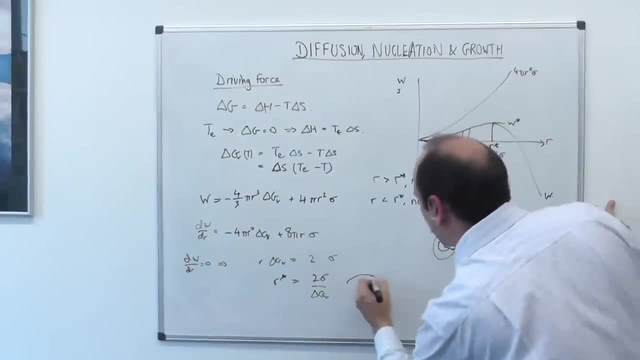 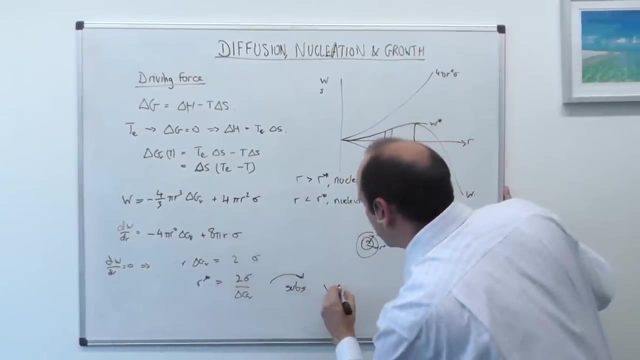 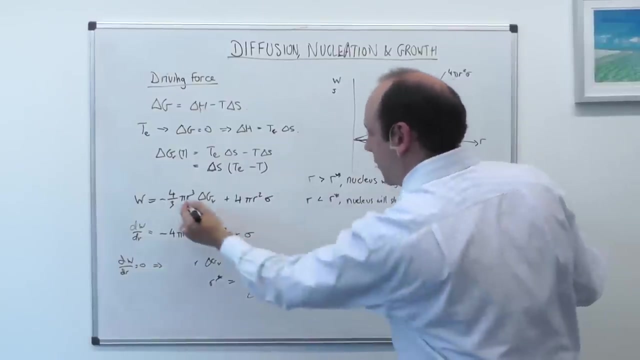 So let's do that over here So we can substitute, substitute subs back into here: W star. call this: w star now is equal to minus four thirds pi r cubed, That's two sigma divided by delta, gv cubed. 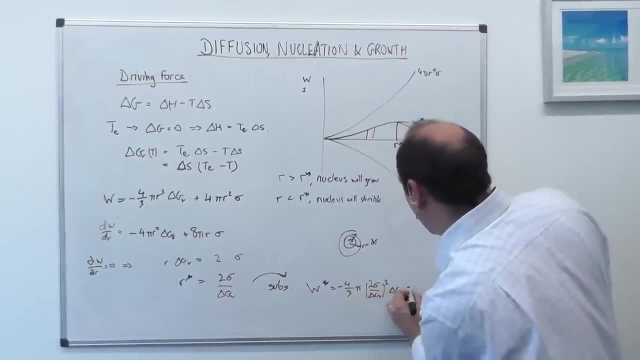 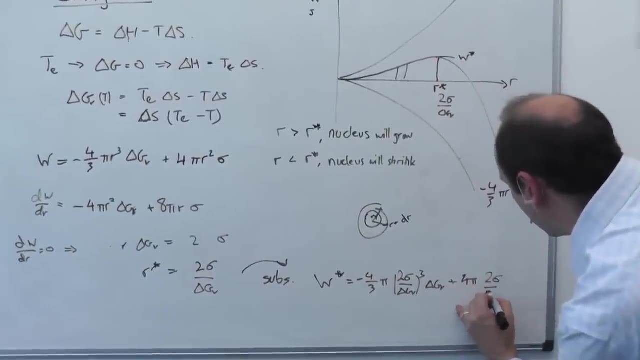 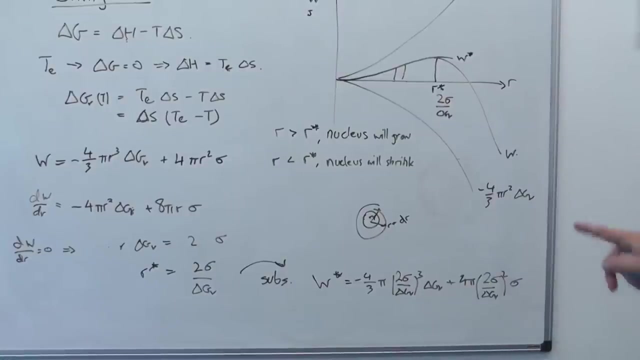 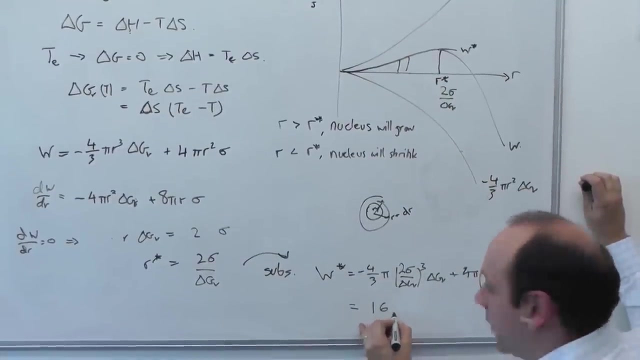 Times delta gv plus eight, sorry four pi, then r squared, So that's two sigma by delta gv squared times sigma, And if you multiply that out then you end up with an answer that's 16 pi by three of sigma cubed. 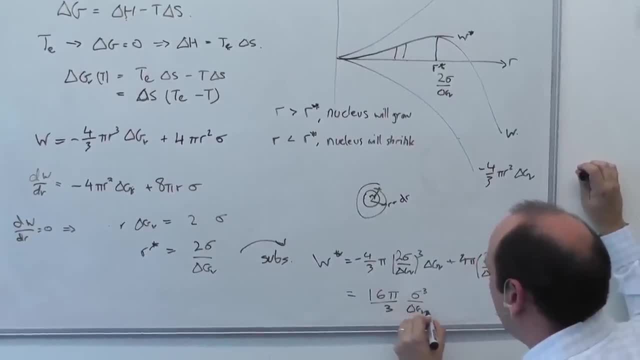 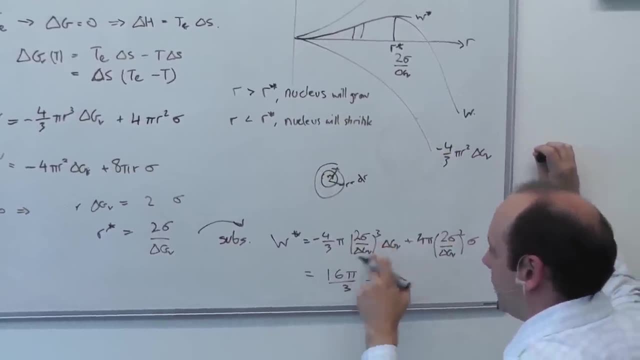 r over delta gv squared Because you see you've got a sigma cubed there. sigma squared, sigma cubed. You've got a delta gv cubed, delta gv. so that's going to be squared on the bottom. This is going to be squared on the bottom. 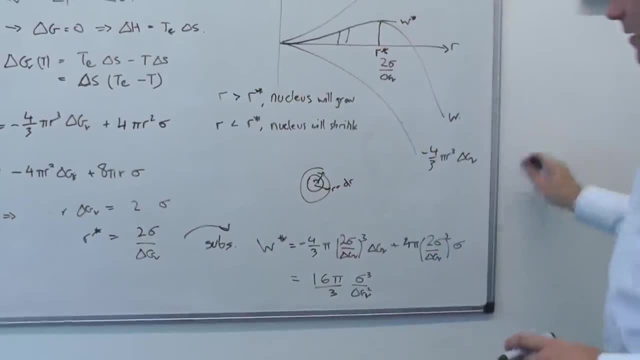 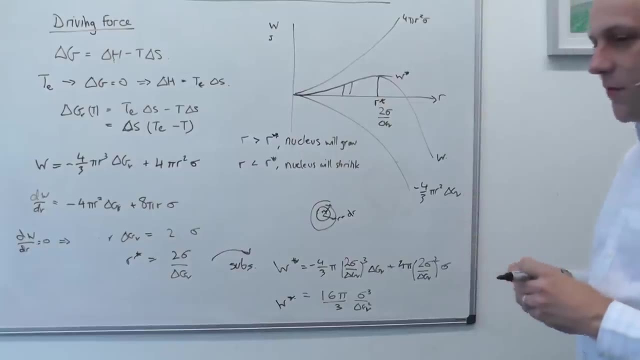 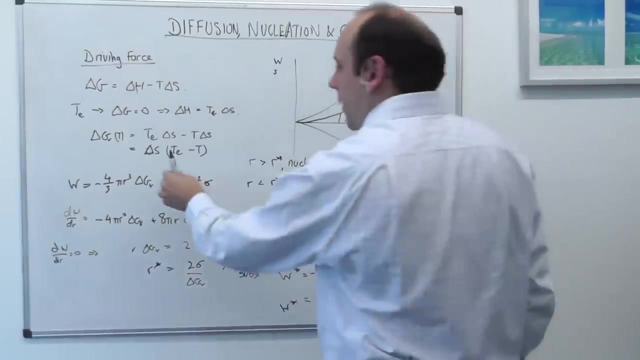 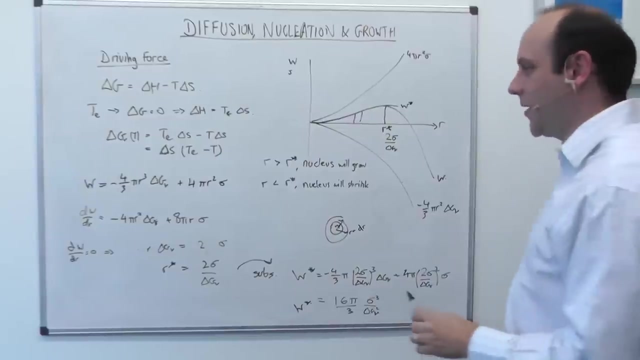 So it all comes out, And so that's our solution for w star. And then we can think about what happens as we change temperature, So as the undercooling becomes very small, as the temperature approaches the transformation temperature, then delta gv here becomes very small. 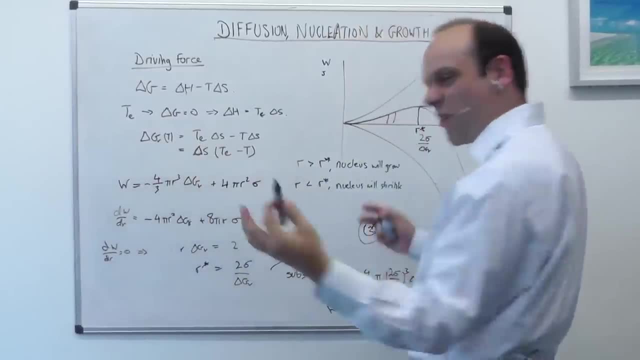 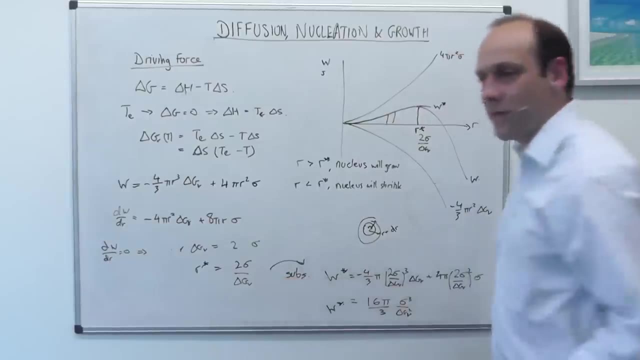 Sorry there. yeah, because this term's becoming very small. We have no driving force And as we go to having no driving force, this work becomes very large and this radius becomes very large. So when we have no driving force, the particle that would grow. 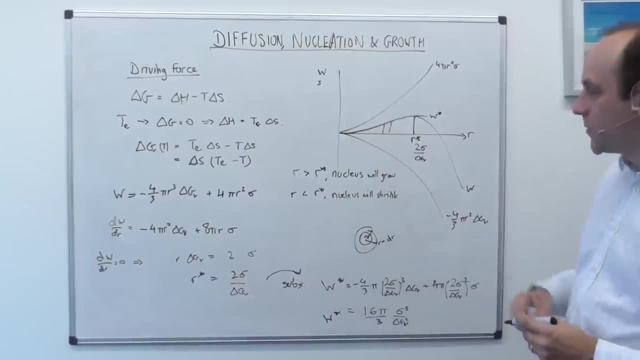 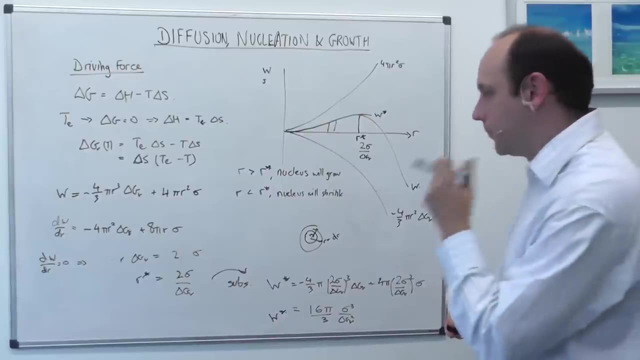 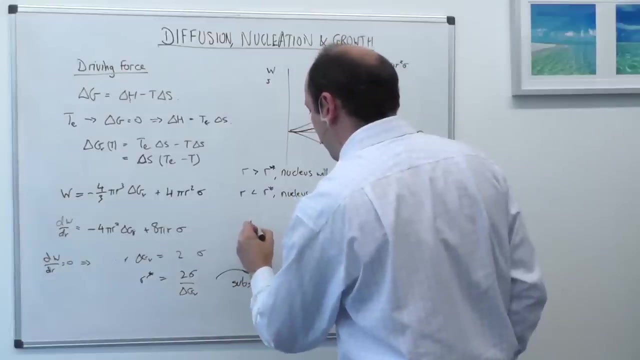 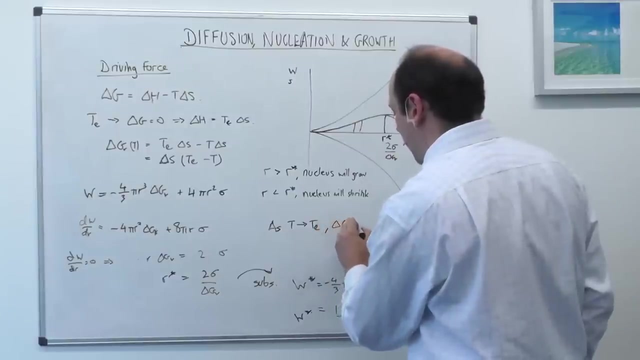 the nucleus that would grow would be enormous. And as we have more and more driving force, smaller and smaller nuclei can come into play. So let me just write that down. So as the temperature tends to the transformation temperature, then delta gv tends to zero. 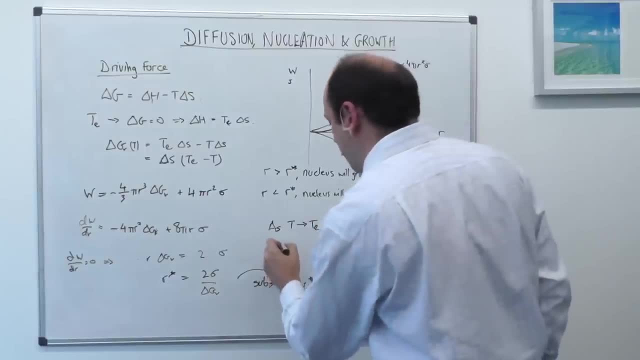 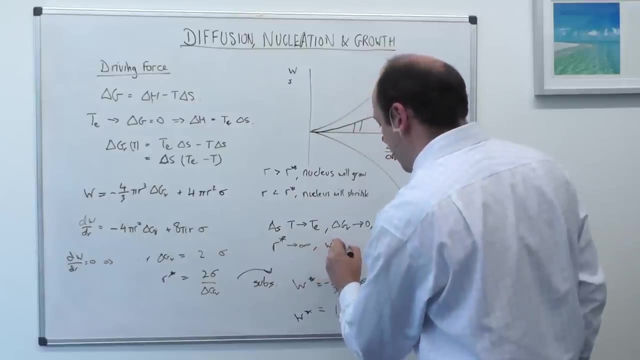 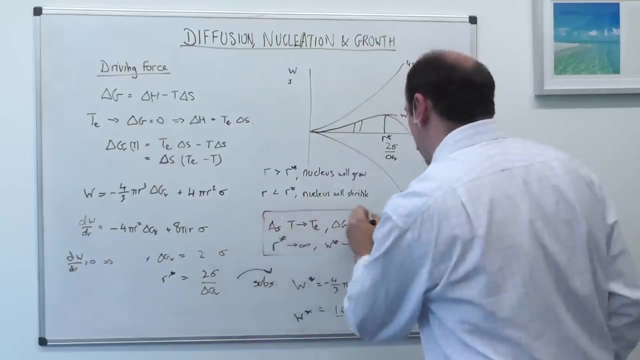 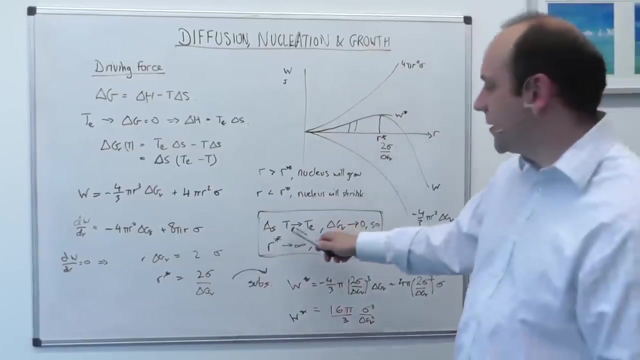 So r star tends to infinity and w star tends to infinity. So what that means- I'm going to tidy that up a bit- What that means is is that as we have less and less driving force, as we're closer and closer to the equilibrium transformation temperature. 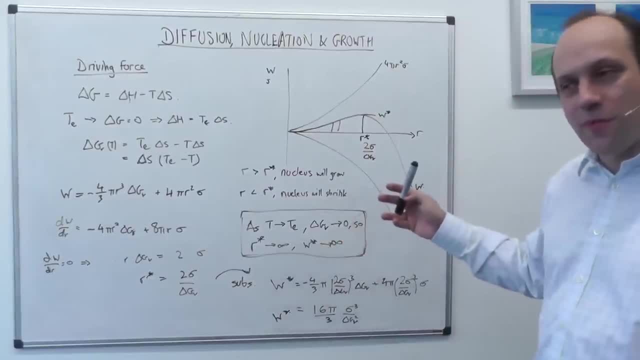 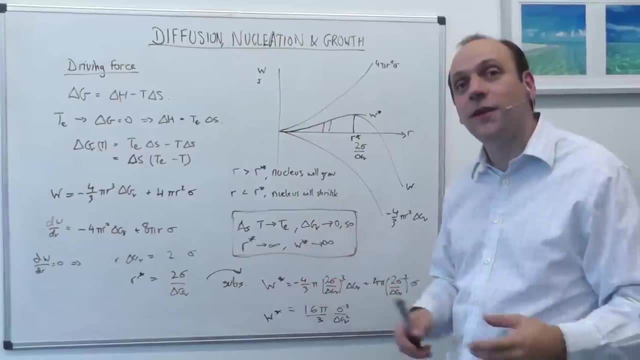 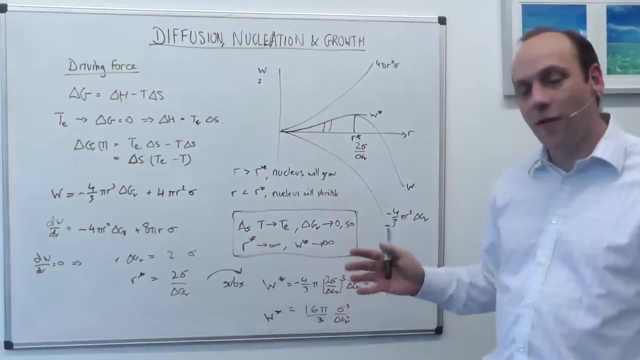 then we need bigger and bigger nuclei to be present, and they won't necessarily be there. So what that means is that at small end of coolings we might not actually see the new phase appear. We need to have some super cooling, some driving force, in order to get whatever nuclei there are there. 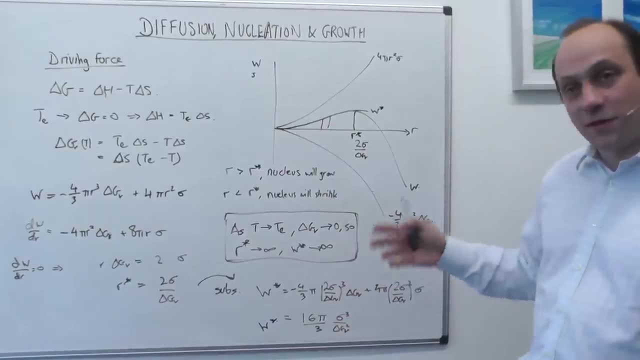 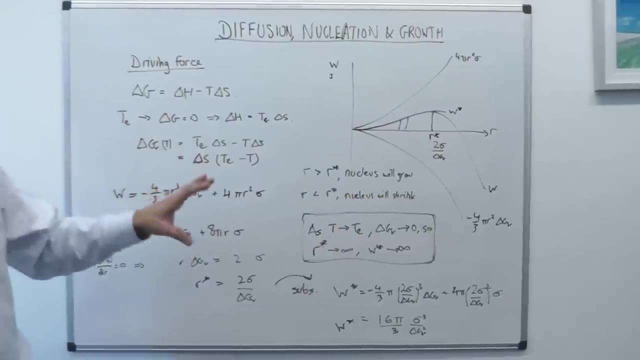 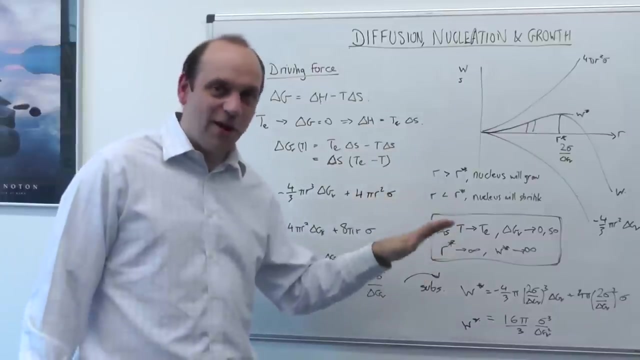 to be able to be effective as nucleation starts to grow new particles. So the other way to look at that is that if we don't have any particles to nucleate from, then we'll find nucleation quite difficult, And if we put some in, then nucleation will become quite easy. 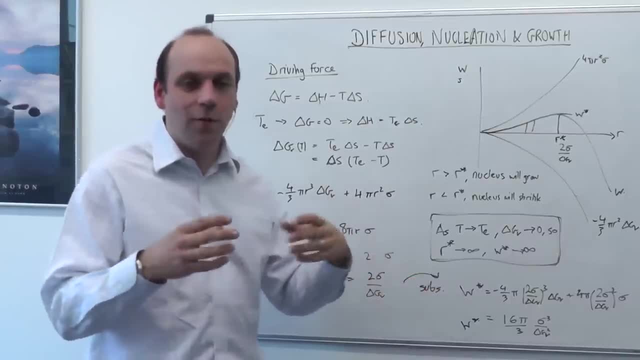 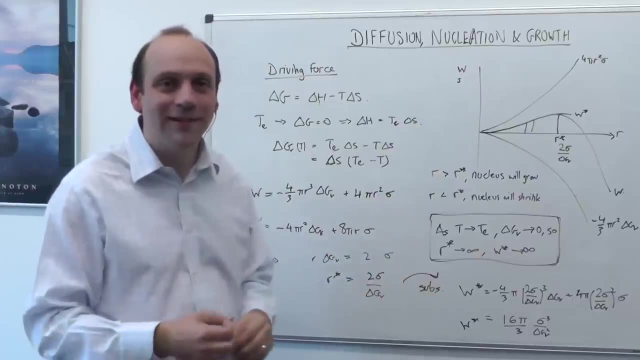 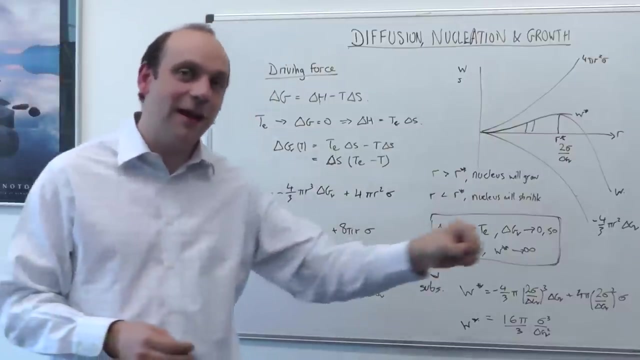 There's two examples of that. One is our example with making ice. It's quite helpful often to put a bit of grit in. basically, You require less super cooling. Another way of another example is when you're welding aluminium alloys. quite often people will sprinkle scandium in. 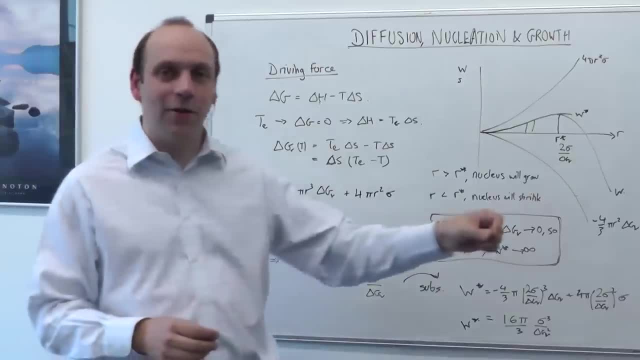 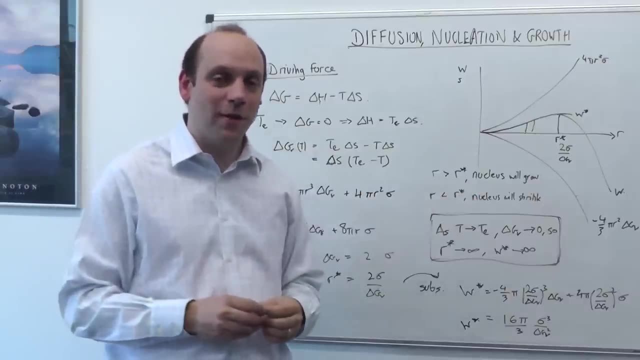 or scandia scandium, Scandium oxide into the alloy, which provides nucleation sites, And that results in a much finer grained microstructure in the aluminium world, because you have more nucleation sites, so you end up with more grains starting growing. 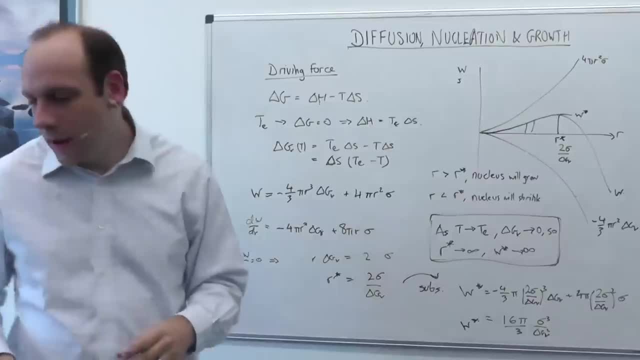 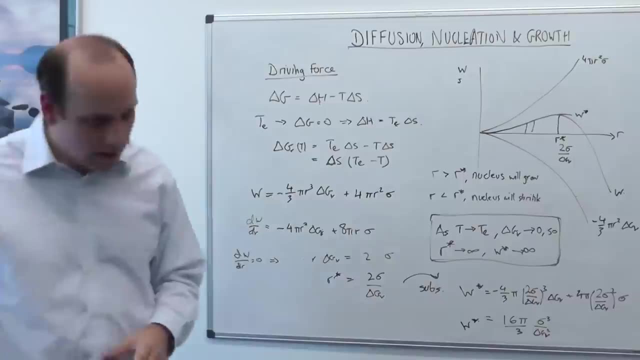 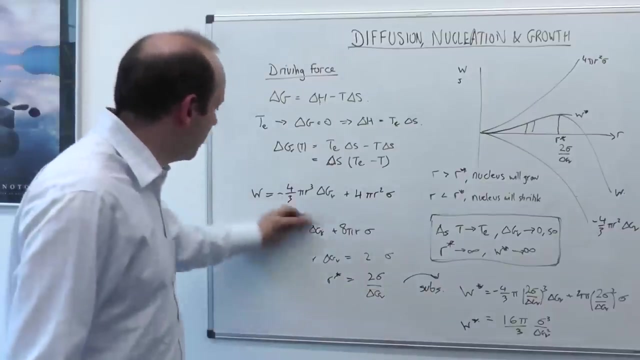 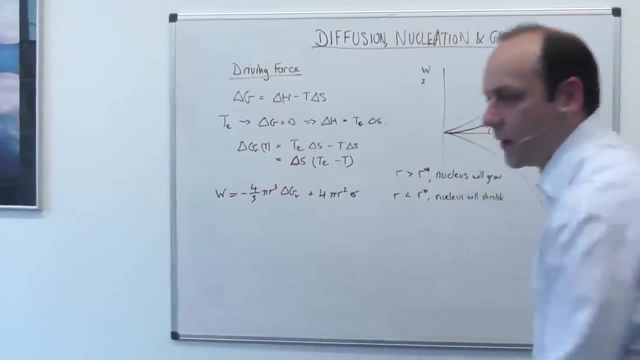 when you first form the solid from the liquid. We can keep on going with this. There's one or two last little things to say, So I'll just rub This stuff out. We can also imagine that when we precipitate out our particle, 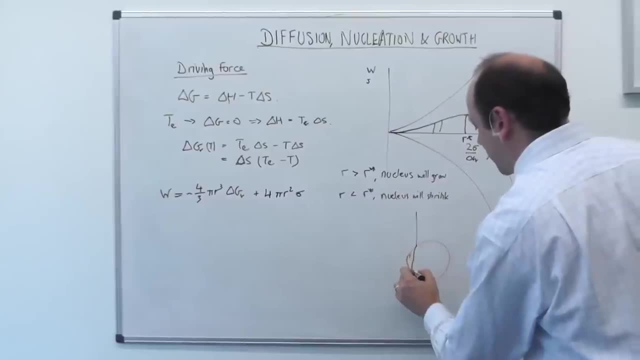 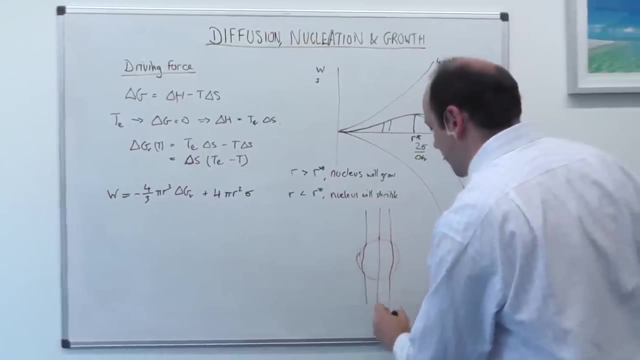 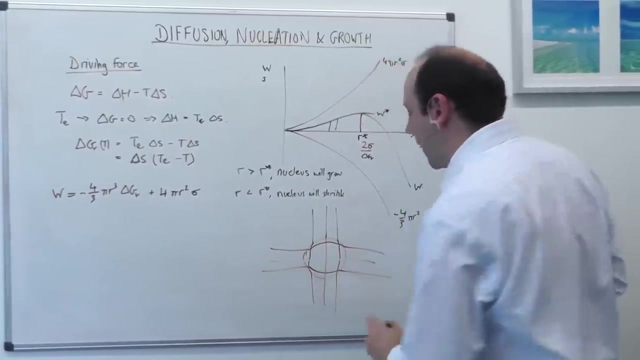 what it might do is it might stretch the atomic lattice around it. It might have a larger lattice parameter than that of the surrounding lattice. So imagine different lines in the material would be pushed out As they went through it. So those who imagine different planes, and they've been stretched out by this new particle that has a bigger lattice parameter. 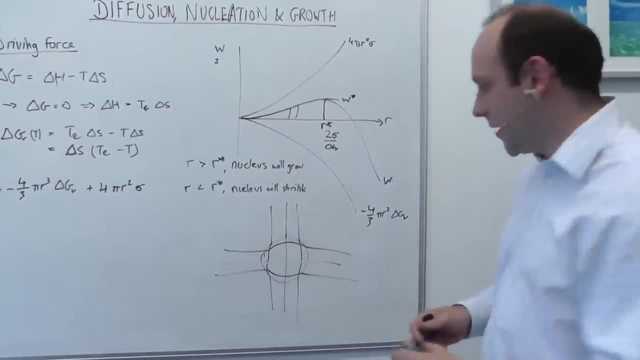 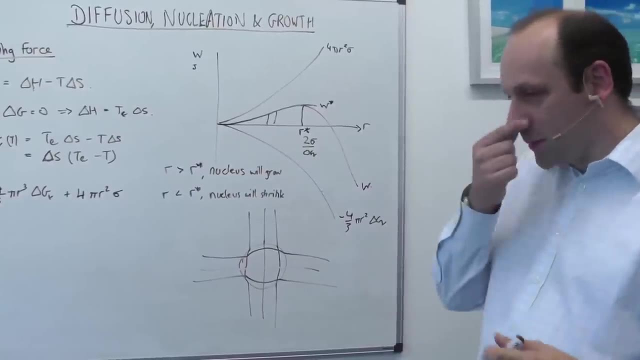 And there would be a strain in the surrounding material associated with that. There'd actually be a bit. this strain field would extend slightly beyond the particle And that would then be another term that we could put in. That's a term per unit volume for the sake of argument. 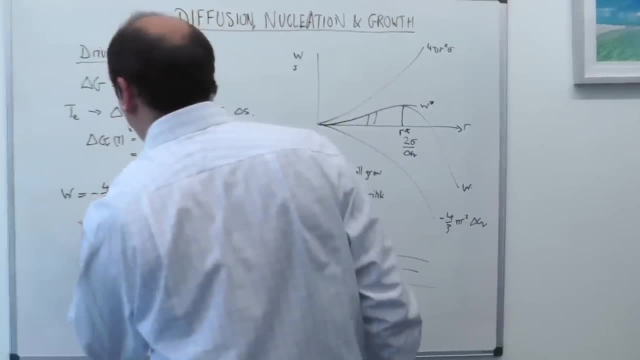 And so we could put that in as being a minus four thirds pi r cubed- And that's a term per unit volume for the sake of argument, And so we could put that in as being a minus four thirds pi r cubed. 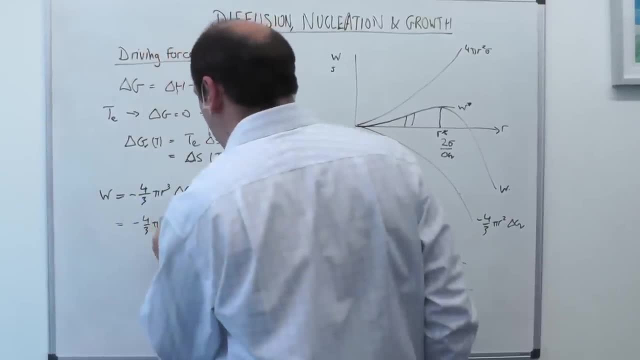 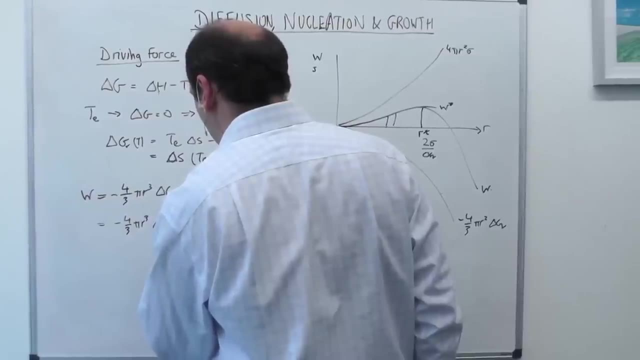 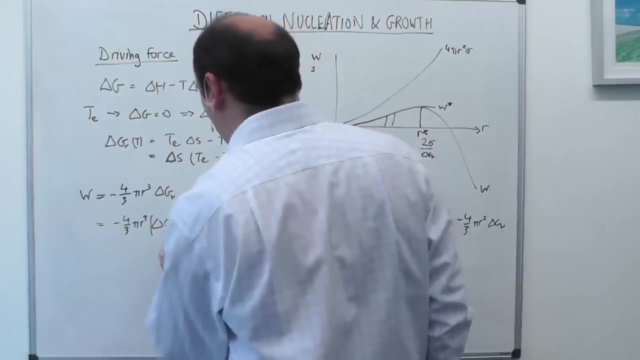 And so we'd put that in as being a minus four thirds pi r cubed Times, the Delta GV minus CK Gamma squared. And we explain what those terms are in a second Four pi R squared Sigma. And here, if we say that the strain is proportional to the composition, 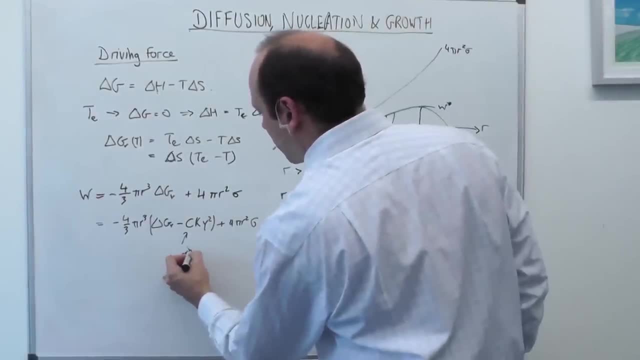 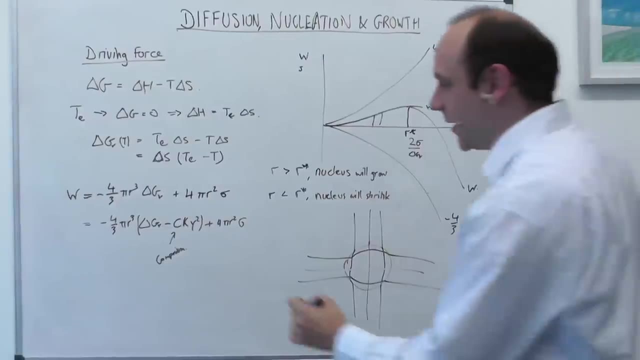 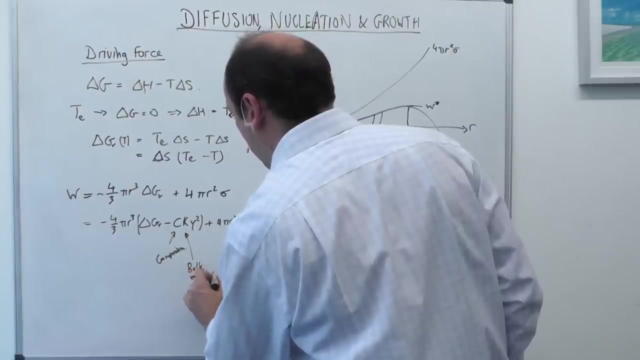 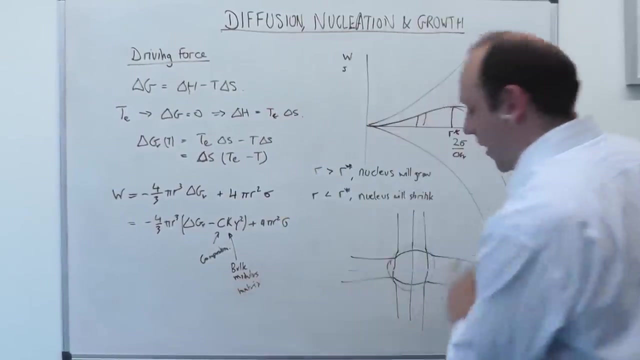 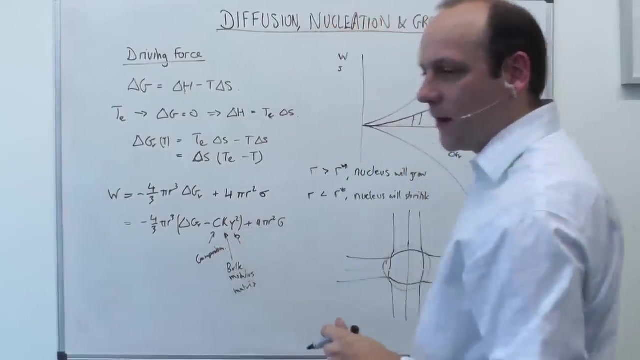 So that's the composition or the composition difference. in fact, particle k is a stiffness constant. k is actually the bulk modulus of your matrix material of the matrix, sorry, that is, of the material around the particle particles nucleating into and gamma. here is then a final term that's to do with the surface. 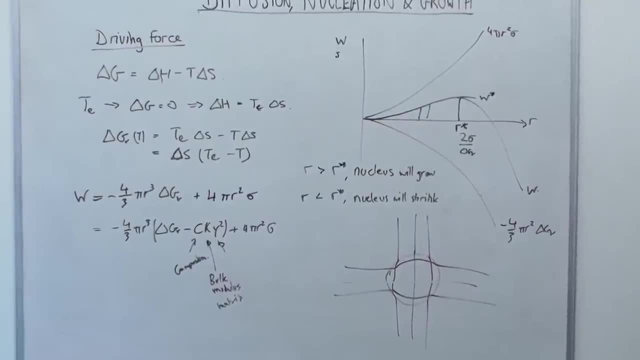 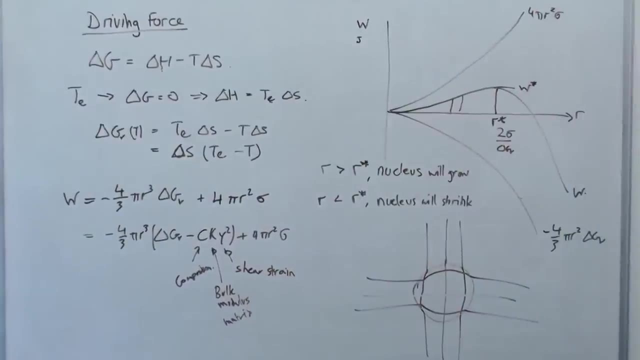 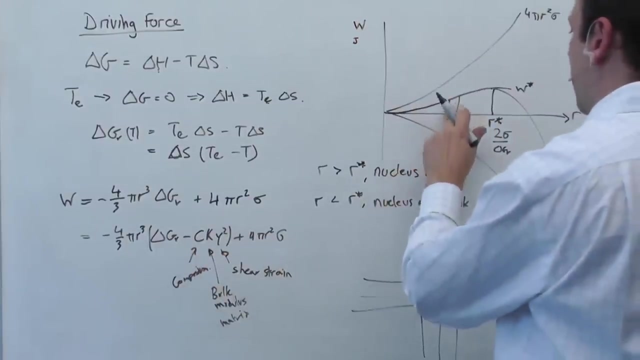 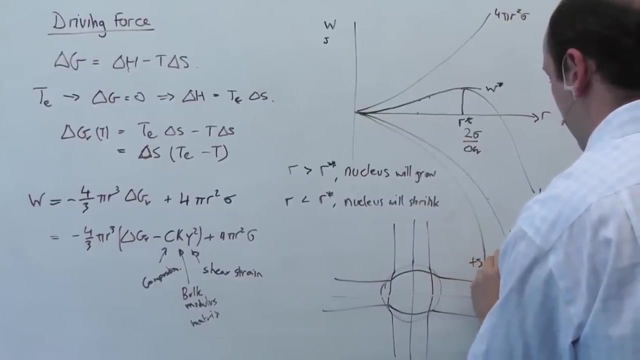 um, i think no, it's a shear strain. it's a shear strain, it's an intrinsic shear strain, um, but it goes per unit volume, and what that means is is that, uh, you actually have an additional penalty. so what this will do is it will lower this down. so that's plus strain here, plus the. 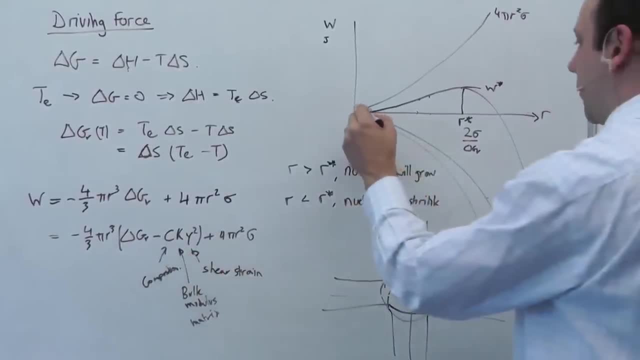 effect of strain, because it's adding on to this cube term and so it will lower this down and it's actually going to work with the beam gene structure plus the effect of strain, and so what that name means is that you actually have an additional penalty. you. 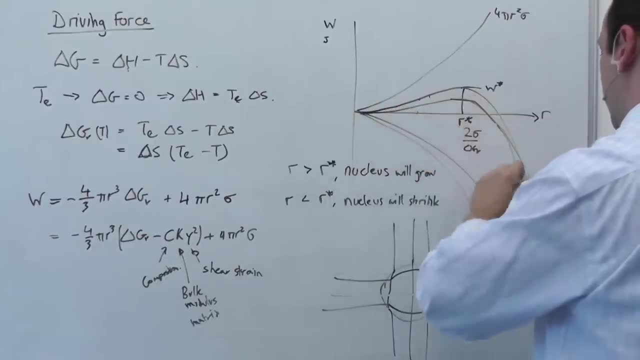 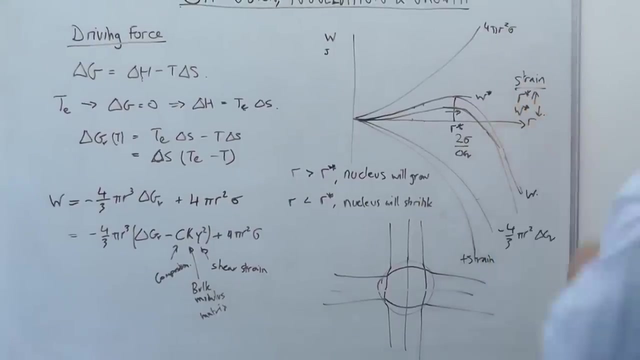 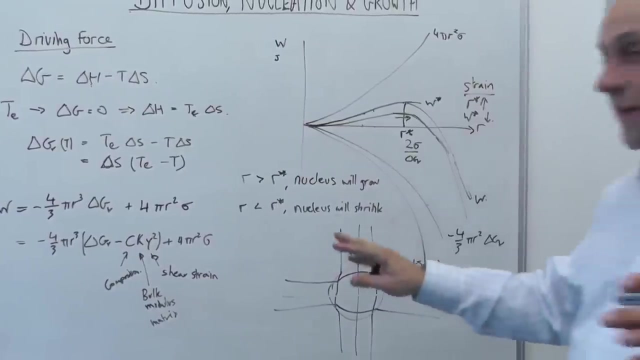 down here. so it's going to push R star bigger and push W star down, So that effective strain will be to make R star goes up and W star goes down, And that will be another thing that makes nucleation harder. So this shear strain you would need to have then some super. 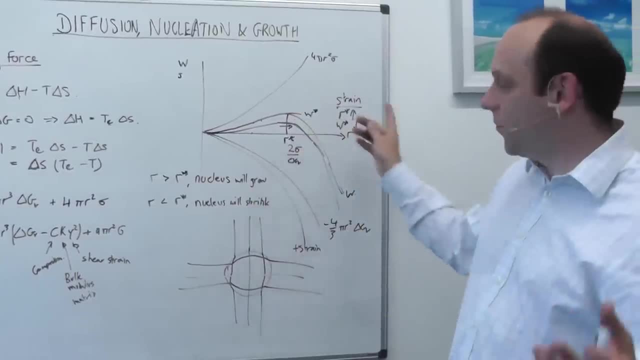 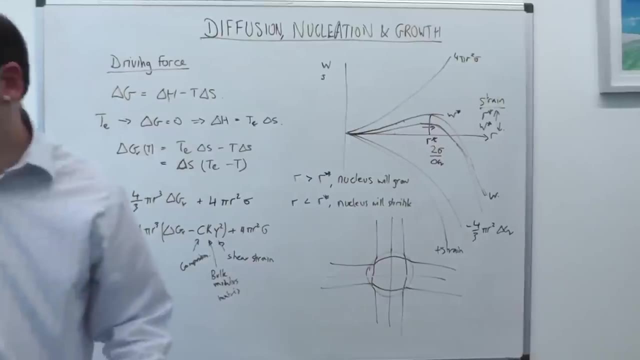 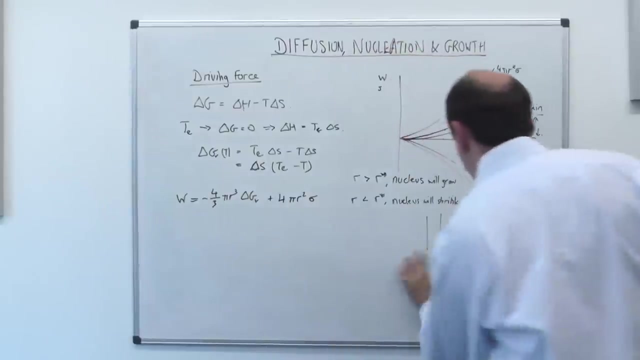 cooling to be able to nucleate at all, even from a very small particle. So that's the effect of strain. So what does this all mean? What does this all mean? A few headlines. Let's in fact get rid of the maths. It's now a distraction. 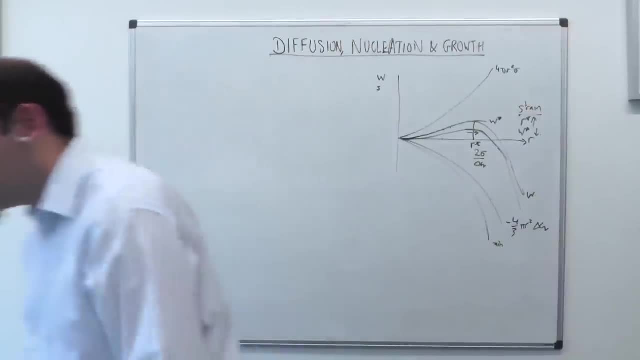 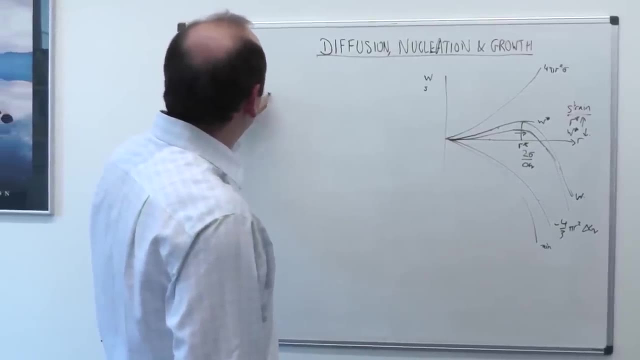 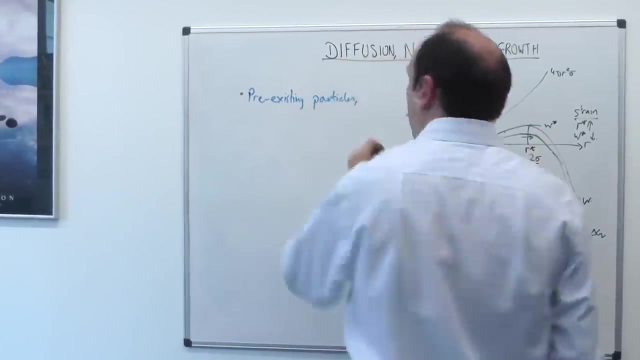 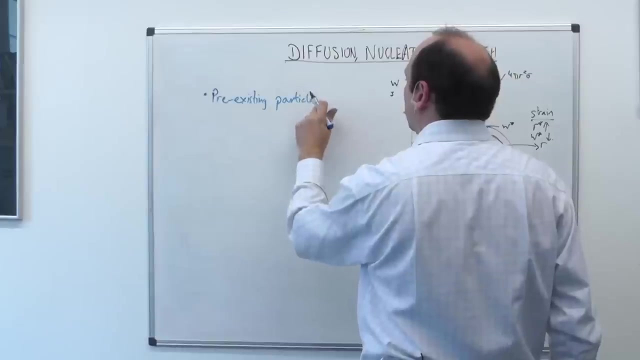 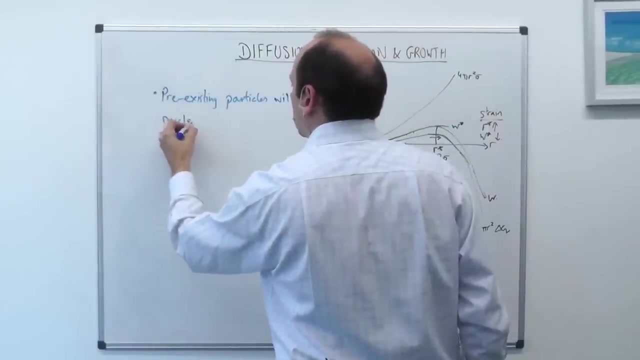 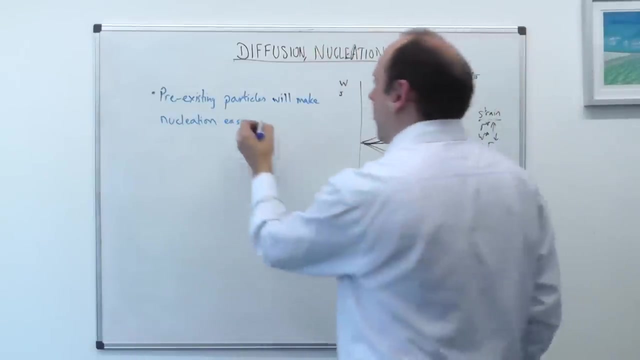 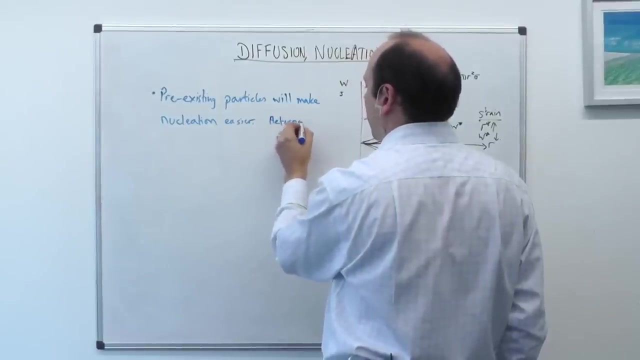 And this means a couple of things. Generally, having pre-existing particles, some things that already exist that you could just grow on, will make nucleation easier. So what does this all mean? And that's called heterogeneous. hetero- it's Greek genius, So there's an additional. 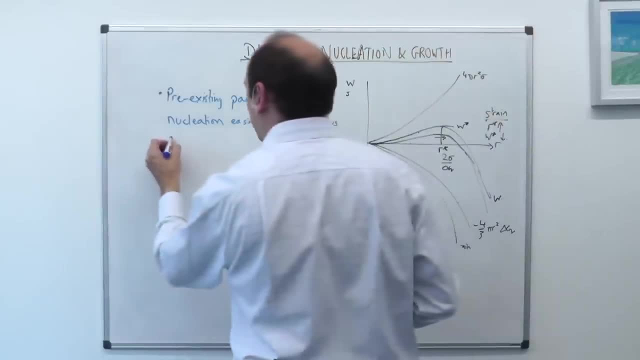 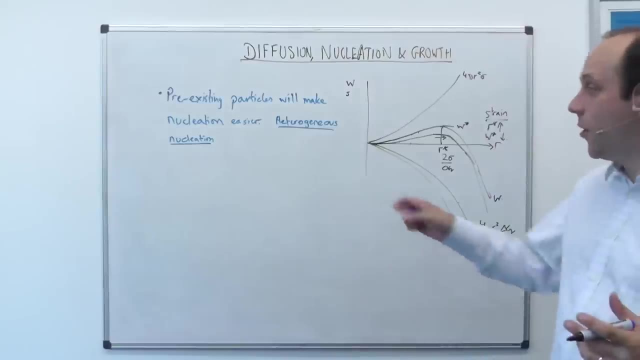 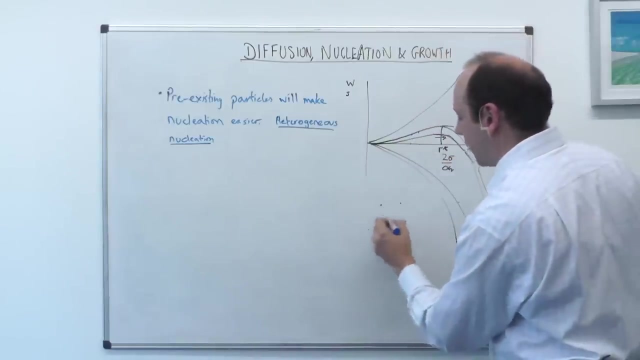 E there. Heterogeneous nucleation is the name for that phenomena. So that's when you nucleate off of some things that aren't homogenous, that are distributed, that have a distribution. So if there are some flecks of stuff in your material in 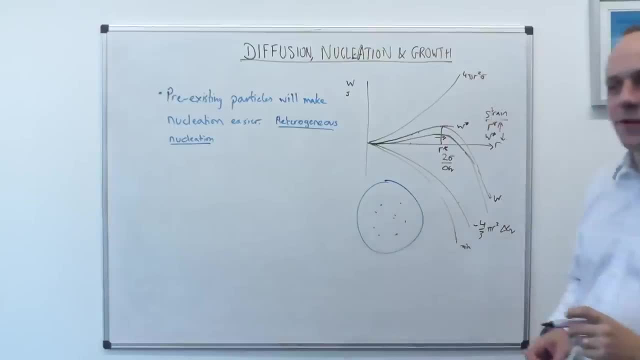 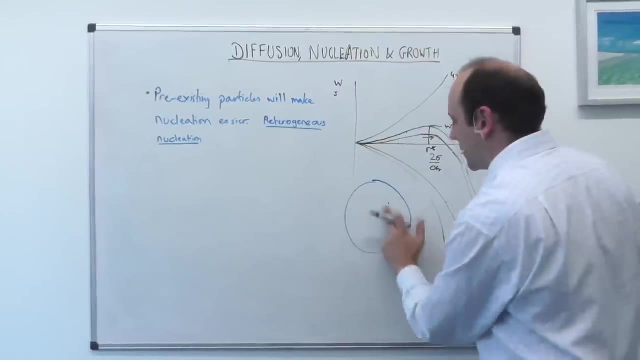 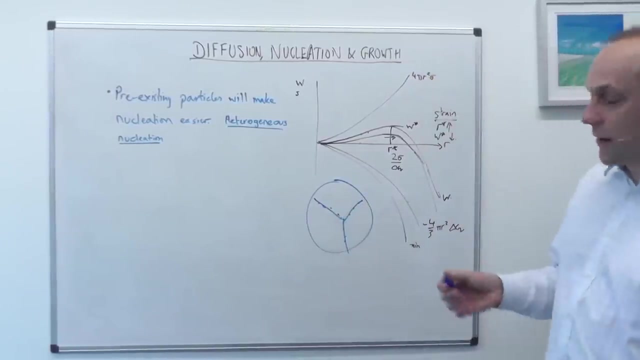 your alpha grain. if you have some particles to nucleate from, then those pre-existing particles will make nucleation easier. which is why we said back at the start that if we had three alpha grains, then those heterogeneous nucleation sites will be good places to nucleate. 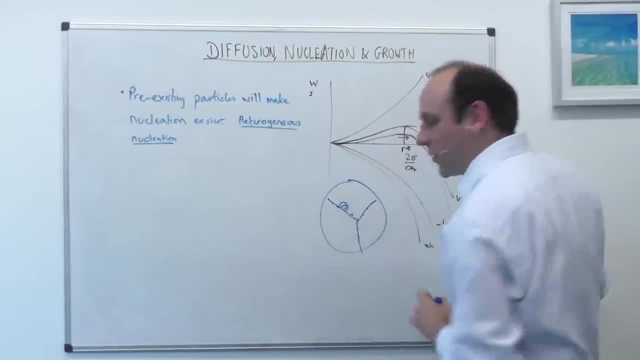 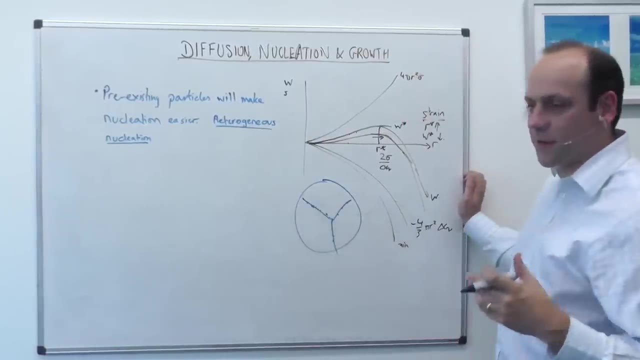 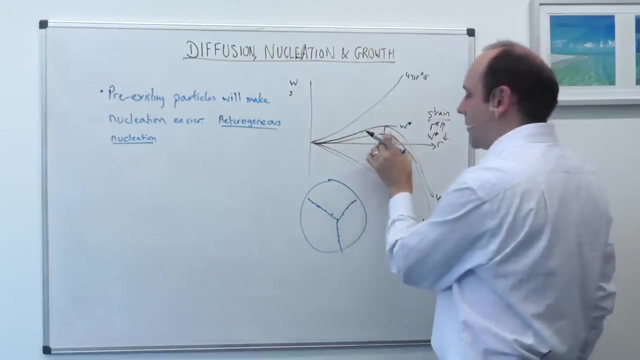 new phase, Then we'd be in a slightly different situation. We'd be growing something like a cap, a circle cap or something like that. So that's called heterogeneous nucleation, And what the effect of that is is that those will come into play once our star declines to the point that it's smaller than the heterogeneous. 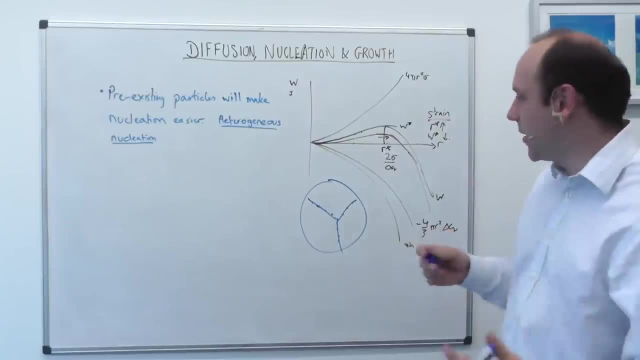 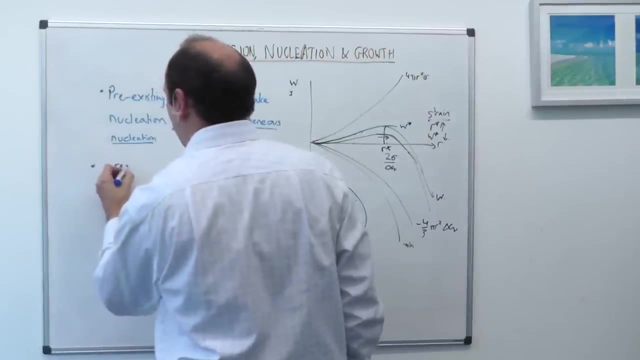 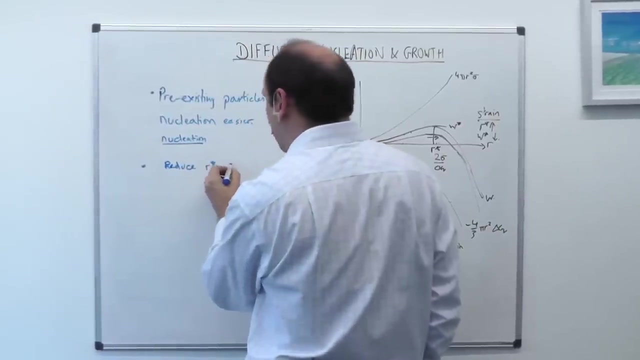 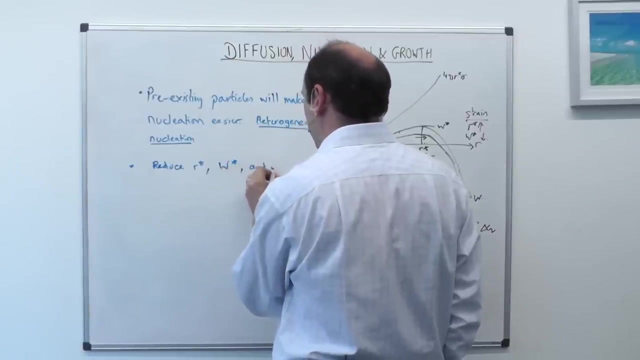 nucleation sites. So the other way to look at it is that it's sort of an alternative way of thinking about the same thing, Which is that they will reduce. there'll be a pre-existing volume, so they will have to reduce r star and w star, And so and we'll have an Oxford comma, and so we'll reduce. 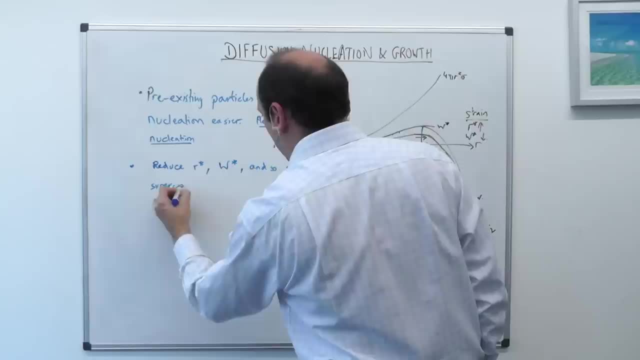 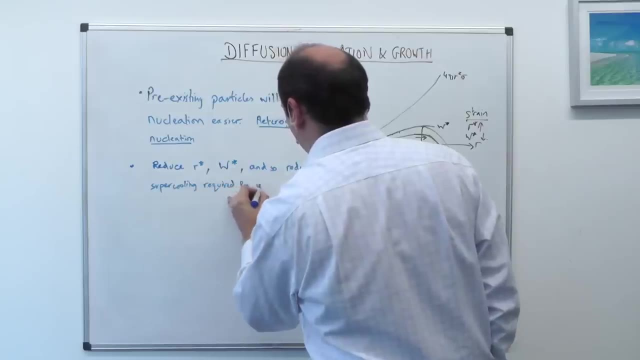 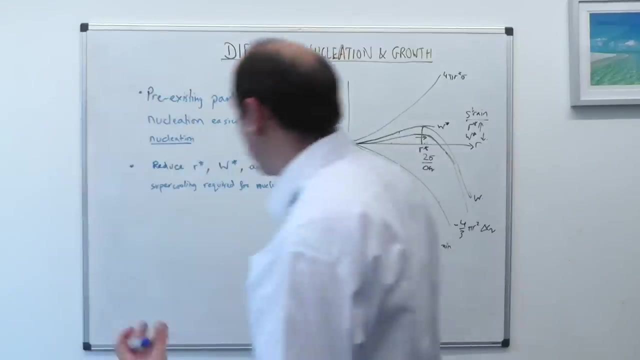 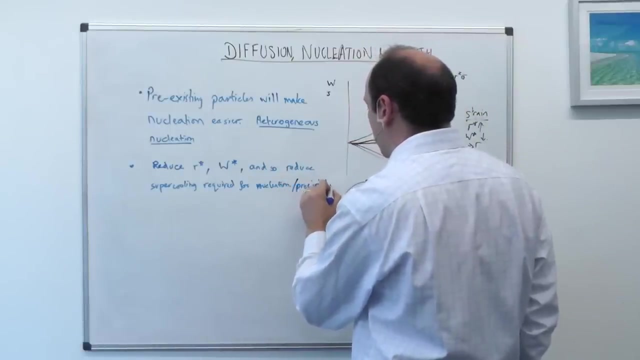 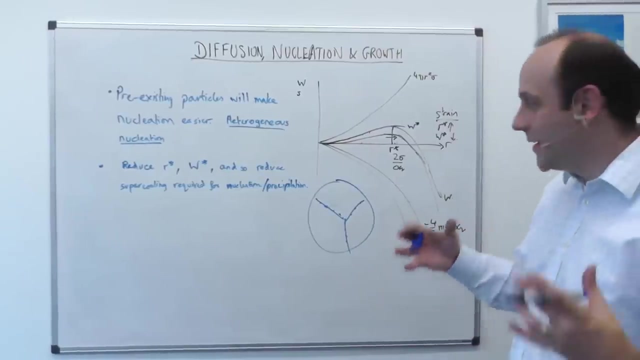 the super cooling or under cooling required for nucleation to occur- okay, or for precipitation to occur, and the other side of this is that homogenous nucleation, that is, nucleation off of no pre-existing sites, is something that's very difficult. so our observation then would be: 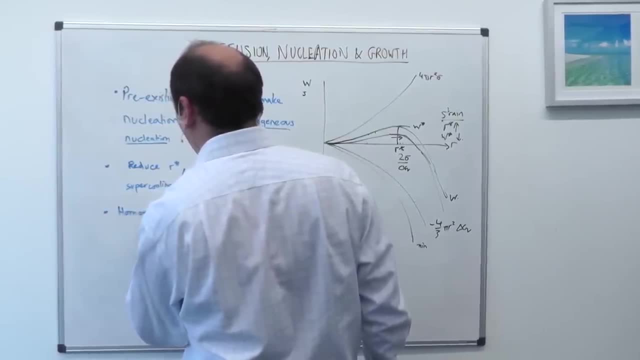 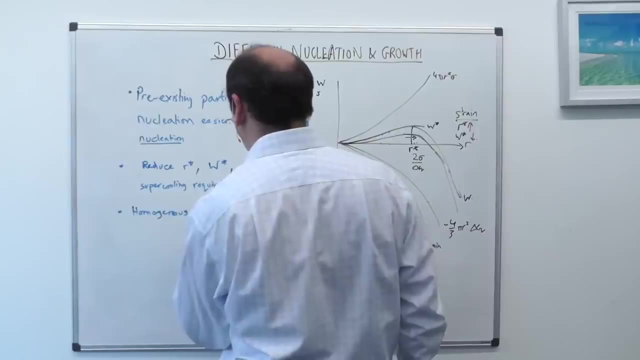 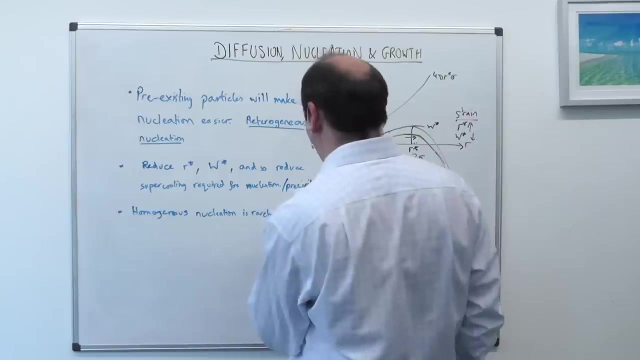 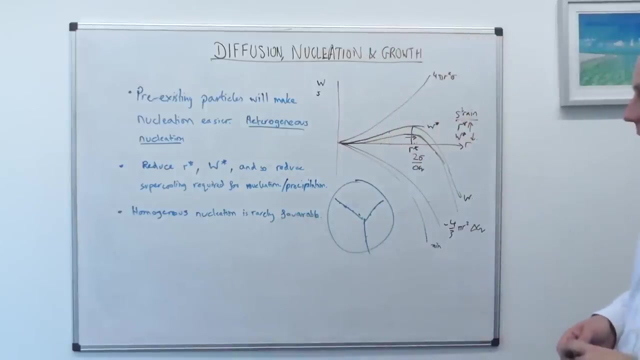 that, because of this thermodynamic argument, homogenous or homogeneous nucleation is rarely favorable. it rarely happens and we'll be. we'll be british about this and have favor with an our rather than american. so if we think of an example of this, um, there's an example actually, in aluminium alloys and aluminium copper alloys. 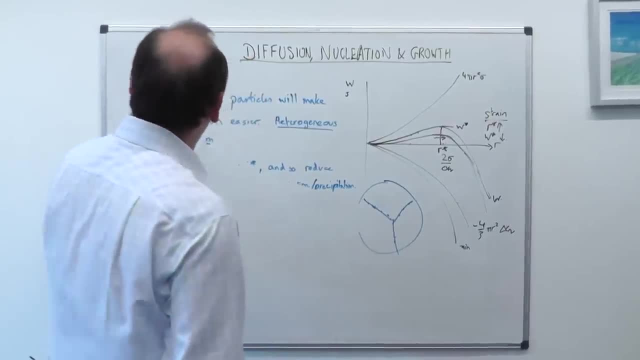 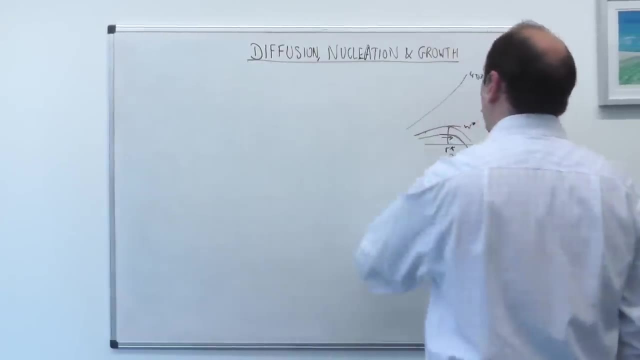 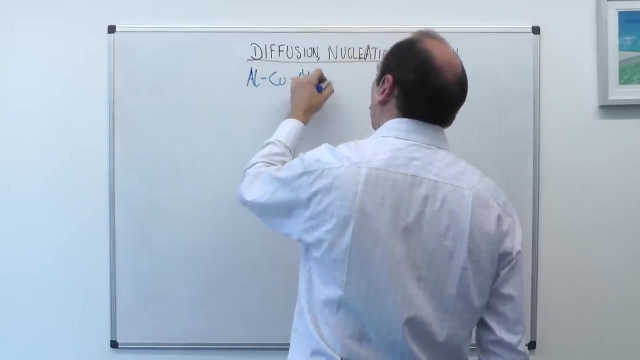 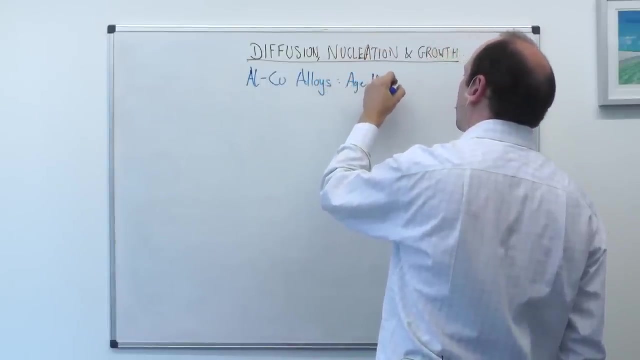 um, and that's going to be where we'll we'll end this segment. let's think about this example: um. so in aluminium alloys, what you observe, or aluminium copper alloys, so these are alcu alloys, um, and this is an example of an aluminium copper alloy- and they're age hardening, how they precipitate out particles that strengthen them. that. 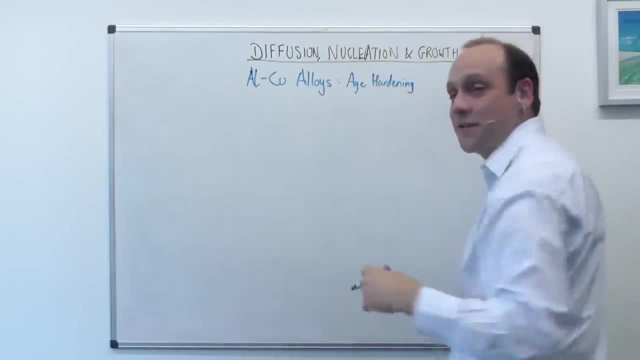 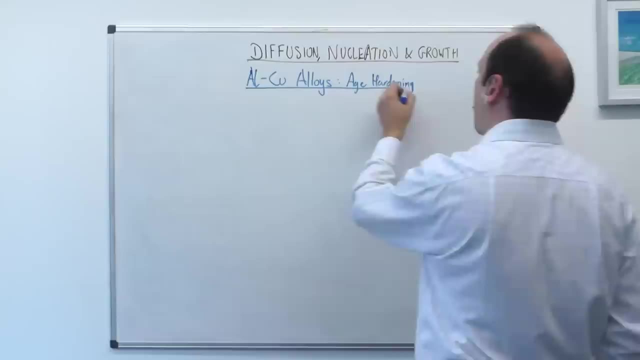 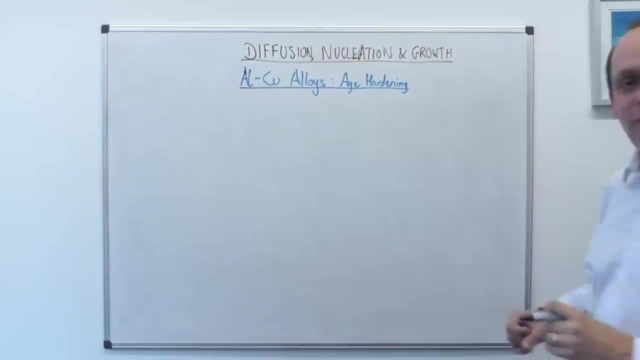 make them harder as you age it, as you put, give it time at temperature. so time at some temperatures are like 200 or 300 degrees c and what you find is that the first precipitates you form so you're in a big aluminium enriched copper grain. then say: you're in that grain. 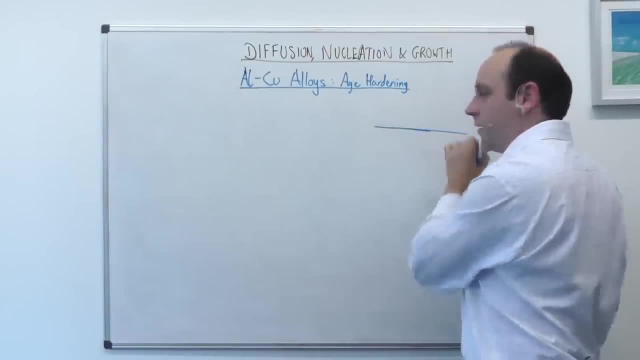 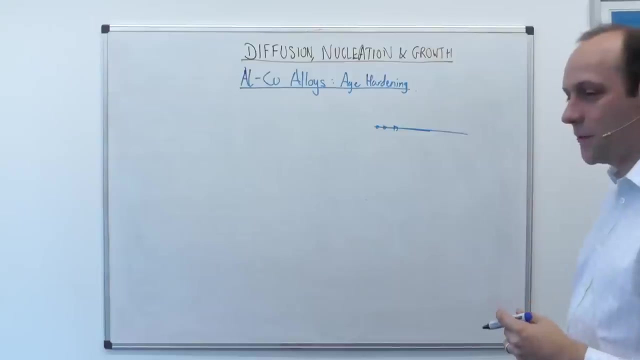 then what you form first is a tiny little disk, one or two atomic layers thick, of the same composition, um, and- uh sorry, not the same composition- of alternating areas of aluminium and copper, which is called a gp zone. um, and, if you look at the phase diagram, the gp zone. 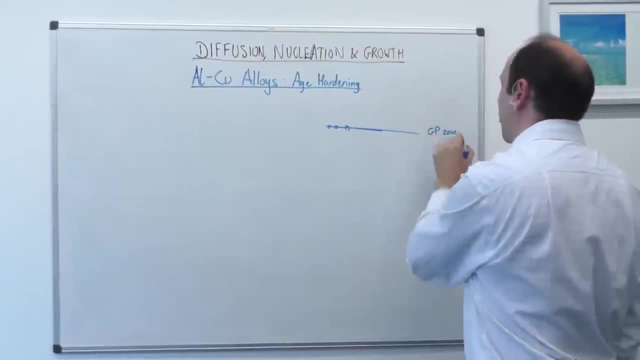 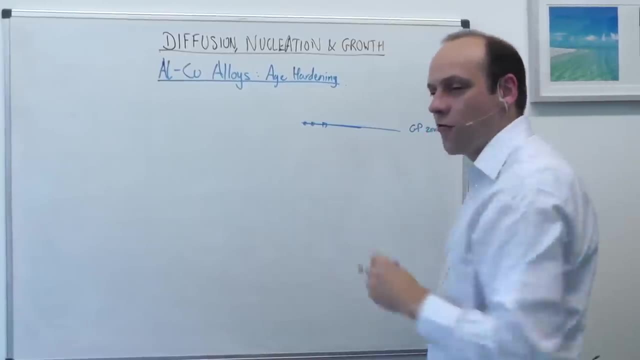 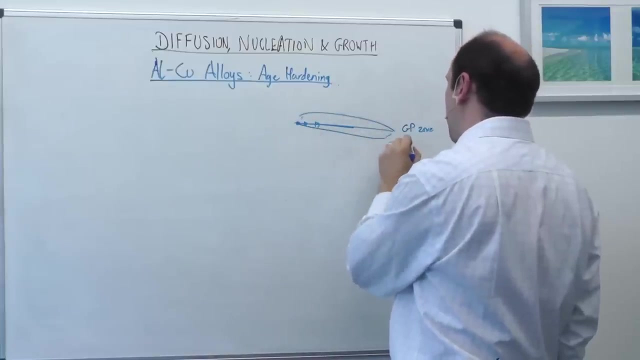 doesn't appear on the phase diagram, um and uh. it then acts as a nucleation site that you can grow another precipitate on, which is called, and so it gets consumed, which is called a theta double prime precipitate, and that also isn't on the phase diagram. it's not the stable phase. 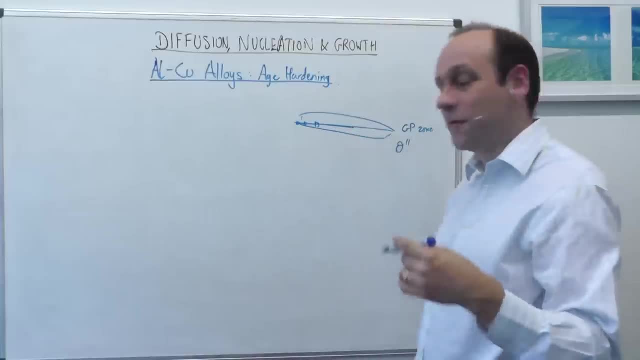 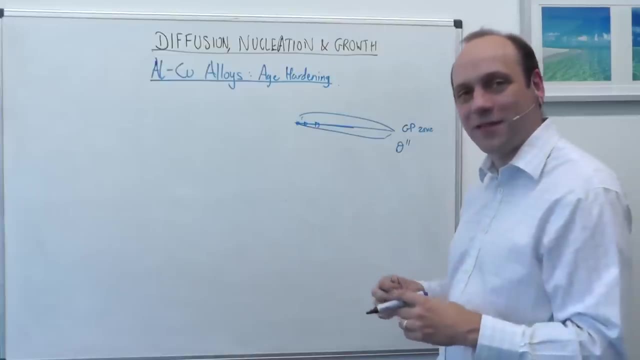 then. but it's this. theta double prime is still uh, cubic, it's still the same crystal structure. it's still the same crystal structure. it's still the same. it has a low surface energy. um, therefore, because it's sharing the crystal structure and it's got a. 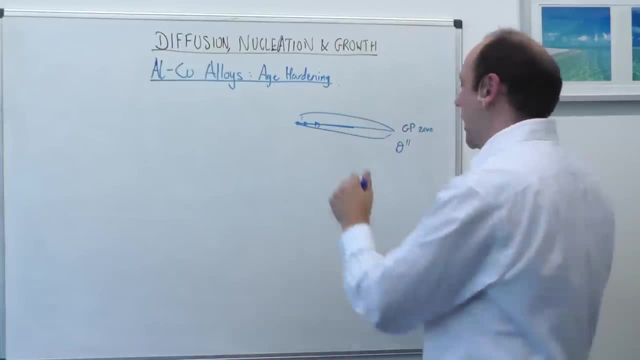 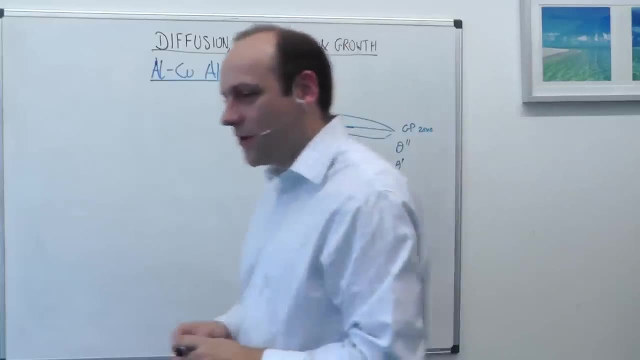 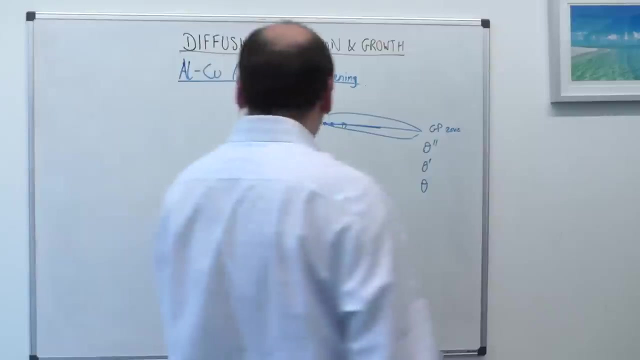 similar composition, um to the alloy um, and then we go through another one until we finally get to our final theta precipitate. so if you look at the phase diagram, what you see, or look at the energy curves, in fact, if you've got um, your gibbs- energy against composition. so we go from. 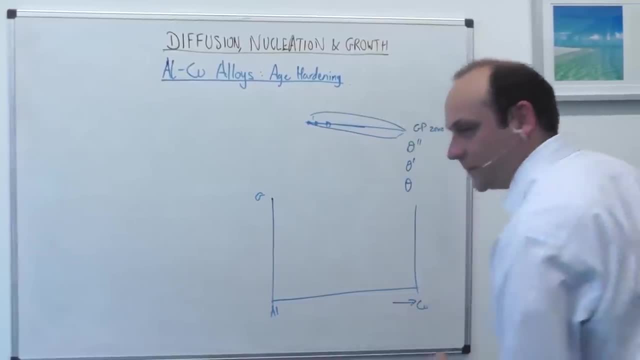 aluminum to copper. you've got um your gypsum energy against composition, so we go from aluminium to copper. you've got um your gypsum energy against composition, so we go from aluminium to copper and it's increasing copper content over here. then we've got our alpha aluminium doing something like: 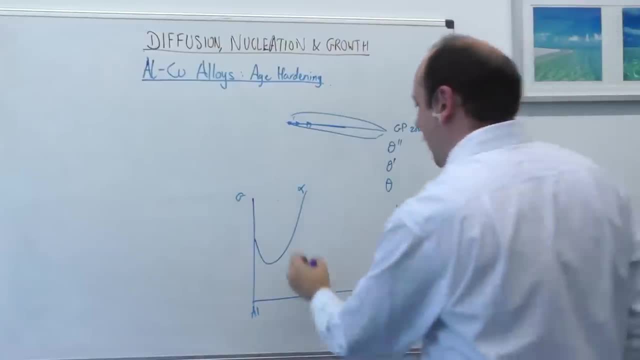 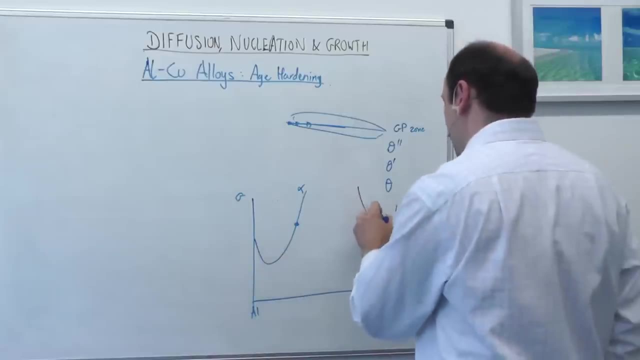 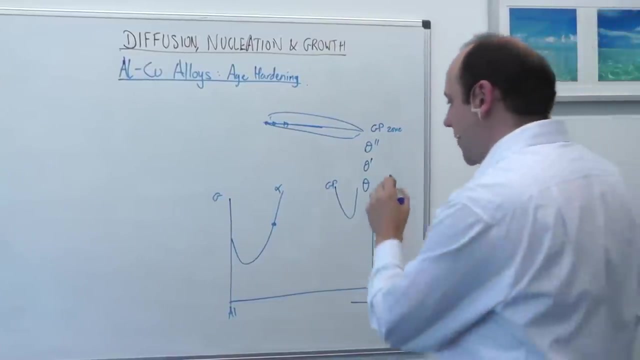 that, yeah, and say we're in an alloy, at our temperature, at our aging temperature, which has a gibbs energy there. well, the first thing to happen is it forms a gp zone with an energy, with a composition over here and then, and so it can lower its energy by forming a tie line like that. 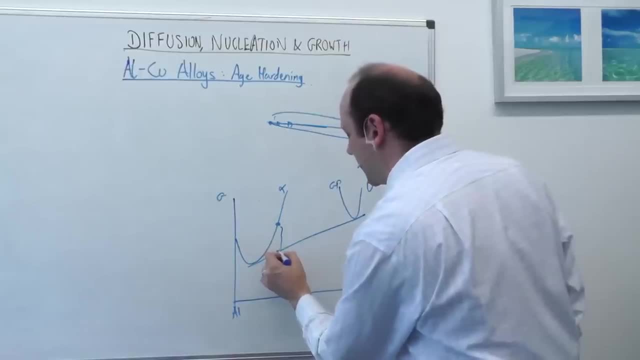 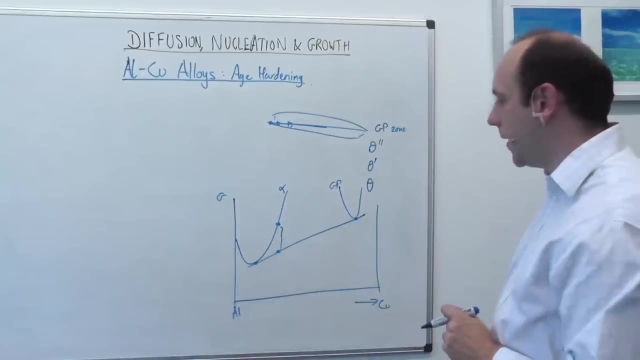 and that lowers the overall energy by this amount, to give you an overall energy there composed of alpha of this composition and gp zone of that composition, and then what can happen? and this is quite favorable, this doesn't require, because you don't have a lot of surface energy for the gp zone. 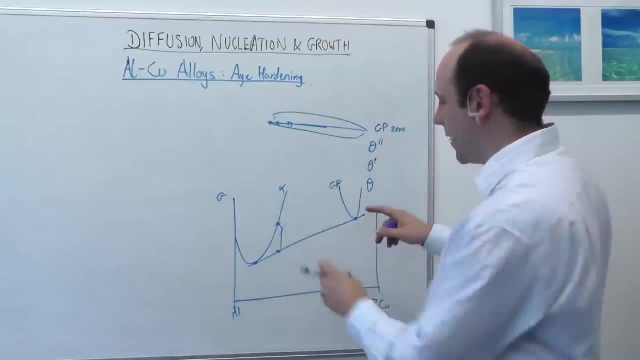 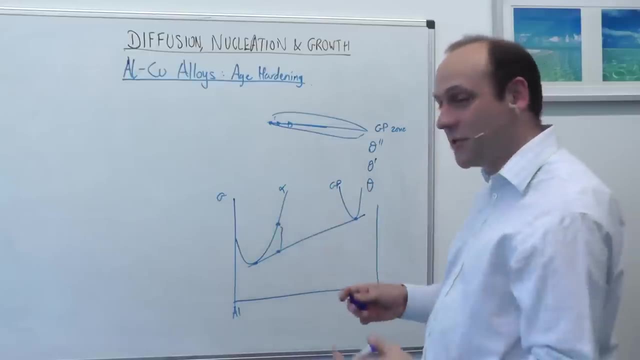 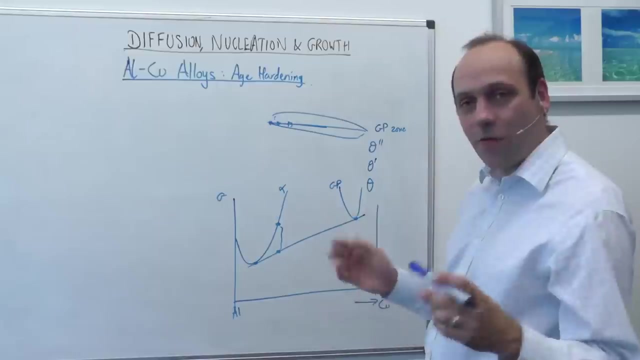 it's only two atoms thick and it has the same sort of crystal structure as the alpha, so this doesn't have a very big sigma, a very big surface energy that penalizes nucleation. so this happens at very low under coolings and can happen off of small little lattice defects, interstitials or whatever. 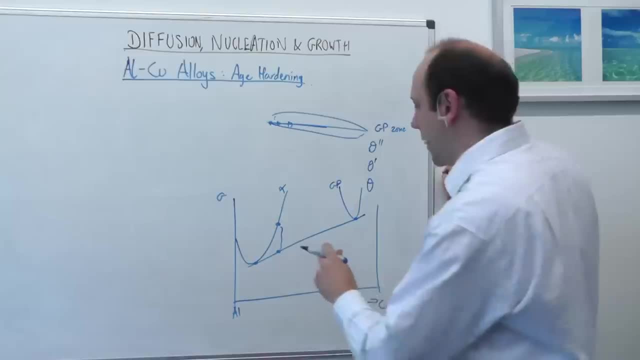 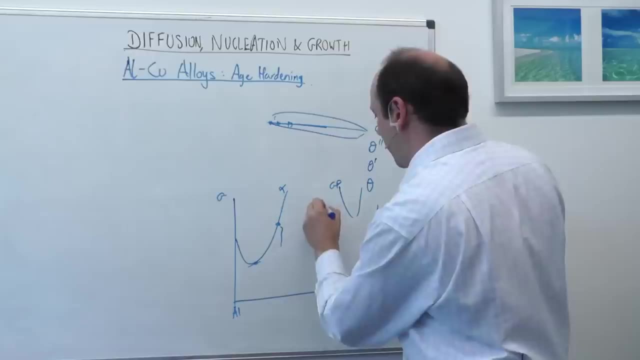 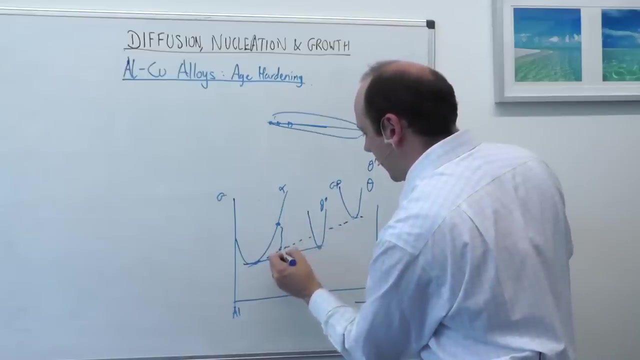 vacancies. and then what happens is actually, you then form a theta double prime and that's closer in composition to the final theta phase. and then what happens is the gp zone gets, gets. so we went from, we went from being here and the gp zone gets consumed and the alpha composition 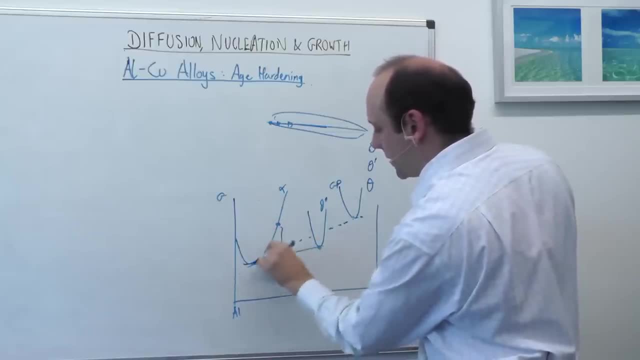 here will move to being slightly pure actually, because you're going down this gradient in the tie line and you get another bit of energy and forming theta double prime here and alpha, which of its composition slightly changing. so then you get actually quite a lot more theta double. 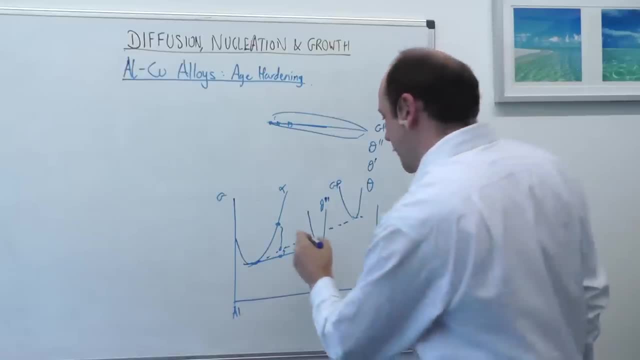 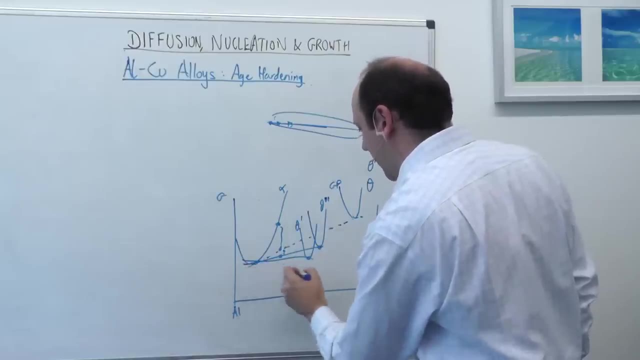 prime forming as well, the volume fraction goes up and then there's a theta prime and you get another tie line, and then there's your final theta phase over here and you get another tie line, and at each step you get some gives energy. this is for composition c. 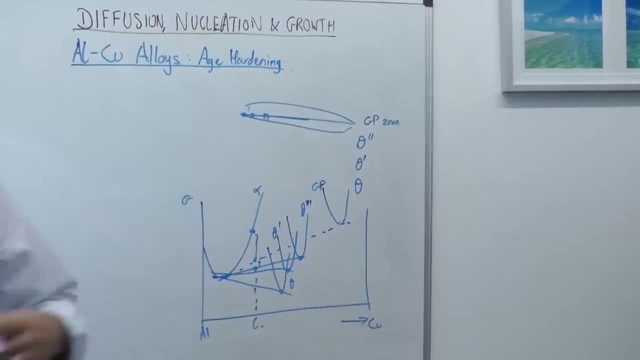 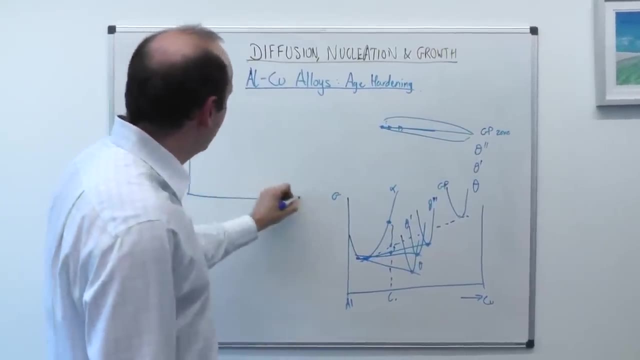 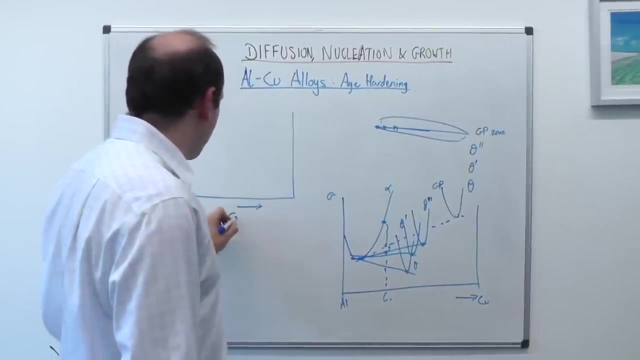 um, so that's sort of the what it looks like on a uh, on your gives energy curves. so what that means is is the phase diagram will look like this: so this is temperature against composition. um, so this is aluminium and this is increasing amount of copper. um, in i know, weight percent, atomic percent, whatever. 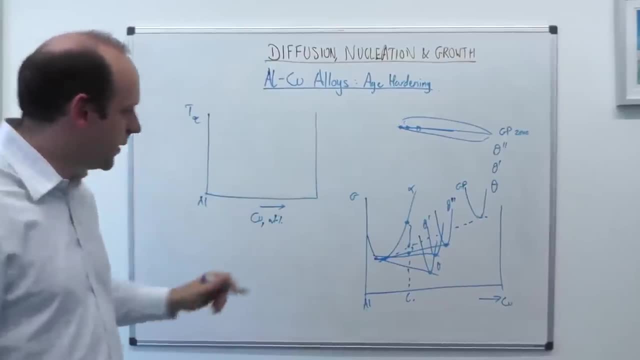 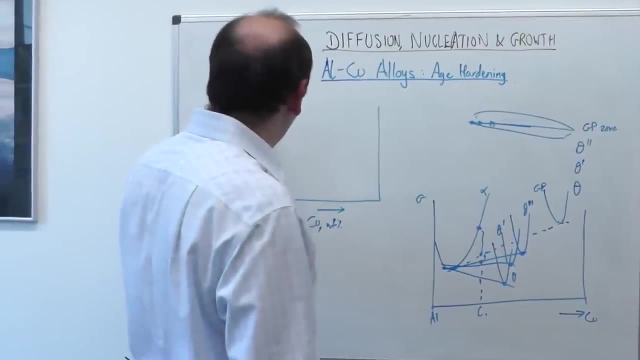 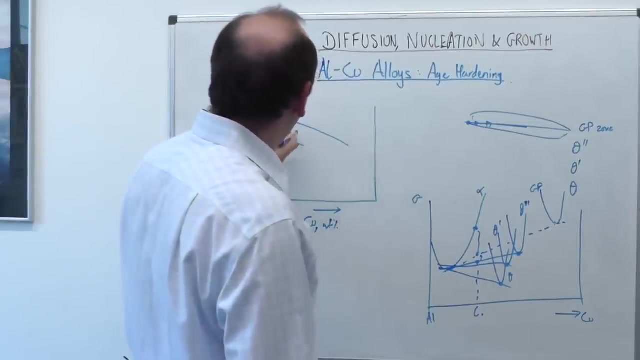 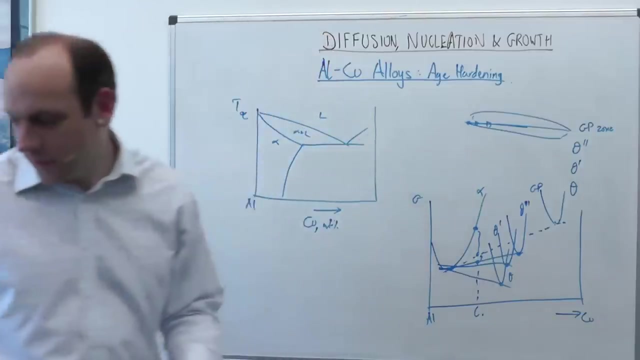 you like: uh, that's in degree c, um, and uh, the copper content, you. you go from something that's a bit like this: you go: you've got an alpha phase, uh, that's there, um, you've got an alpha plus liquid field liquid, alpha plus liquid, and your alpha phase is there. there's your eutactic, whatever it is, and this is the alpha plus theta. 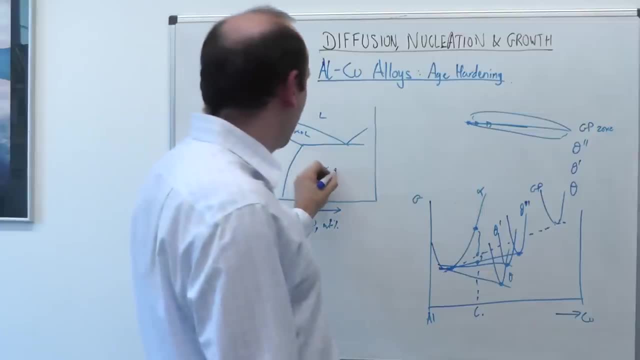 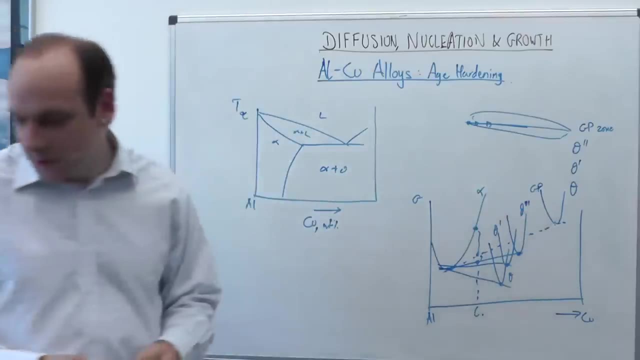 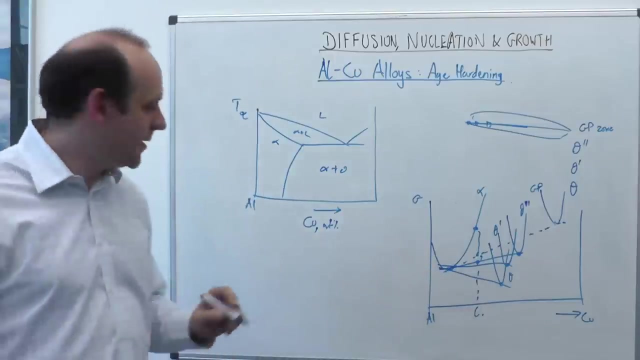 there's a theta precipitate over there somewhere on the diagram. so you have alpha plus theta um in the equilibrium phase diagram. but as you go through this sequence you get a gp zone which comes out initially at a larger composition with a greater amount of solubility in the alpha. so the 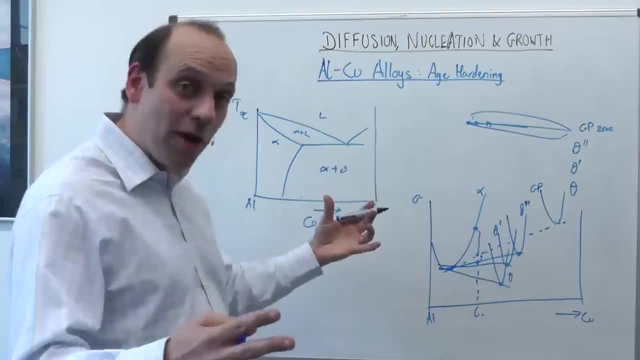 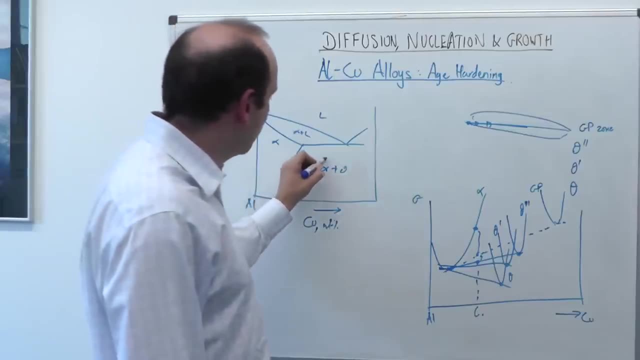 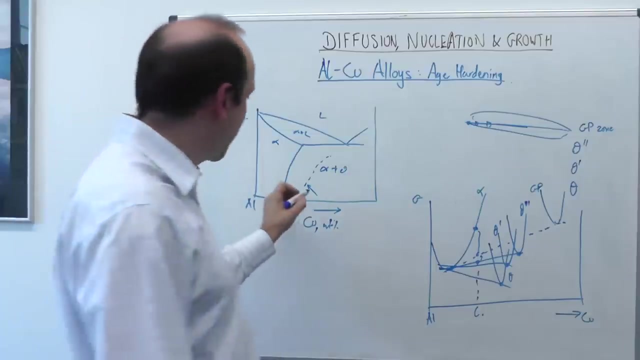 tie line. it's not a in the equilibrium diagram, but the tie line for the alpha gp zone would be somewhere slightly over here. we don't know precisely where it is, but it's somewhere slightly over there. so that's the uh tie line for the alpha associated with the gp zone and then the 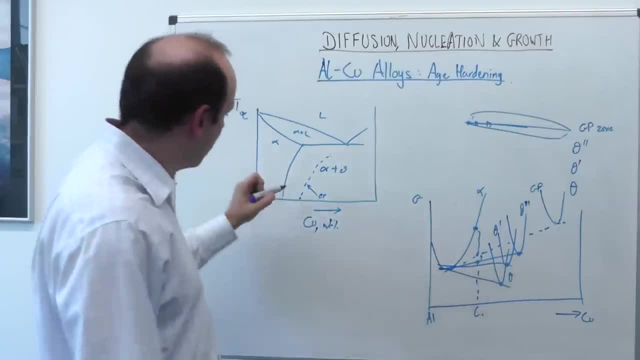 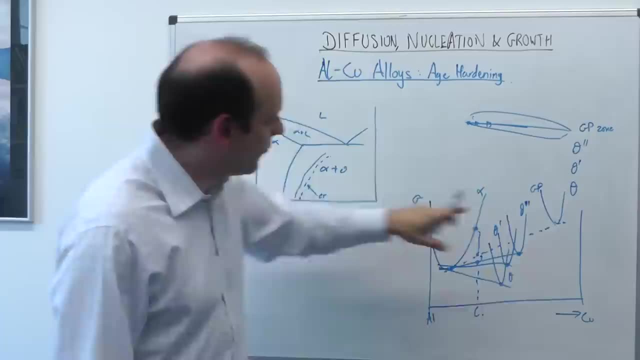 composition of the alpha when it's with the theta double prime. well, it's gone slightly purer. so with the theta double prime it does that um, uh. so that's the theta prime and that one's the double prime. i always forget the sequence. and then this one. 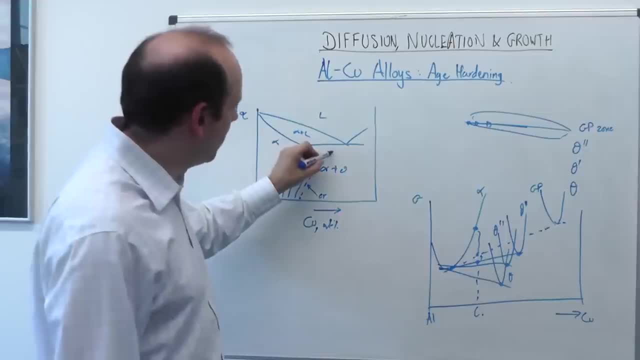 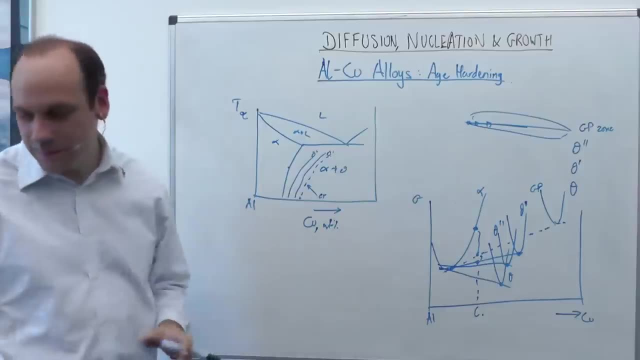 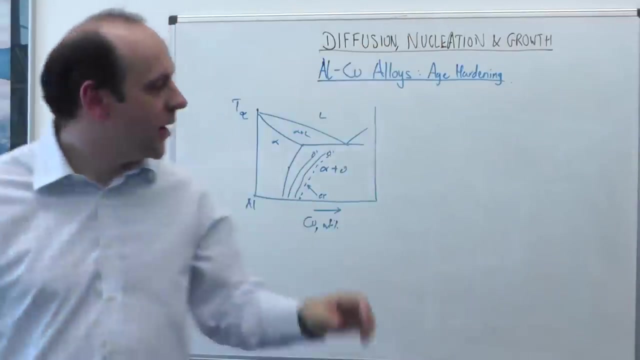 would be for your theta double prime. so that's your theta prime, theta double prime, and then this is your final alpha composition when you're forming with your theta phase um. so what that looks like. i'll put a micrograph up here of the theta prime phase in aluminium copper um and that micrograph shows that you've got little discs. 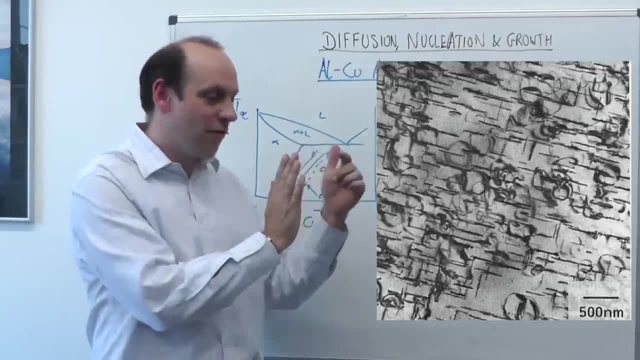 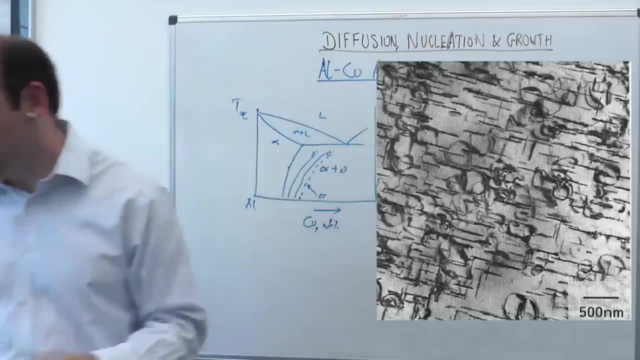 those little outlines. you see those little circles and you're viewing them either flat on or edge on um of those little discs. um, so you're viewing. it's like you're viewing a. um, if i find something disc shaped, uh, it's like you're viewing a disc. either that way or that way. 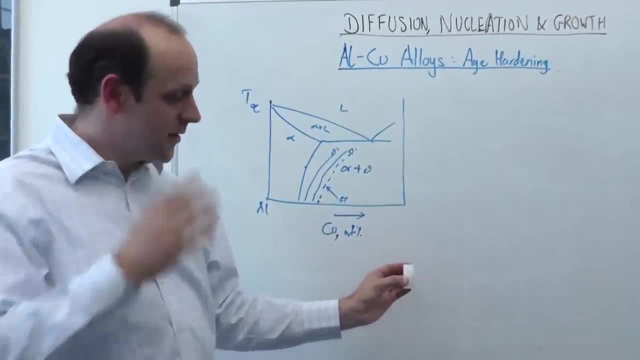 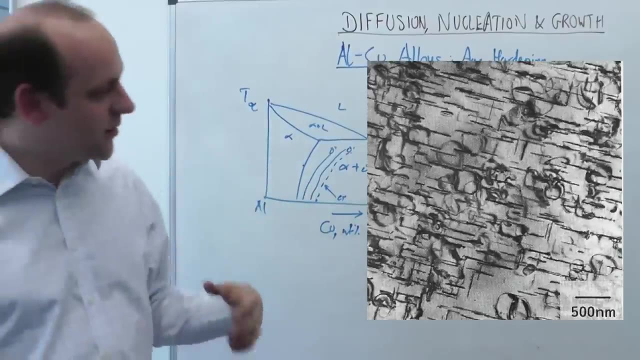 because there's an orientation relationship with the matrix that's being shown in this micrograph. so if you view the disc like that, you see a circle and if you view an edge on, you just see a line. and what you're seeing? there are circles and lines of the theta prime phase in an aluminium. 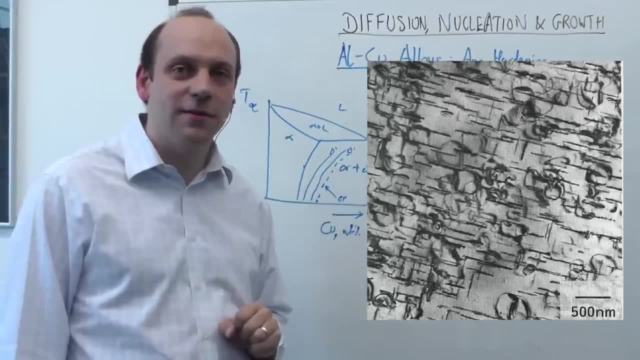 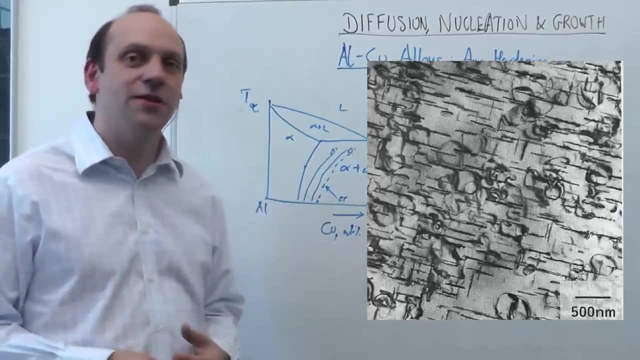 copper alloy that's been aged part way through this transformation sequence, and so that's a way in which aluminium can nucleate the final theta phase with a big surface. energy that requires quite large nuclei. and how did it get the nuclei? well, what happens is: first it's a big surface. 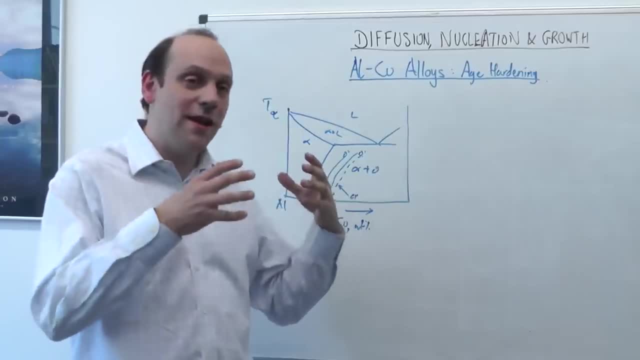 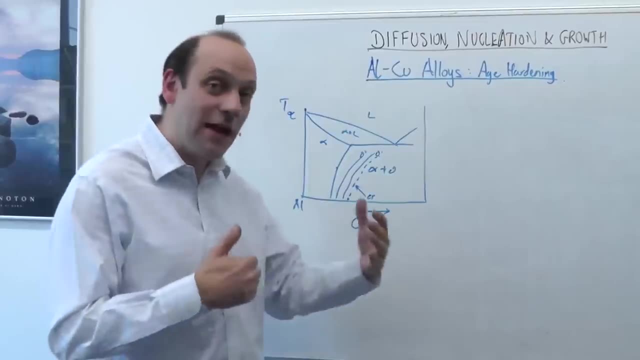 it forms some metastable phase, some phase that's not in the equilibrium phase diagram but is something that forms during the transformation sequence, that's easier to form but doesn't have as much surface energy, so it's so-called metastable um and that would be the gp zone and then the